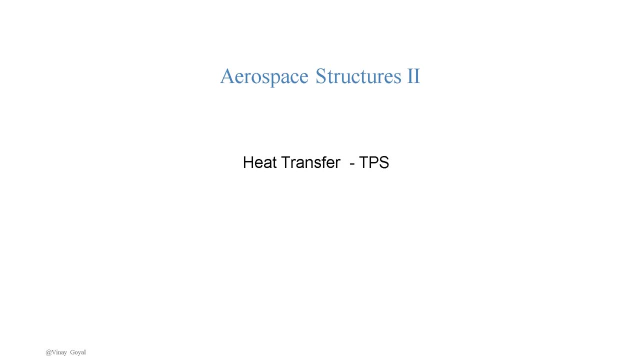 applications can work really well as well For launch vehicle applications or military spaceflight applications that have been regain their internal Hamilton applications. Heat transfer is also very important. You use insulation to protect the vehicle during ascent and you also need insulation in the nozzles or the various engine components or 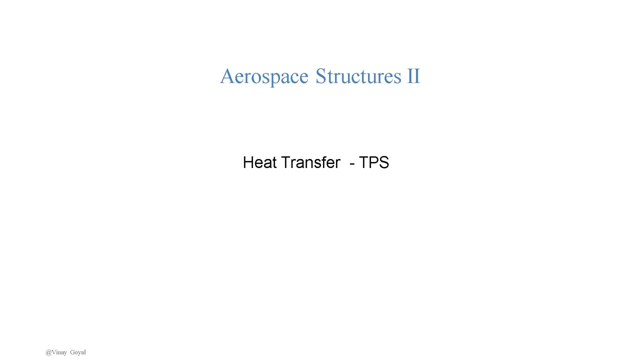 rocket components, You may also have to analyze a few heat transfer problems related to when you're filling up the tank and when you're heating up the tank and things like that. So those are very important to consider in the design of thermal protection systems, in the design of material. 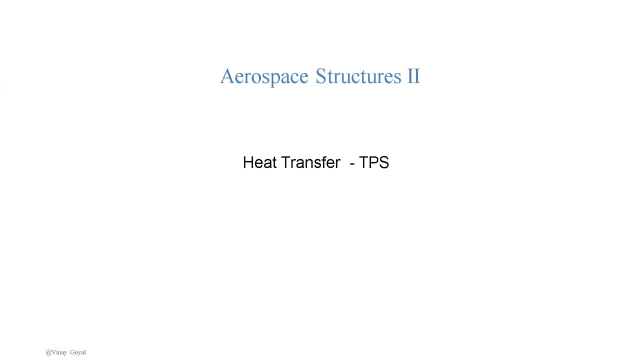 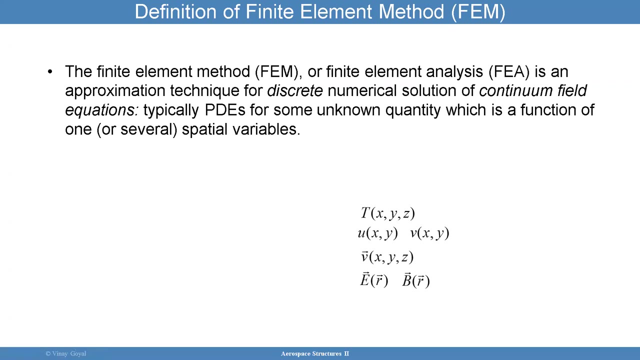 selection and also play a key role into the structural design process. So that's why we're making this a priority: to make sure we learn about the heat transfer, And while the finite elements is a very well-known technique, I want to just kind of open it up and kind of give a very 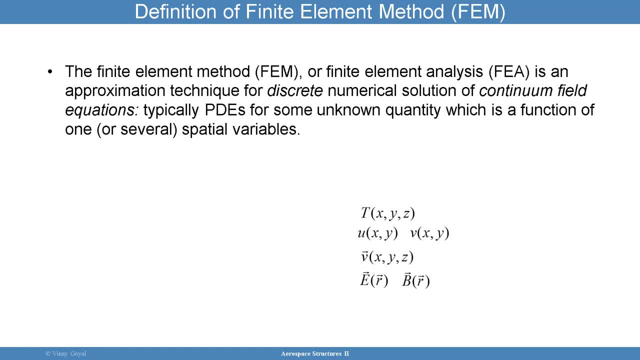 top-level view of what finite elements is really doing, because it is a true mathematical mirror. The finite element modeling or finite element analysis is an approximation technique that we can use and that's used to discrete numerical solutions. discretize numerical solutions of various problems And you can actually solve a lot of different problems, structural problems. 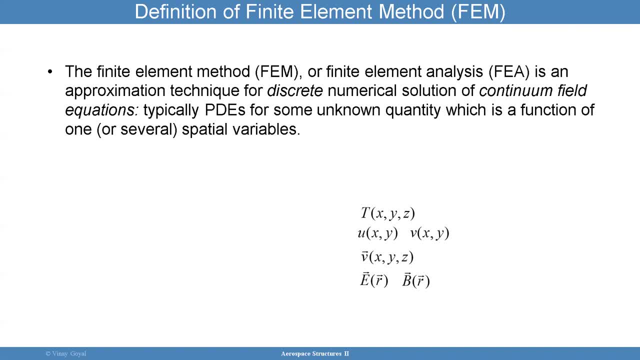 heat transfer problems, moisture diffusion problems and even find a fluid mechanic problem. So the idea is that when you have a partial differential equation which goes to the physics of the problem, that partial differential equation has to be solved for a particular variable of interest. So in a heat transfer problem the variable of interest is temperature. 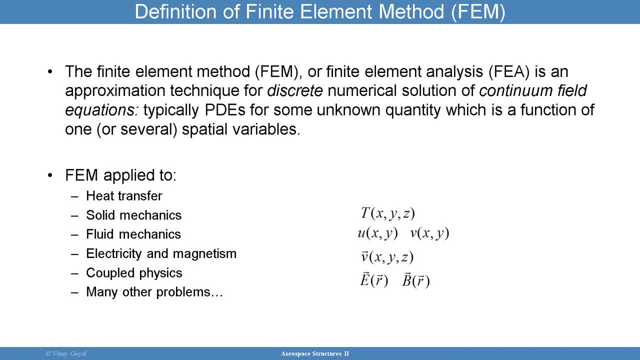 and that temperature can vary across in all three directions. Okay, so that's the variable we want to solve for. In solid mechanics, structural mechanics, we're trying to solve for deflections in all three directions, So that's the variable we want to solve for. So in that, 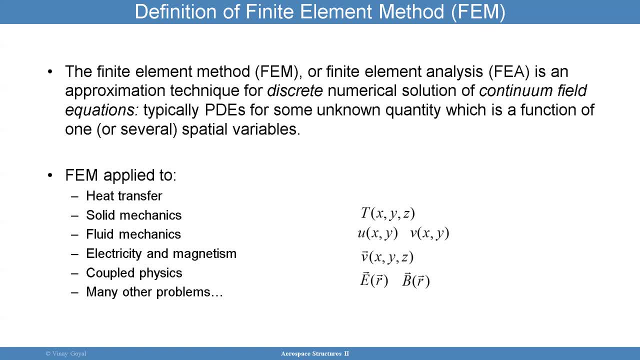 all the different directions. And once I know deflection, I can calculate strains. And once I know strains I can calculate stresses. And once I know stresses I can try to predict failure. And in reverse engineering I wanna make sure I design something so it doesn't break. 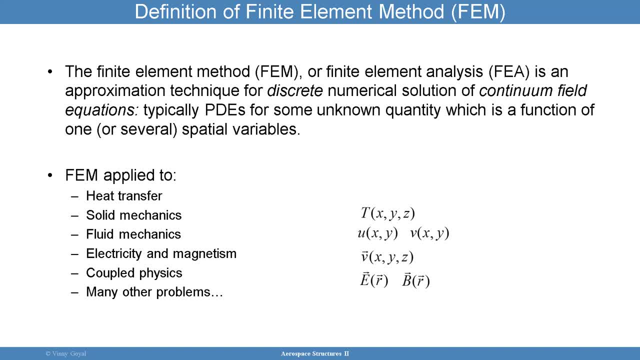 So you can then thicken the sample. You can do whatever you wanna do to make it work. Fluid mechanics: As fluid mechanics you're looking at velocity of the fluid. You also have electricity and magnetism, And then you have problems where you can couple heat transfer with solid mechanics. 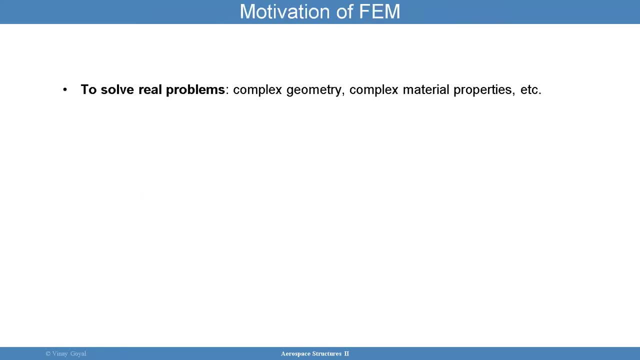 or couple a few of these things together. So what is the motivation behind finite elements? I think the idea here is to solve real problems, because without finite elements you are kind of stuck with hand calculations. Now, we're not against hand calculations by any means. 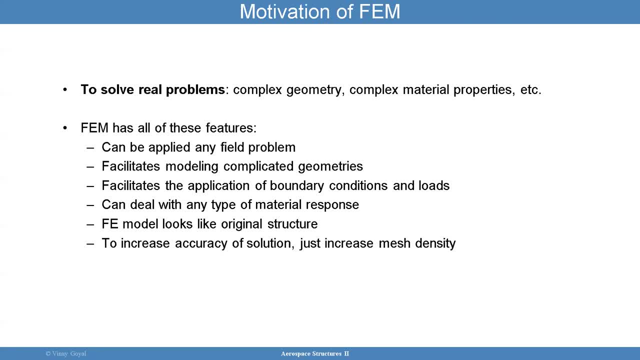 but it is very powerful to be able to solve problems involving a high amount of complexity like an aircraft. An aircraft is highly complex to solve by hand, But if we can do some work with finite elements to simplify the modeling, so I can get somewhere with it. 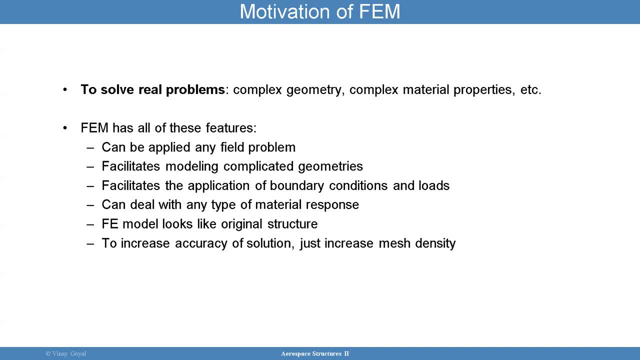 why not? And so the finite element has a feature that no other code really has. It can be applied to any field problem. It can facilitate modeling complicated geometries, It can facilitate the application of boundary conditions and loads and can deal with any type of material response. 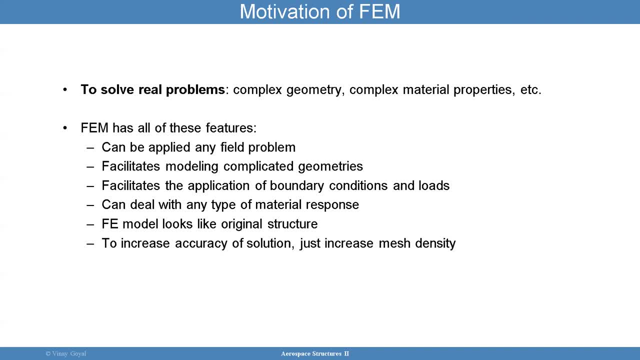 The final model. the good news: it looks like the original structure, And that's a cool thing. You can look at it in a computer To increase accuracy of the solution. the cool thing is that all you have to do is to increase the mesh density. 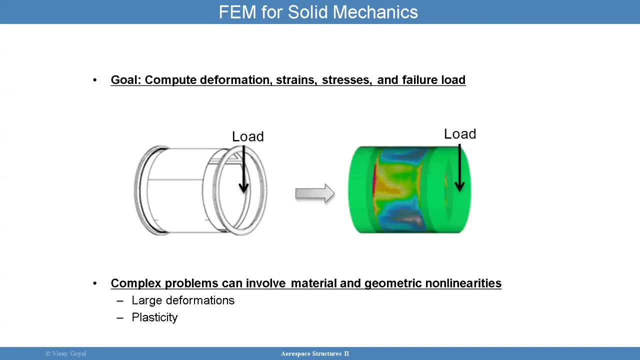 And I'll explain a little bit later what I mean with mesh density. So what is the goal? The goal in this particular example for solid mechanics is to compute the deformations, the strains and stresses and the failure load. That is one objective. 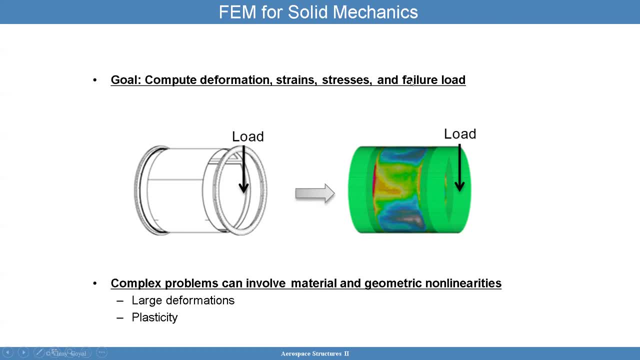 or if you know what the failure load is going to be, with limits of the structure of the loads. you can then design it so that it doesn't fail at that particular load it needs to survive. The complex problems can really involve material and geometric non-linearities. 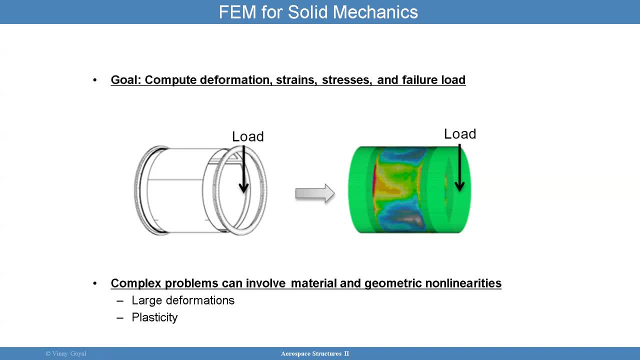 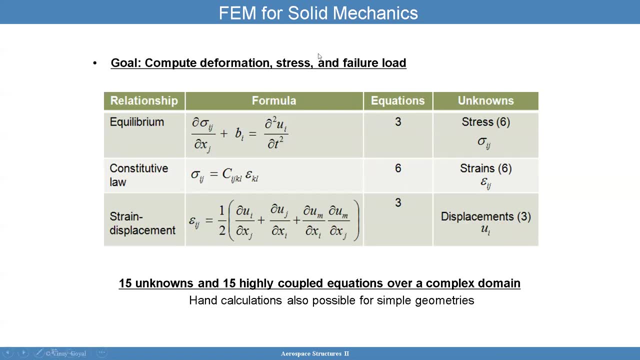 We're going to see that later on in this course, large deformations and plasticity will both be discussed. We need to compute deformation, stress and failure load. So here's an example of the partial differential equations that need to be solved, And there's a error here. this should be six, six equations. 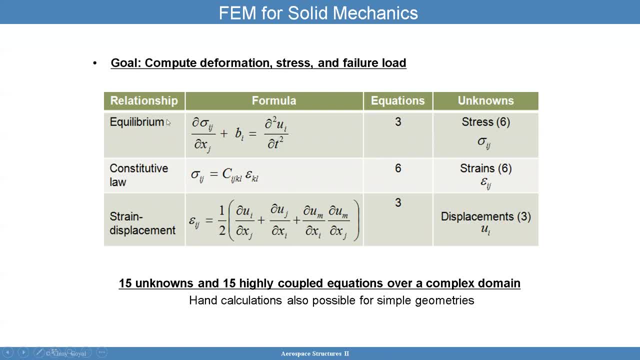 So we have 15 equations that are highly coupled. In the first equation set we have equilibrium equations. In the second set we have the constitutive law that relays the stress of the strain, And then we have the strain deflection relationships. 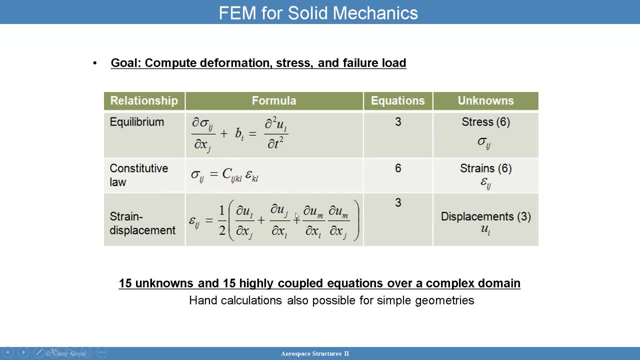 where the strain relates to these deflections: U1, U2 and U3.. So how many equations I have here? I have three. here I have six, here I have six. I have a total of 15.. And how many unknowns I have? I have 15.. 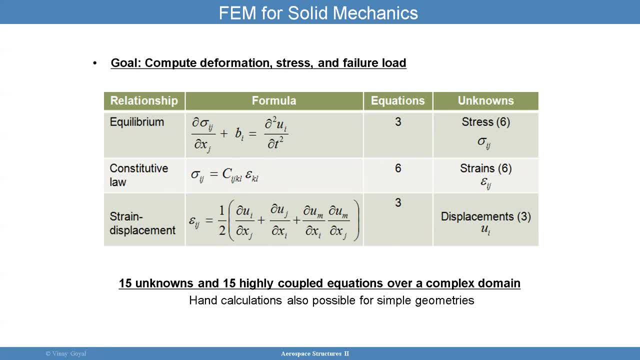 And so how do I solve 15 equations and 15 unknowns? They're highly coupled and they're also need to be solved over a complex domain. If you recall when you took differential equations in school, that was quite complicated for a simple problem. 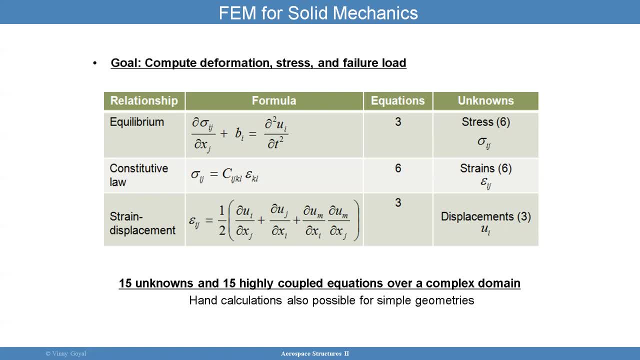 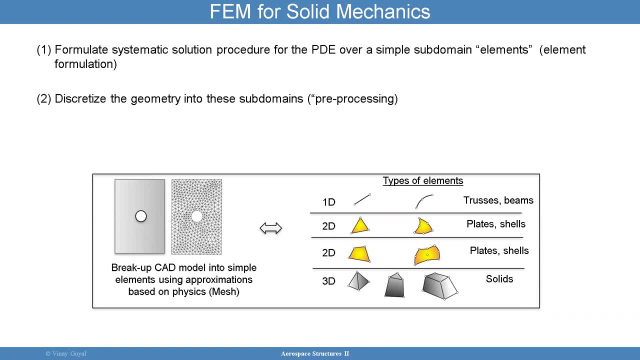 in a one dimensional domain. Just imagine trying to solve this in 3D and it's partial differential equations and it's 15 equations, 15 unknowns. So what is the idea of finite elements? You know, the goal of this course is not to teach. 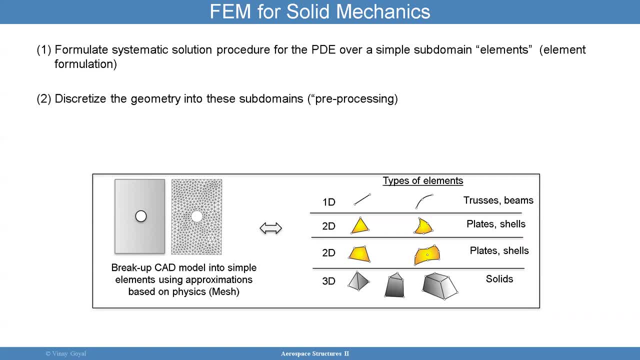 the fundamentals of finite elements. That's taught in a different course And I have a number of video lectures you can watch if you're interested in that, Or you can take a finite element course at your university. But right now what I'm trying to do 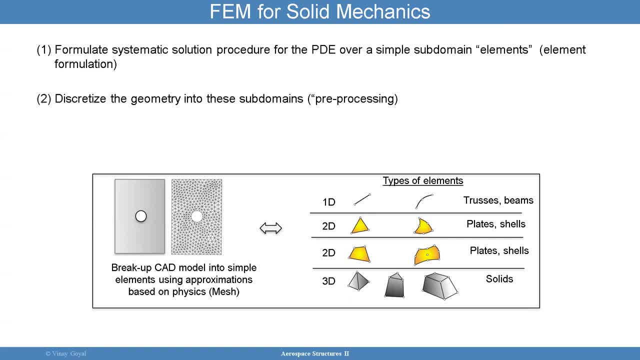 since finite elements will be a big part of what we're gonna be teaching here or using in the applications, because this class is an applied class. We're gonna be applying some advanced concepts in finite elements to real, real world applications, And so that's why it's for me important. 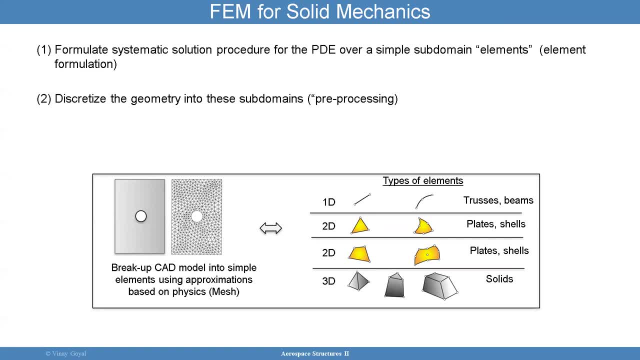 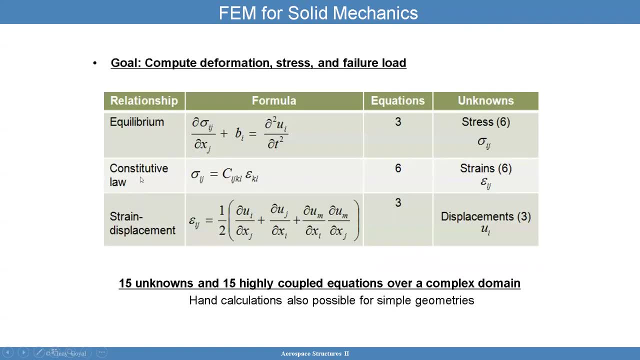 that if you have not taken a finite element class, you at least understand the conceptual ideas behind them. So if you look at this CAD model on the left hand side, I wanna solve this- partial differential equations that are highly complex. they're highly coupled. for these 15 unknowns. 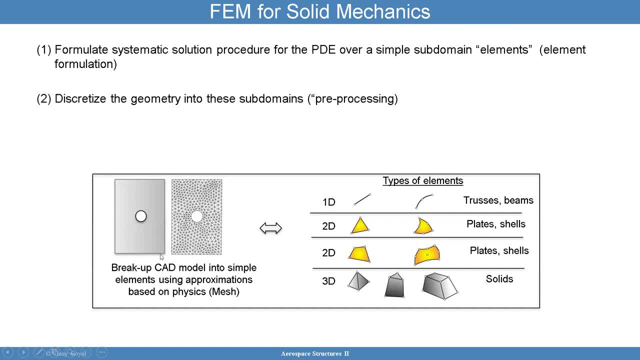 Well, what I'm gonna do is something very simple: I'm gonna take this domain and I'm gonna divide it into subdomains- small subdomains, very small subdomains. And what I'm gonna do is I'm gonna divide it into subdomains- small subdomains, very small subdomains. 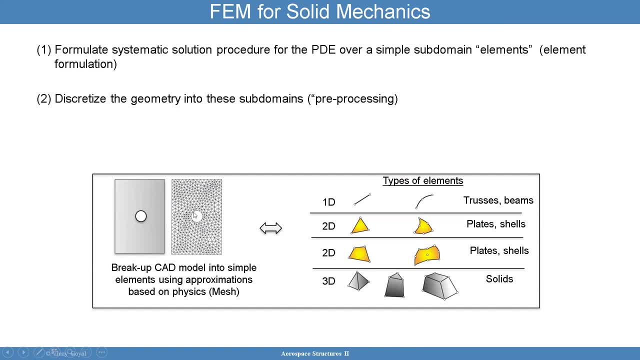 And what I'm gonna do is I'm gonna divide it into subdomains- very small subdomains, very small subdomains. And where it matters the most, let's say I'm interested in what's going on at the hole, then I'll increase the number of subdomains. 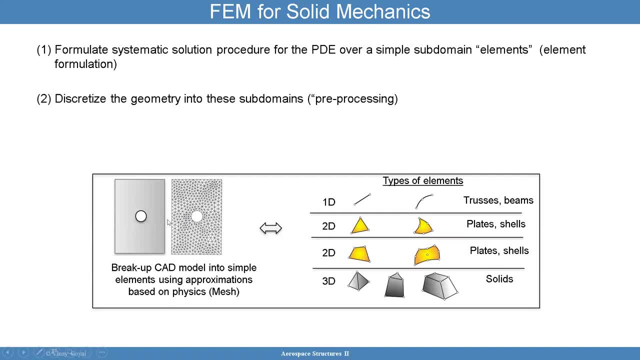 And you can see very clearly. I divided a subdomain into triangles. I could have used quadrilaterals, for example, I could have done that, but in this case I'm showing you a triangle. Well, I'm breaking up that CAD model into simple subdomains. 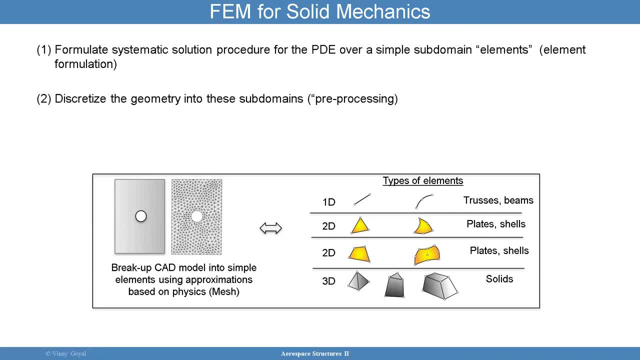 which I'm gonna call those subdomains elements. So when I say I have an element, an element, what I'm really talking about is these little subdomains And these subdomains. the cool news is that I can have various element types. 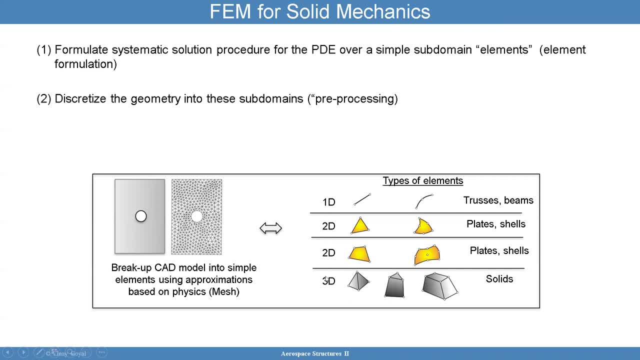 So finite elements basically is based on using subdomains that have shapes that can be used for breaking up the structure. So in 2D I could have used this one or this triangle to break it up, Or I could have used even a more advanced element. 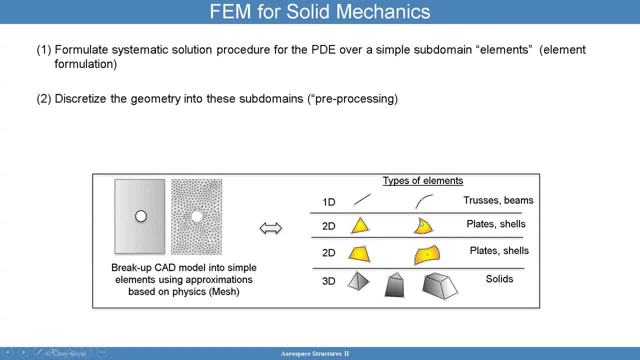 which has mid nodes and allows me to model with more accuracy. maybe this sharp, this, this circular hole, we can then put this triangle around that, for example, so we can get more accuracy. But it's more computation expensive. So you have to kind of trade which one is best for you. 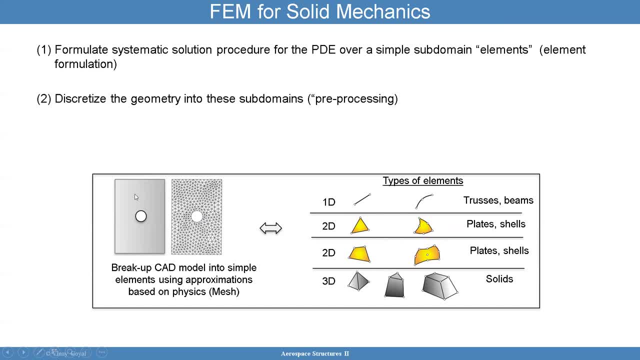 The point I wanna make is, all I'm trying to say is that this CAD model is broken up. It's broken into small elements, And those small, those elements that you see here. the beauty of this is that this, every single element here, has different shape. 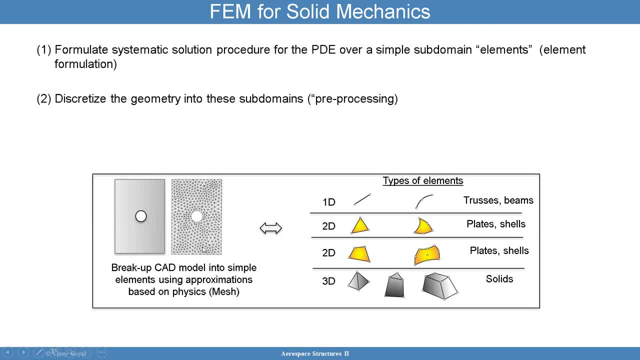 and it's not the same. However, there is a way in finite elements, to take every element and map it into a standard element, And that element, basically, is where you do all the calculations. The cool news is that you can take these 15 equations. 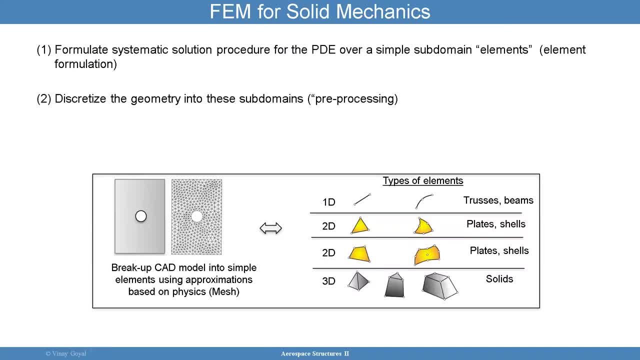 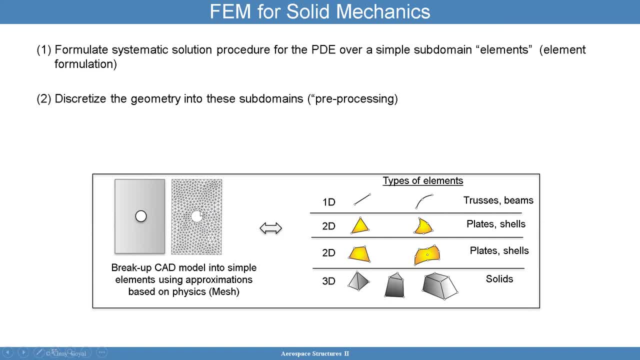 because every single triangle here is not the same as that standard element. I can also do that with quadrilaterals. This quadrilateral here has a very random shape, And if I were to discretize this domain with quadrilaterals, every quadrilateral will look different. 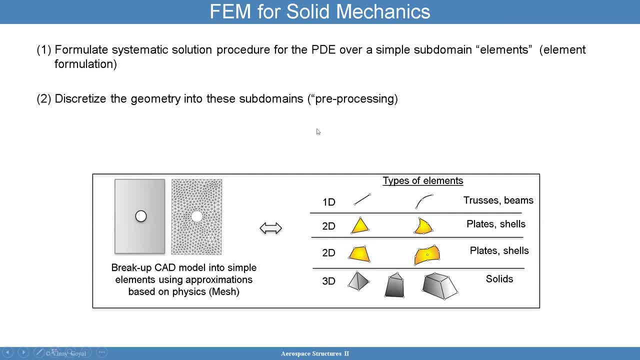 But if I map it, I could map it into a square, which is incredible, And that square is what I will be using to solve these 15 equations, 15 unknowns, And so that's the good news is that I can break with finite elements. 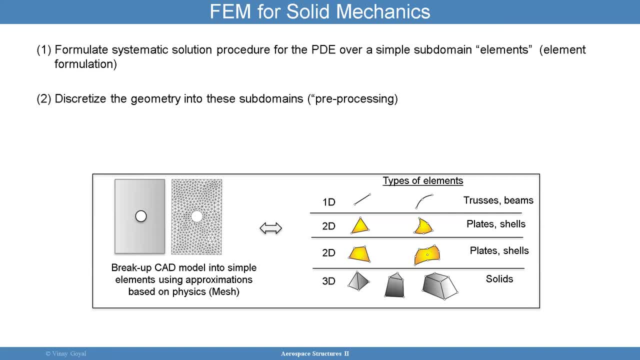 I can divide the domain into small pieces And those small pieces can be turned into standard elements. that applies to every single element in the domain And, using something called mapping, we're gonna map a triangle to a standard triangle And by mapping the geometry to a standard domain. 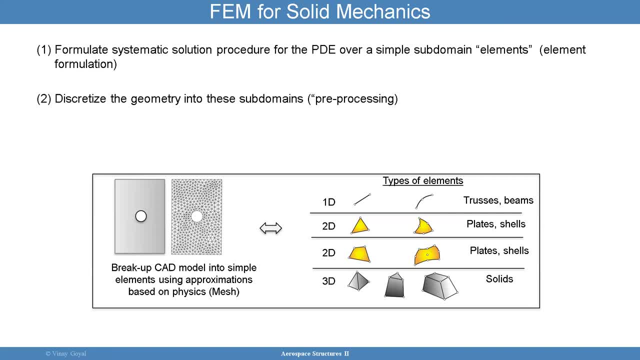 what I've done. I've simplified the problem And I'm now able to solve these differential equations by connecting them back together. You can see, I can solve every triangle by itself, but then I have to piece it back together And the locations at which the two triangles meet. 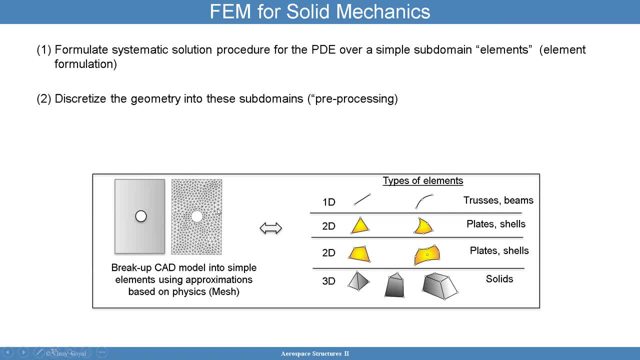 you can see there a vertex. we call that a node- Locations where elements meet with each other. So, for example, this triangular element has nodes, has three nodes: One, two and three at each vertex. So this element will be adjacent elements. 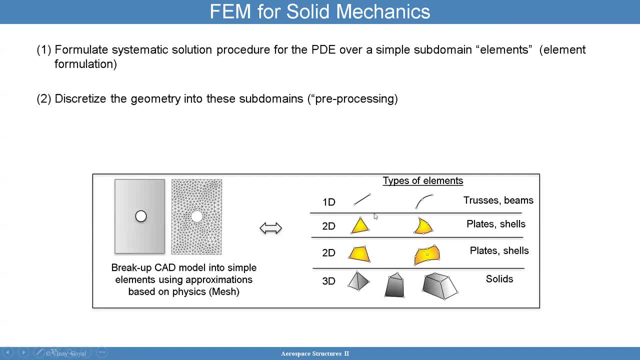 will be connected through these two nodes. So I'm gonna have a triangular element right here And then for this here. you can see here it's highly curved. Well, I may have another element that's next to it, And these nodes are shared. 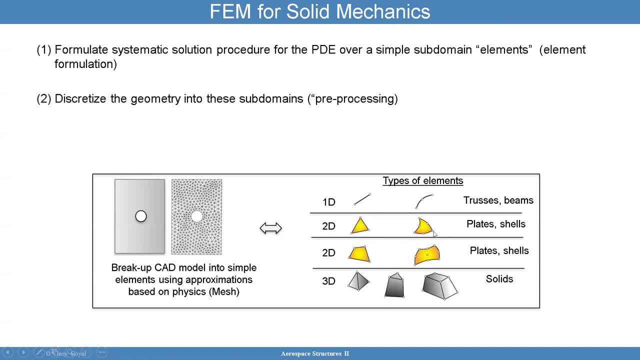 these three nodes are shared along that edge. Okay, so that's kind of what we're talking about here. So I wanna make sure it's clear that this triangular element is of lower accuracy than this triangle element here with mid nodes, And the reason is because you have more degrees of freedom. 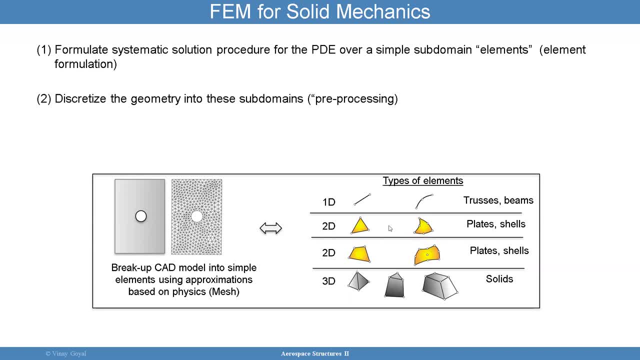 So the polynomial, because this, the solution of partial differential equations- really accomplished by assuming a polynomial distribution that's able to basically approximate the solution to the triangle, And the same thing goes for this one here. So the triangle here on the right-hand side has more nodes. 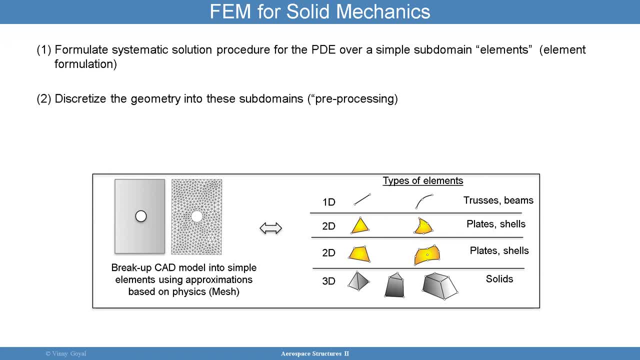 So you're gonna have a higher order polynomial that's going to be better at capturing the response of that triangle And in addition to that, square elements have more terms. I have four nodes, so I have four terms in the polynomial approximation compared to 2D. 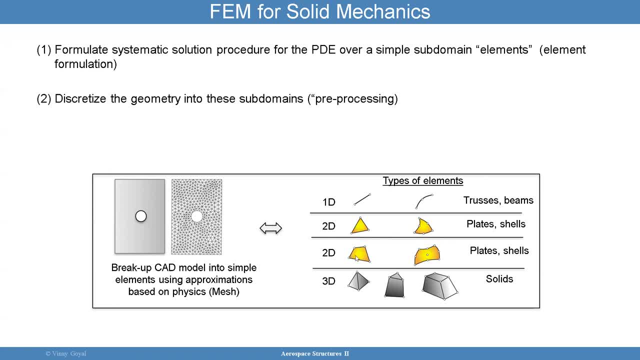 2D has only three, So I'll expect a 2D element to be a little bit more accurate than a triangular element, And when I go to mid side nodes I have even more degrees of freedom, So therefore I'll expect even more accuracy. 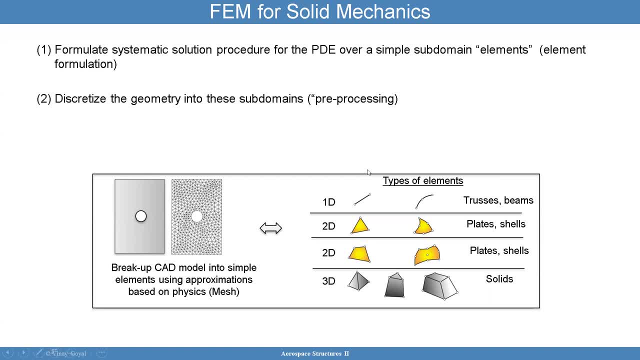 but that's not always the case And you have to do kind of the study to figure stuff out. So this process of taking a CAD model and converting that into subdomains as you see them here, we call that the pre-processing stage. 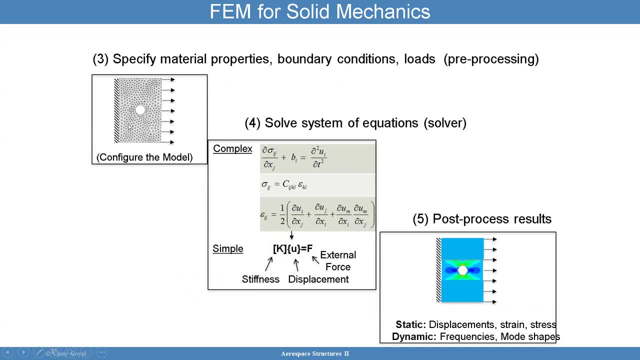 And then I have to configure the model. What do I mean that with that? That's also pre-processing, by the way. I'm gonna apply the loads at these nodes. I'm going to apply boundary conditions. So say, it's clamped at the very left end. 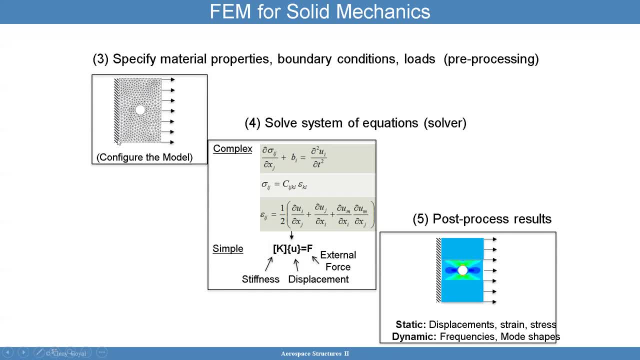 I'll take those nodes and fix them And I will apply material properties. I'm gonna say, okay, this is steel or aluminum. I have to tell the software what this material is And I'll specify to the software what those properties are. 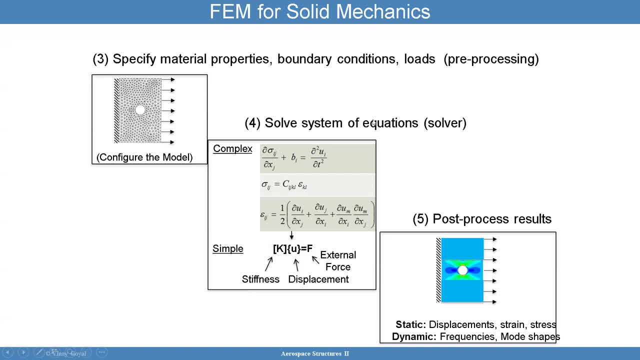 And then this is where the magic happens. We solve the system of equations, And this is an insane part of finite elements. I'm taking a very complex problem with 15 equations of 15 nodes and I'm taking that and simplifying that. 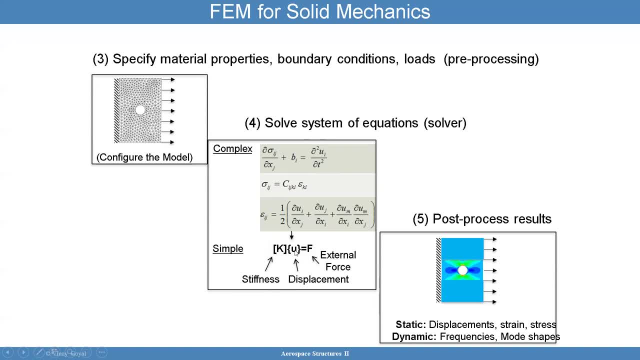 into a stiffness matrix. times the depletion equals external force And these are very simple thing to solve for And what this is gonna give me is the deflections at every node. you see here Beautifully done, because now I can take that and plot that directly. 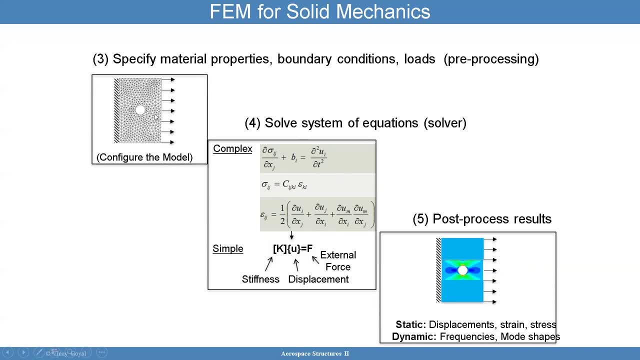 So I took a highly complex fix, complex partial differential equation for a very complex job. it's actually complex, not easy to solve, not complicated for a domain that's not easy and i'm solving them and that is going to lead to simplification, which is a linear algebra problem. ku equals f. all i have to do is invert the stiffness. 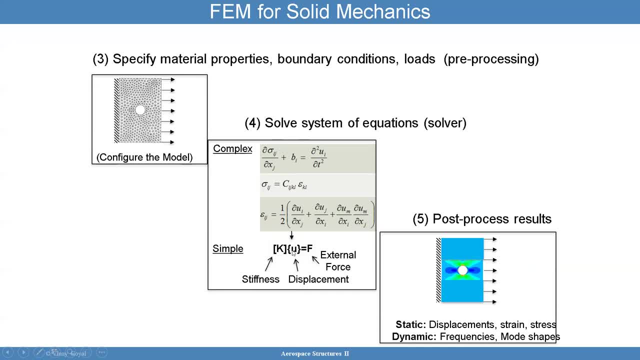 matrix and i can solve for the deflations. one enough. once i know the deflections, i can solve for strains. once i know for strains, i know strains, i can solve for stresses. we can do this and now that i know the deflections, i can plot the deflections, i can plot, the strains, i can plot. 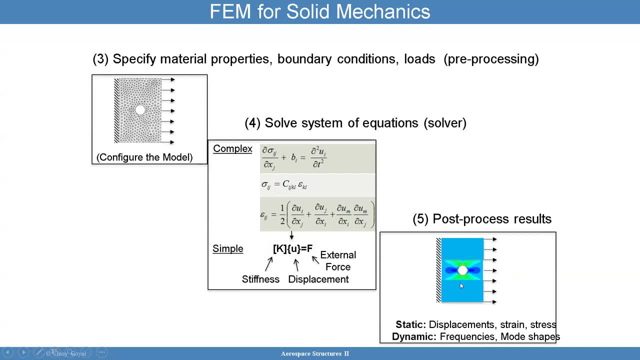 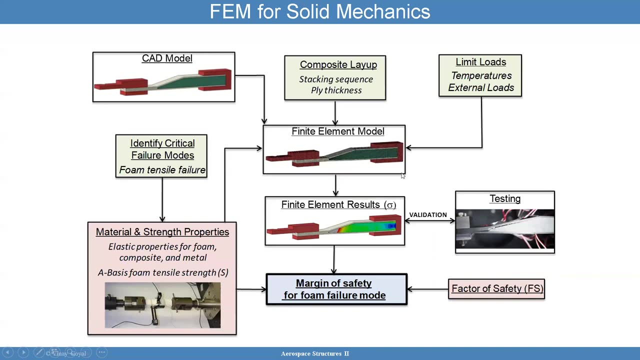 the stresses. what's plotted here is the stresses. for example, i can do dynamic modeling as well. we'll be doing a lot in this course. we're going to be doing steady state dynamics, random vibration and so so the idea of finite elements is quite powerful because i can solve problems i couldn't. 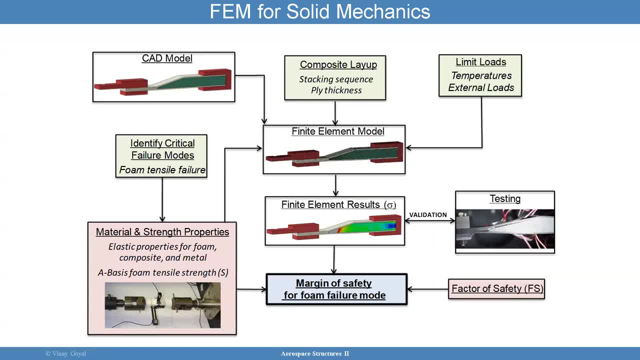 do before, so in finite elements for solid mechanics. what are the different aspects that come together in the big picture perspective? you're trying to make sure that you have a sufficient margin of safety for the system, and so that implies that you have the cad model that you're giving the composite. 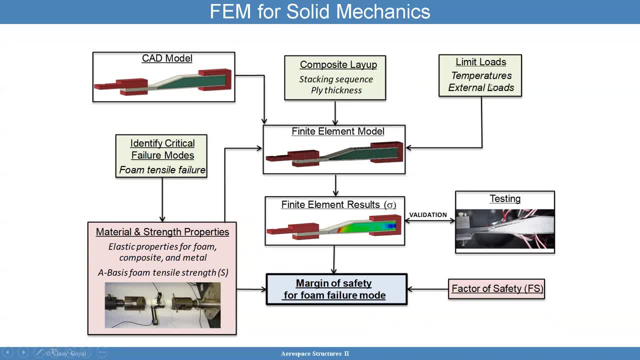 layup, the stacking sequence. you're giving the limit loads, the temperatures, external loads, all the stuff you need, that you have identified all the critical failure modes and then you have measured all the properties for all the different constituents: the composite, the foam, the metal, everything you need that goes as an input into your finite element. 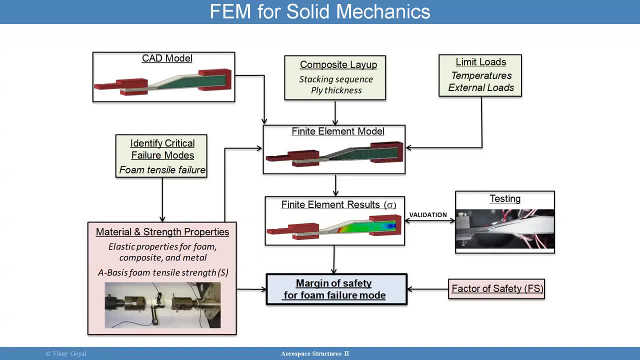 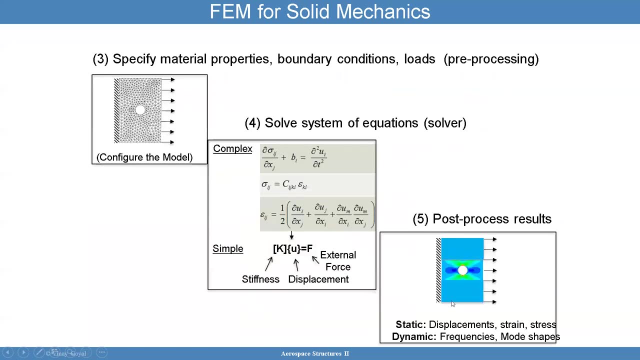 model, all the elastic properties, the modulus, the young modulus, the Poisson ratio, the composite layup, the geometry, the limit loads. you mesh it and here you can see that as a divided sub domain, using this solid elements here on the very bottom right, 3d, solid hex elements, we call them, has eight nodes. 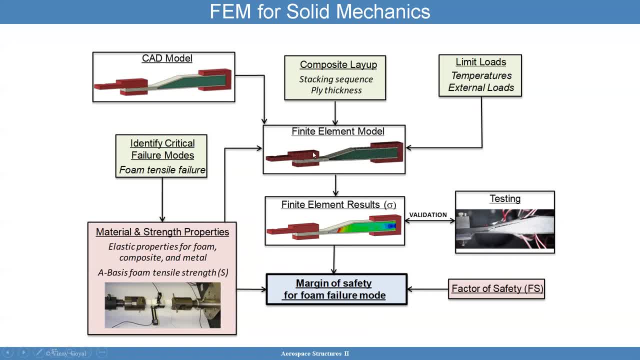 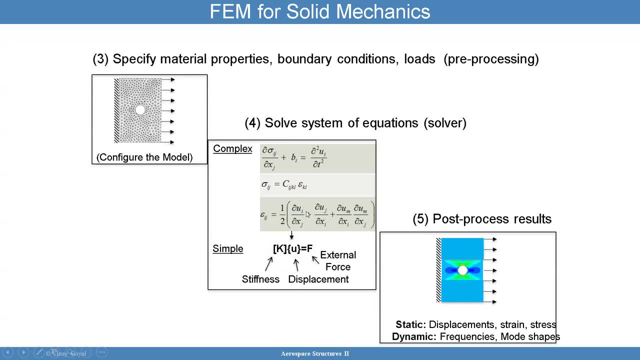 and so it's very nicely meshed, and then that is then the. what we're going to do now is solve this 15 equation, 15 unknowns, by approximating the subdomains into polynomial using polynomials, and that what allows me to do is allows me to. 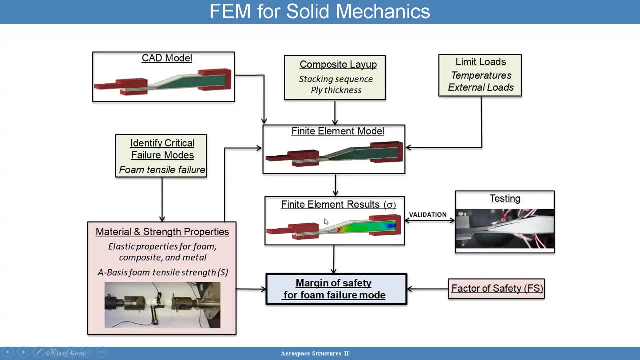 simplify the problem to: ku equals f, which allows me to then plot the stresses very easily. and then i can now validate my model to make sure it matches the test. if it doesn't match the test, i have to make adjustments to my model to see what i got wrong. 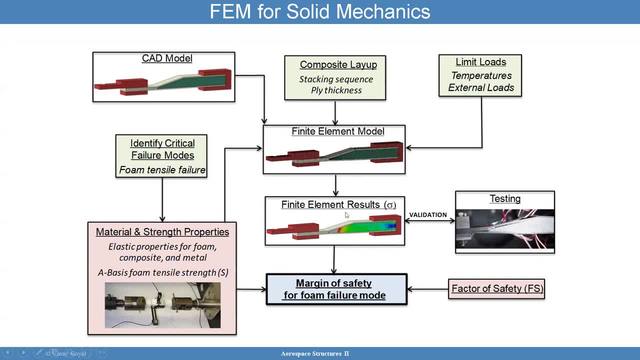 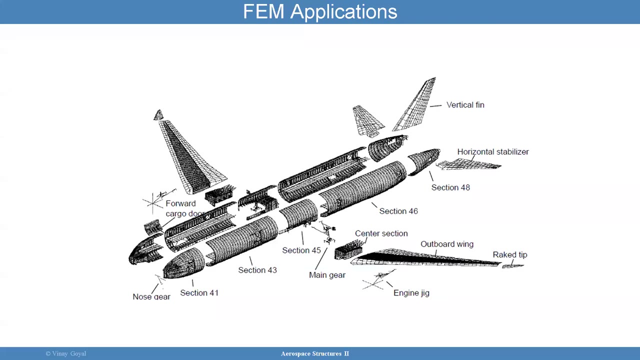 because analysis does become important. is the analysis what provides the transfer function between a test on the ground and something that's flying? and now i can use the finite element results to provide the margins- margins of safety for the system, if you know the factors of safety for the given program. when you look at more advanced applications of final elements, as 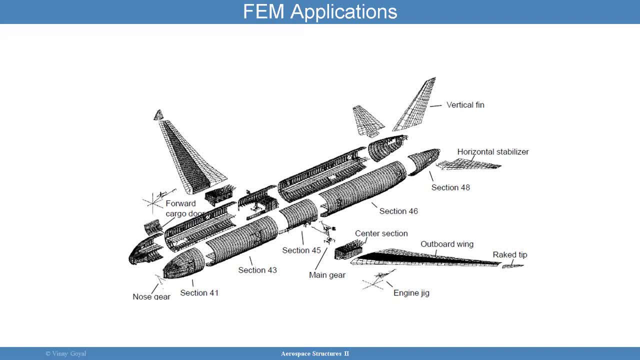 applied to airplanes, for example. um, you're going to have to really be smart about how those are applied and typically in a large company that's working on an aircraft, you could have various components of the aircraft being provided to the various um various peoples within an uh on our organization, so you could have person a works on the wing. 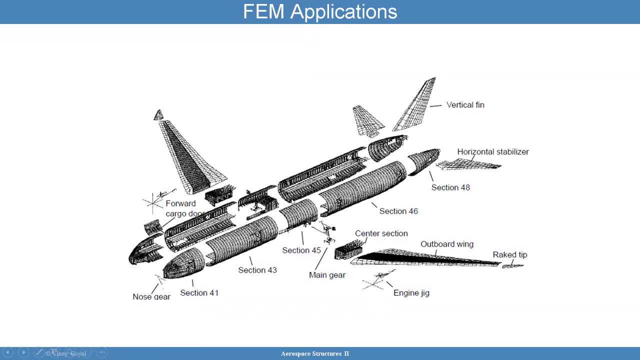 person b works on the tail and what you want to do is have a way of connecting everything together. so there is some amount of coordination to make sure that the mouse can be assembled into one big model Because, as I will discuss later, dynamics becomes very important. 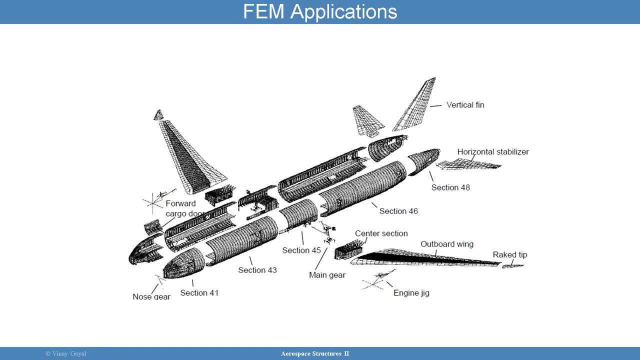 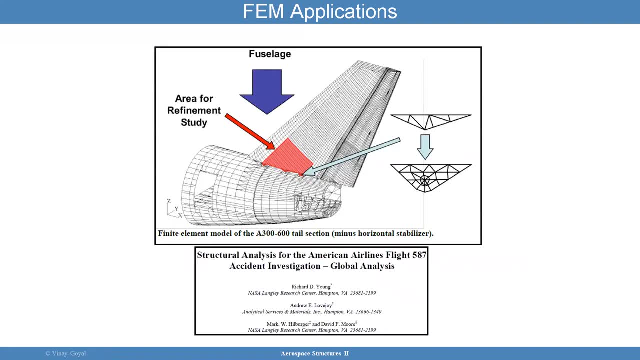 We're gonna derive loads based on dynamics and then apply those loads into static models to gain more confidence in what we're doing. Final, eminent applications have been used quite significantly. For example, you have the American Airlines flight 587, accident investigation where the tail broke off. 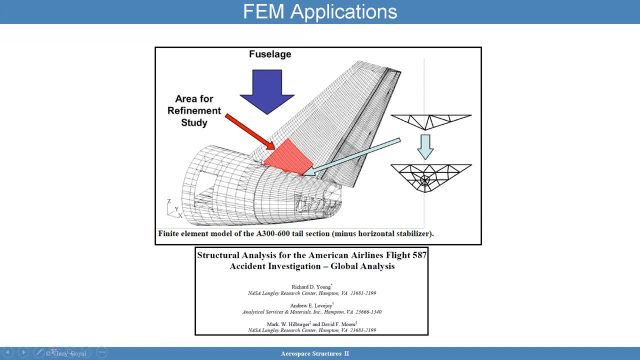 and the aircraft crashed. That's an example of where you could then study the area of concern by refining the mesh. And when I say refine the mesh, it's to increase the number of subdomains, make it smaller, make the elements smaller and increase the density of them. 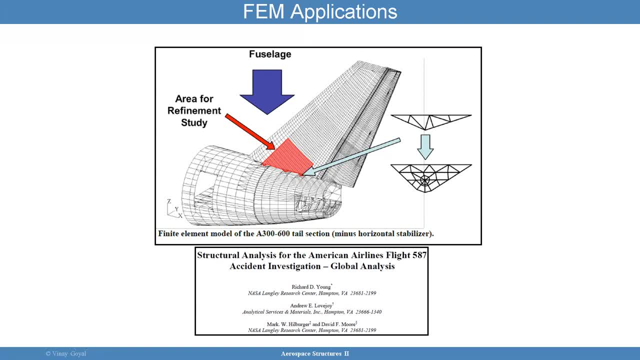 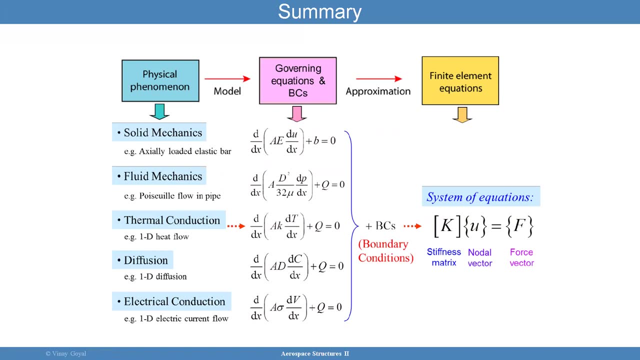 to increase our understanding of system performance in that location. So, in general, you have a physical phenomena- and I hear what I've discussed with solid mechanics, but you have a physical phenomena, solid mechanics, fluid mechanics, thermal conduction, diffusion, electrical conduction. 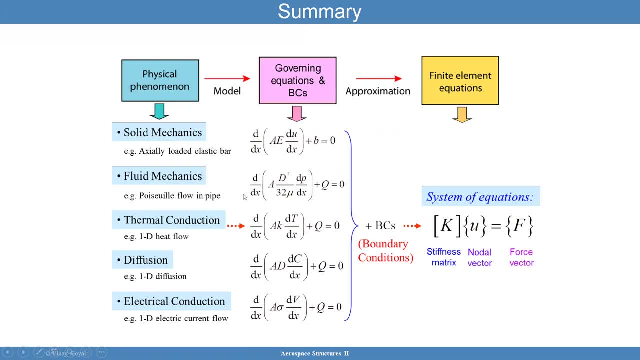 And then I have a set of governing questions for each of these guys that describe that physical phenomenon. That's your mathematical aspects, right? But my goal, then, is to use polynomial approximations to then be able to turn these governing equations, which are a pain to solve by hand. 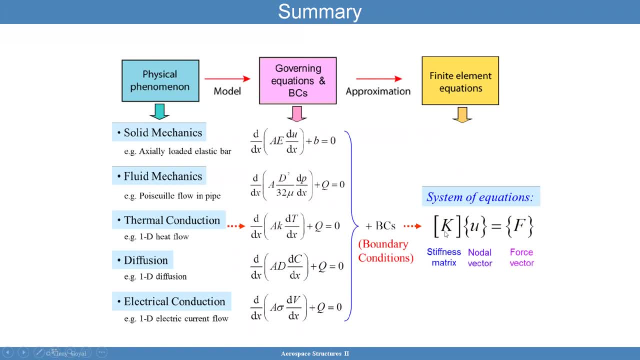 and turn them into linear system of equations and can be nonlinear as well, but generally linear, linear for 90% of the problem. And you have the stiffness matrix times the nodal vector, times the force vector. I can solve for this value here And U here could represent in this case could be: 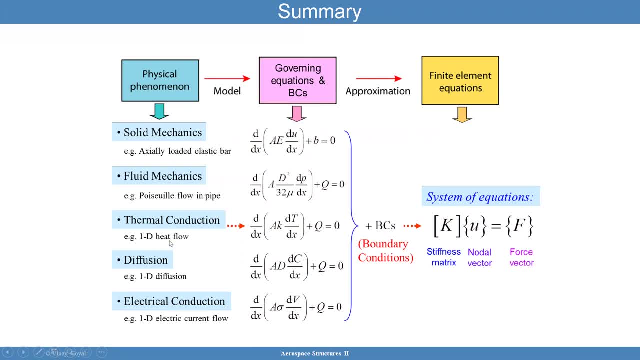 the deflection, In this case could mean the flow velocity, In this case could be the temperature, In this case could be the moisture concentration, In this case could be the voltage. So you can solve for those variables, for the variable of interest. Now here is an example of a 2D. 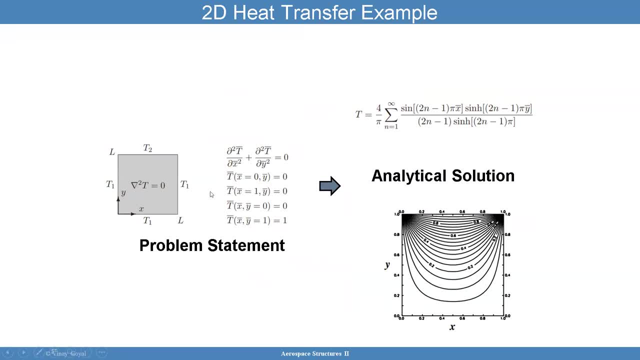 heat transfer problem And you can actually look it up. the solution to this Very interesting If I have this square and look at how simple the problem is. by the way, Look at how simple the problem is. Say that the temperature on this edge is 100, and on this edge is 100,. 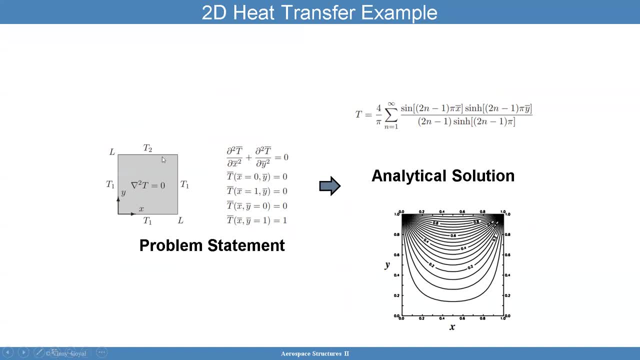 and on this edge is 100, and on this edge is 400.. Well, the solution is actually not that simple And the analytical solution looks like the one at the top right Now. I tried to do that for like an aircraft or a spacecraft which has hundreds of components. 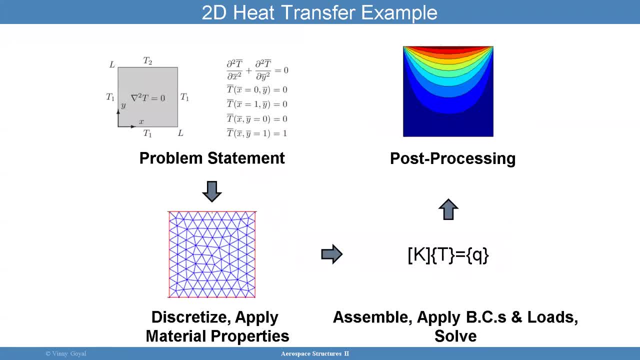 That's not tractable. We don't want to do that. We want to figure out a way of taking that partial differential equation which you see at the top left, which is the Laplacian- It's Laplacian of the problem, And I want to take that, take this domain, which is actually 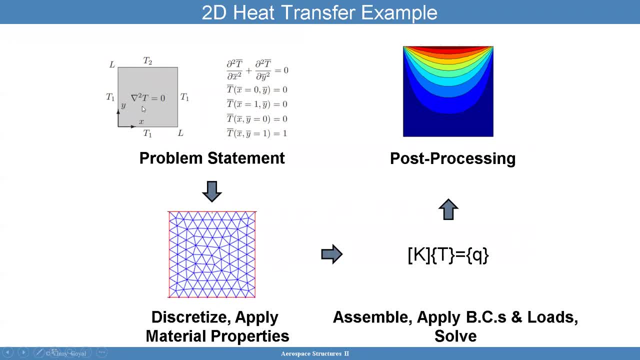 simple. actually, You will think that it's easy to solve, But clearly it takes a very complex analytical solution. I'll take this domain, divide it into subdomains, triangles, and then I'll take that and turn it into kt equals q. k is known, q is known, k depends on the. 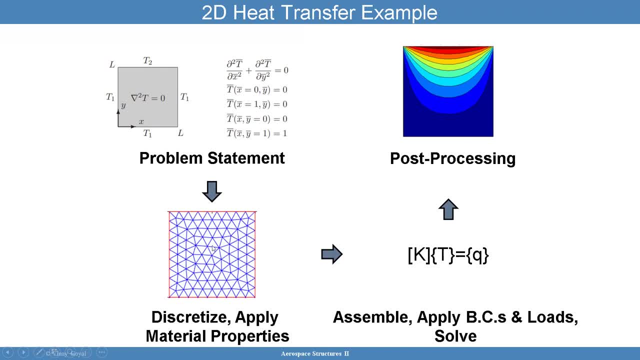 geometry Depends on how many elements I have, It depends on the material properties and so forth. q are the heat fluxes I'm applying or the temperatures I'm applying, But I can solve for t now and when. I solve for t. 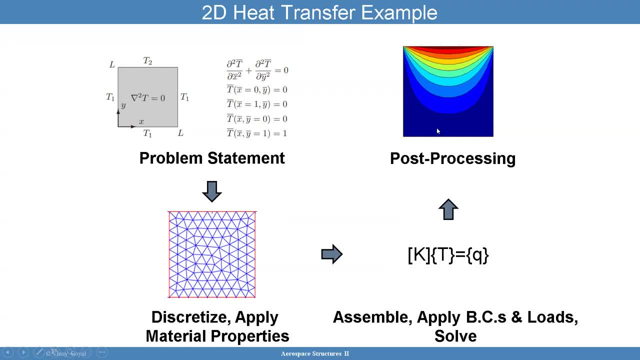 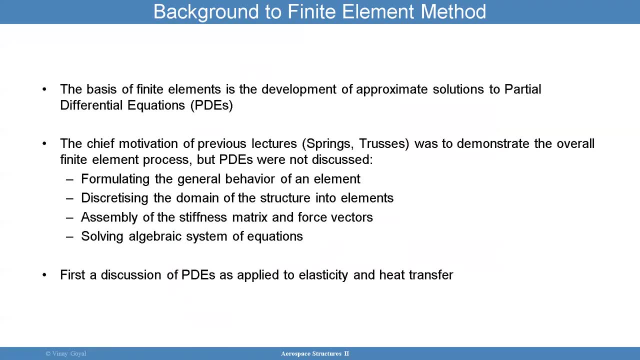 I can just plot it. That's the beauty of finite elements. All I have to do is mesh, apply the properties correctly, plot the results, which is extremely powerful, And it allows us to study problems that will have been otherwise very difficult to study. So the basis of finite elements is really the 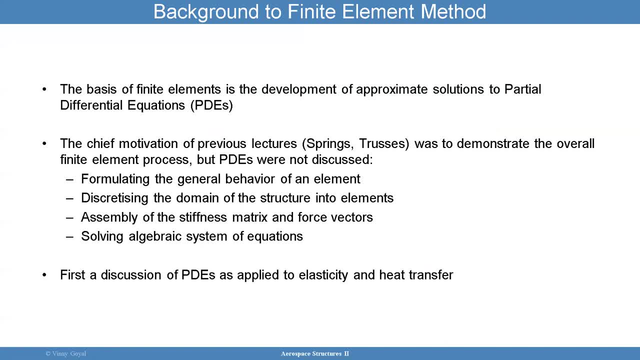 development of approximate solutions to partial differential equations. in summary, And the chief motivation of lectures that you may have seen in finite elements is to study the problem of finite elements, is to really show how to put everything together. So we're going to really look at the 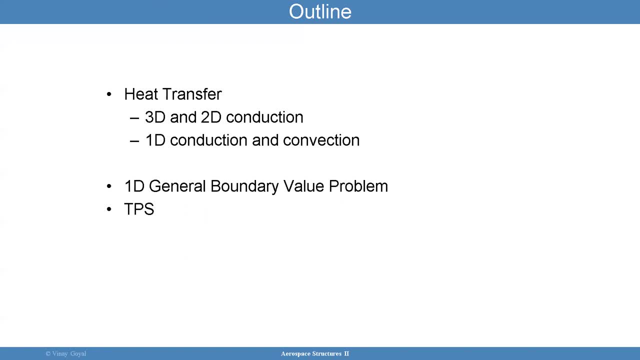 application to heat transfer. today, the 3D and 2D conduction, 1D conduction and convection. We're then going to move to TPS. Thermal protection systems are used quite extensively in our in aerospace applications, So let's first study the heat transfer balance. What's going on with heat? 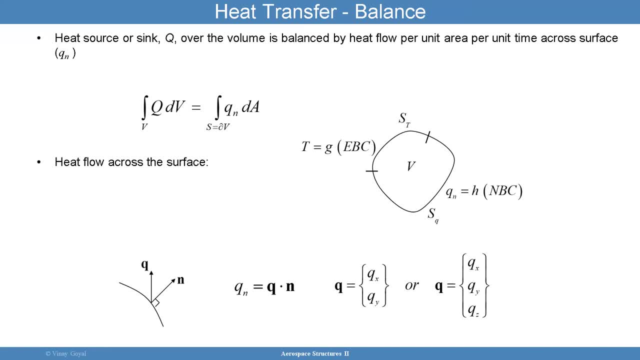 transfer balance. I think it's an important consideration that needs to be considered. We should take a look: So I have a heat source or sink Q, So that's my heat source Q, And notice how that's integrated over the volume And that has to be balanced somehow. It needs to be balanced by the 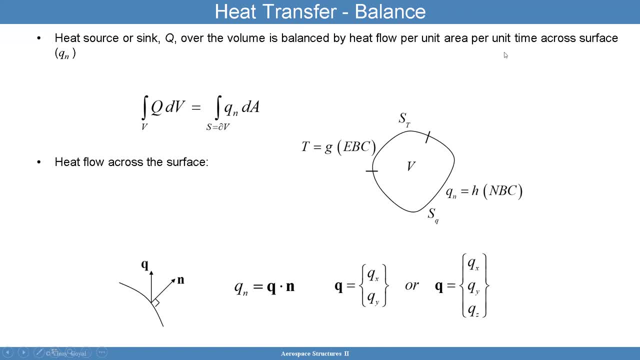 heat flow per unit area, per unit across the surface. So somehow whatever heat generation I have, or heat source or sink I have, within the volume has to be balanced by anything coming out And you can see here is Qn as an example. So if I look at a heat flow vector, so you can see here the 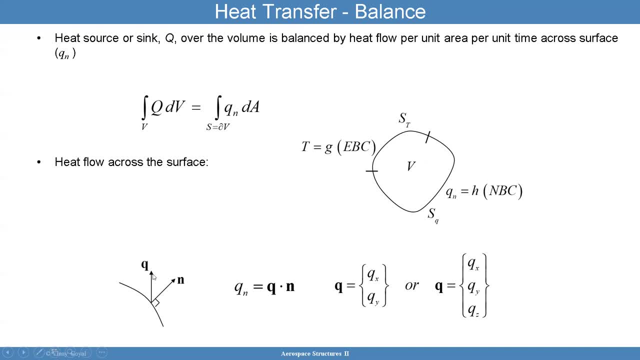 heat flow vector Q is going to have several components, But the normal component is Q dotted with a normal vector at that surface location. So Q dot n gives me the normal to that surface And Q bold is basically for two dimensional Qx, Qy, for three dimensional Qx, Qy and Qy. So that's the 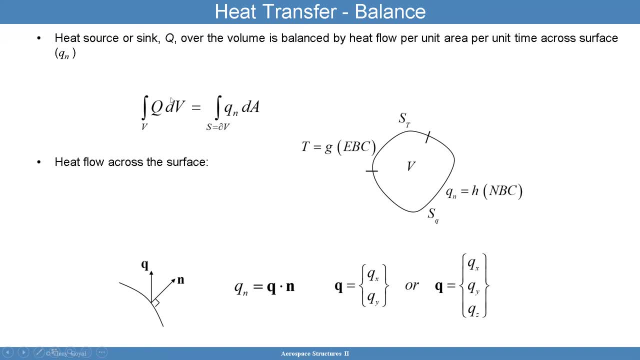 normal Qz. So this right here has to be fully balanced with what's going on at the surface. So that has to be equal. That's a volume integral. But whatever is occurring as a heat source or heat sink inside, the volume needs to be equilibrated by what's going on on the surface. That's really what this is. 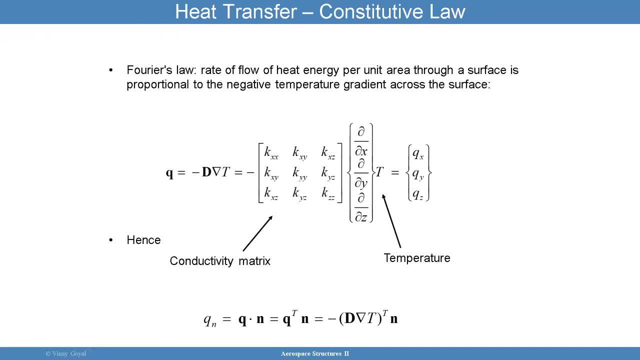 saying, telling us, and I think it's important to discuss. There's something very interesting here that needs to be discussed further, And that's Fourier-gap Fourier's law. What it states is that the rate of flow of heat energy per unit area through a 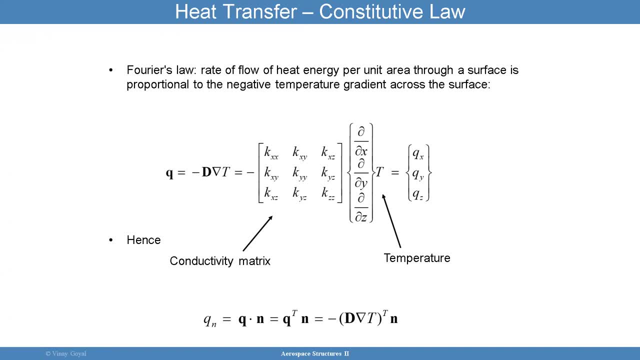 surface is proportional to the negative temperature gradient across the surface. In other words, the heat flux or the rate of flow of heat energy per unit area has to be equal to some constant times the negative of the gradient of temperature, And this d here happens to be the constitutive. 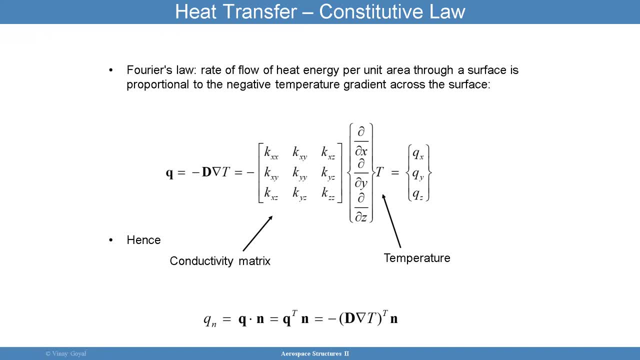 law. It's the constitutive law That tells us how quickly a material heats up or how slow it heats up. For example, heating a cork should take longer than heating aluminum. That's taken care of by d. Okay, that constant And that. 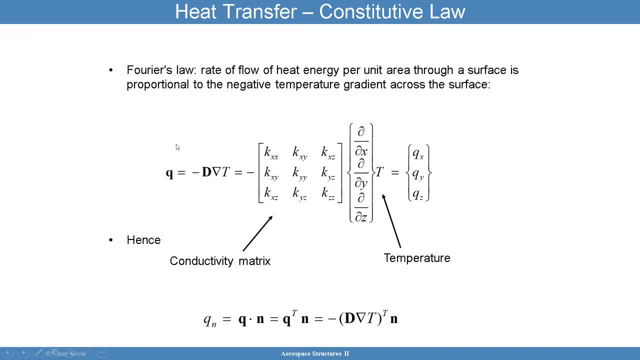 can be measured using experimental observations. So Q-bold equals this matrix here And you can see, here I have Kxx, Kxy and Kxz and so forth, Because for composite you could have a different conductivity in each direction. Now for isotropic materials. 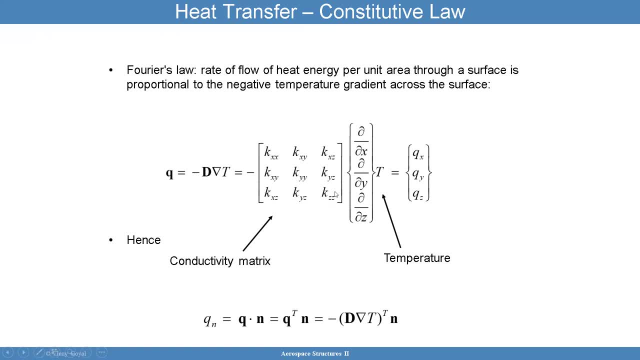 you'll most likely have K as a diagonal, K, K, K, and then you have zero in the off-diagonals And K represents the conductivity of the material for isotropic materials And in this case it's fully anisotropic. Now I have to take the gradient of T, And the gradient means this: If 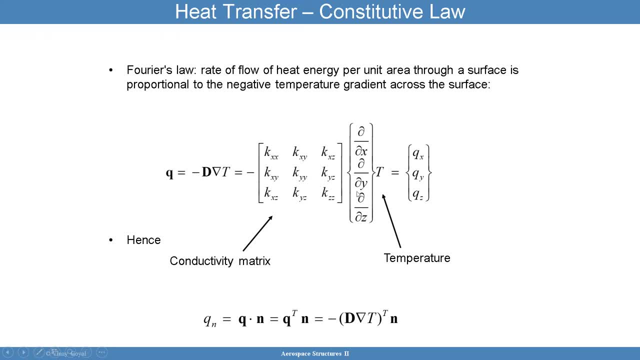 you've never seen it before, that's the gradient of T. So if you've never seen it before, that's the gradient of T. Sorry, the gradient, The definition of gradient. This gradient is applied to T And this multiplication is what gives me the components of the heat flux on the surface. Qx. 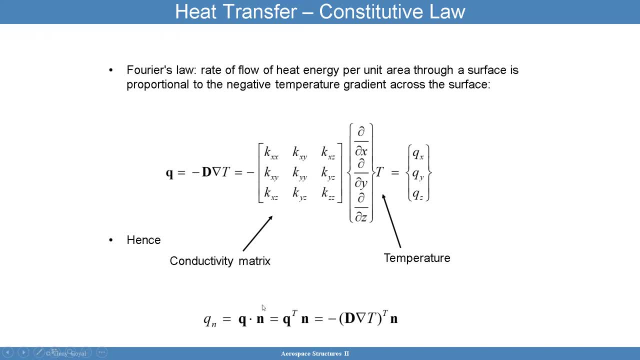 Qy and Qz. So when I go back to the definition, I have Qn, which is Q dotted with n. Then I can substitute what Q really is, which is D, b gradient of t, and i substitute it here and i get qn equals that. so with that said, 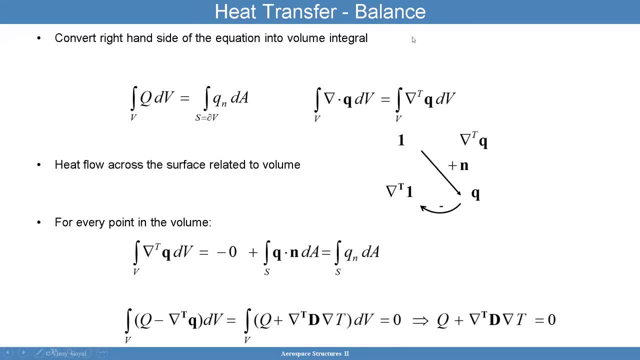 and so we want to convert the right side, we want to convert this equation into volume integral. right now this equation is unusable because here i have a volume integral, here i have a surface integral where- i have good news for you- we can use a gauss theorem or stokes there, one of those. 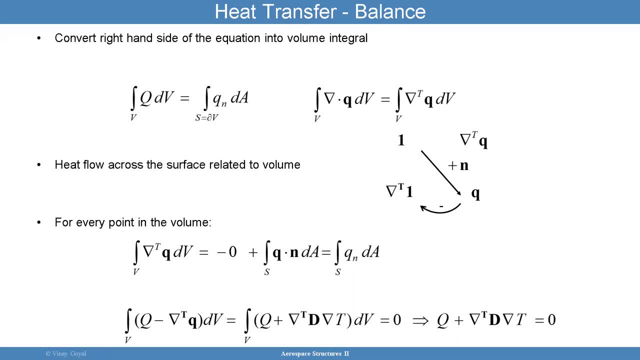 theorems where you can convert a surface integral into volume integral. and when i think about that concept, what i'm really talking about here is integration of our parts. you may have seen that in calculus i like to call it integration of our parts. the gradient dot, q, dv equals the gradient. 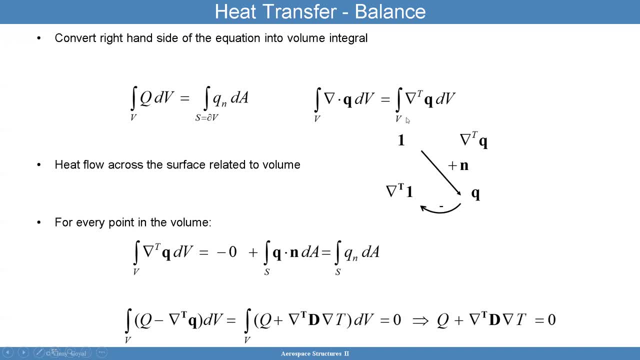 transpose q, dv, and so i'll integrate our parts by pretending there's a one there. that's not there. i'll put one on the left side gradient of transpose q, and then i'll draw an error here. plus n. i'll remove this gradient but pass it to the one and the gradient of one is zero, because the 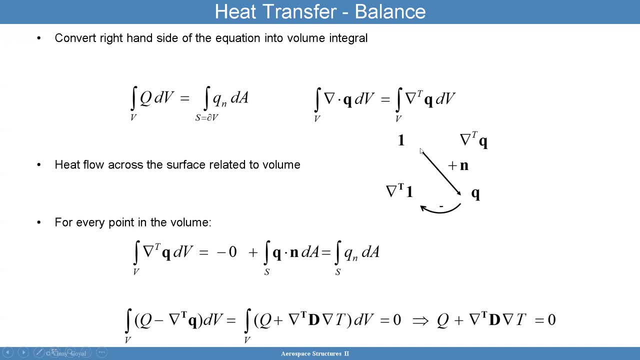 derivative of one is zero. so what i'll do is i'll multiply this cross term and put in the boundary. you can see that there that's a boundary. q dot n. you can see that in the boundary. so what is the boundary of a volume? the boundary of our volume is a surface integral. 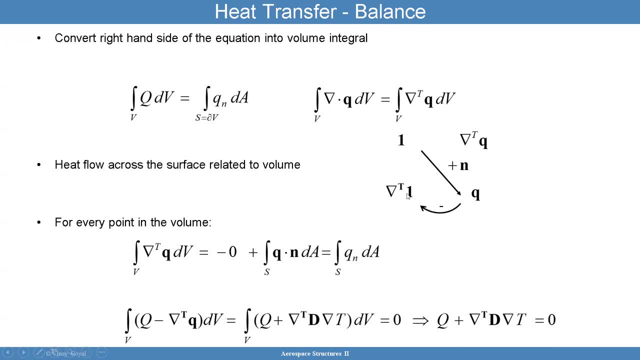 so that's what you see there, right? and then the gradient of one is zero. so zero times q is zero, and you can see that there. so i'm teaching you this theorem, i'm teaching you how to do it without memorizing the theorem, but yeah, this is how i do it. 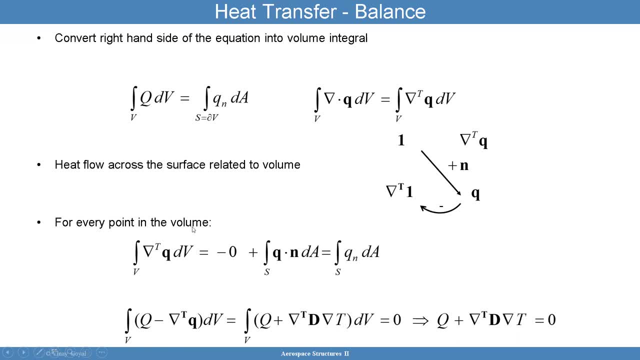 myself, and so now i have a way of converting this surface integral into a volume integral. so this must be equal to that. that's the meaning. so, because i'm able to do so, and it's a mathematical miracle, also because this is telling us, if i know what's going on on the surface, i know what's going. 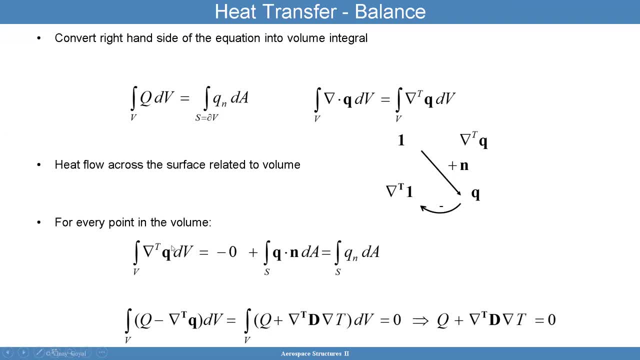 on in the volume, which is quite incredible actually. so i can substitute this term by that term and i can put everything on the left hand side, and when i do that, i get q minus gradient of q. now i know what q bold is, because q is a. 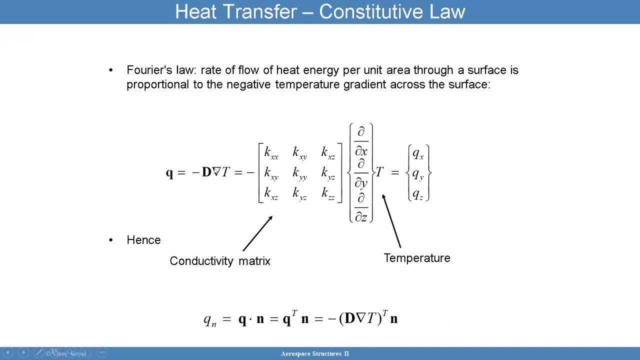 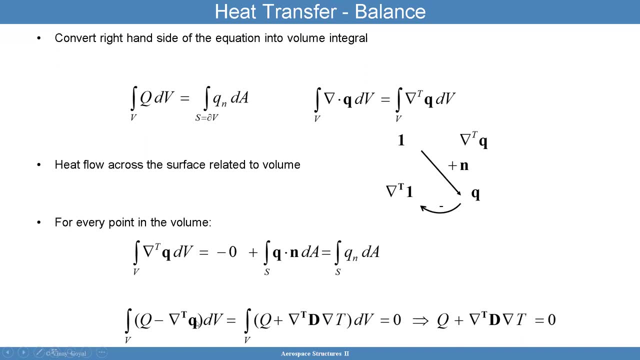 heat flux on the surface, which i have found to be d gradient of t, and i can then plug it in here: because q is d gradient of t and because this has to be true for every point in a domain, the partial differential equation governing the behavior for heat transfer problems is just: 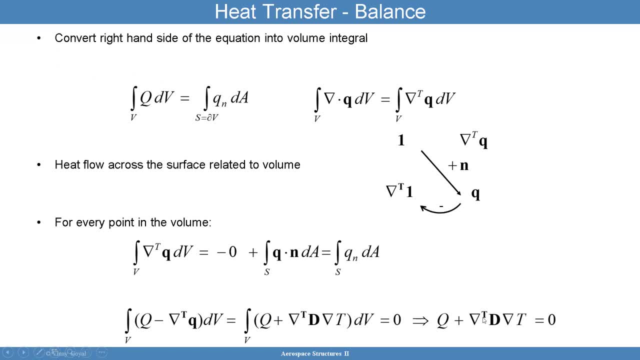 essentially the heat sink or heat source plus the gradient a, transpose d times the gradient of t, and there's a single equation here, just one equation. this here is a one by three, these are three by three and these are three by one. so you get a single equation there and the idea is to: 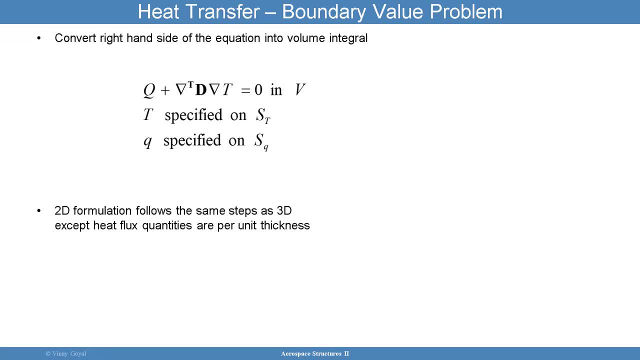 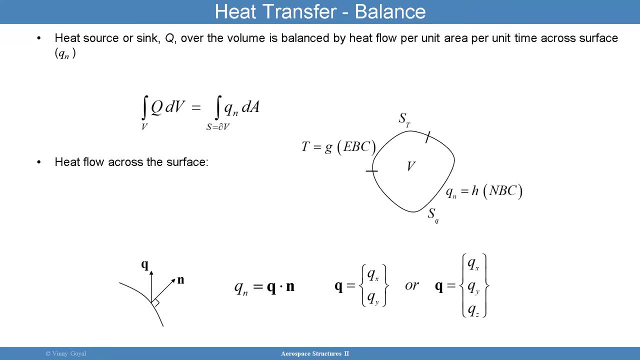 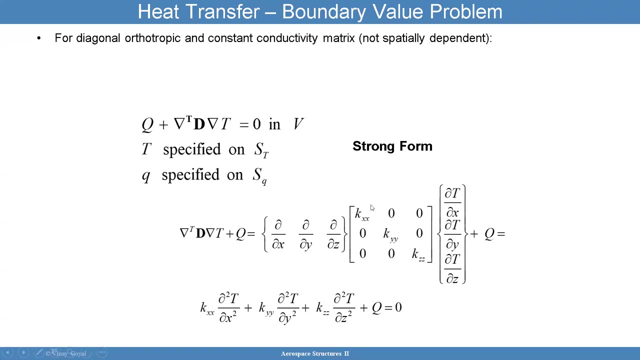 specify either the temperature of the surface or the heat flux at the surface. we can extend this to 3d. i mean, i showed it for 2d here. we can extend it for 3d. very simply. uh, the 3d version looks like this. uh, and when i'm, if i? 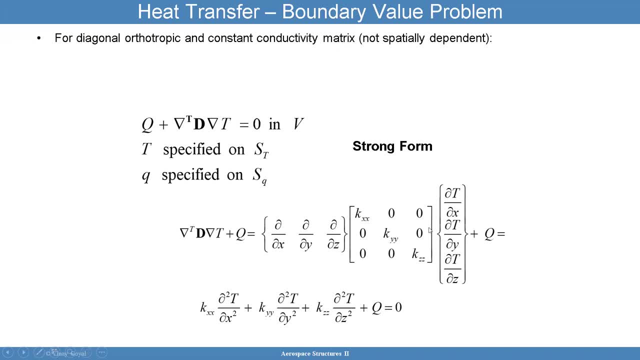 assume that the off diagonal terms are zero. the equation for heat transfer, only considering conductivity and considering temperatures applied on the surface in some sections of the surface, with heat flux applied on the surface and the temperature applied on the surface in some sections of the surface and the temperature applied, gives us this equation here, which looks a lot like the lab. 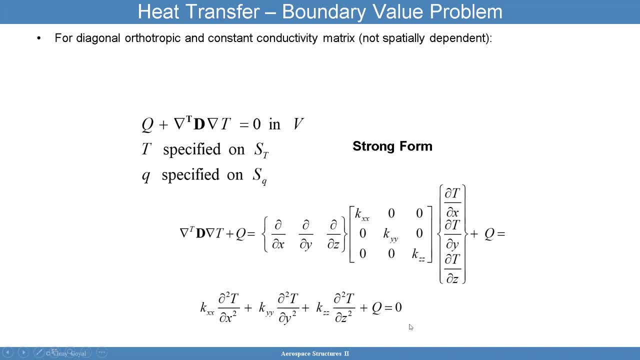 class equation. so this is the equation we want to solve for heat transfer problems: t. here is the unknown. everything else is known. k, x, x, k, y, y and k, z, z are the conductivity of the material which can be measured in the lab, and q is a heat source, or heat sink, which is known as well. okay, so. 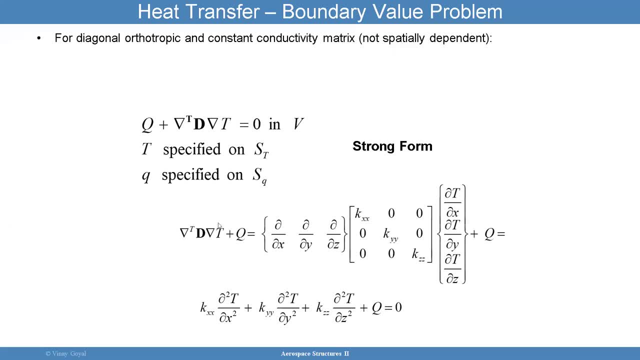 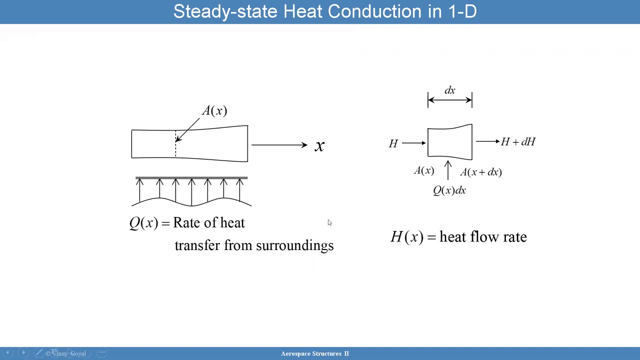 continuing on. i'm going to call this a strong form of the pro, the strong form of the problem, and so continuing on here. um, we're going to be looking at some advanced concepts on that. let's look at steady state heat conduction, so now you could have conduction on the side. 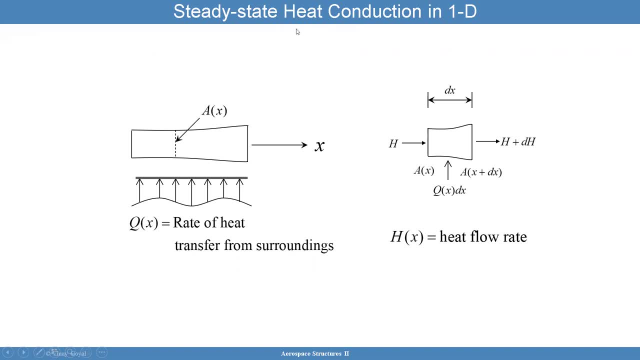 you have, and these were just 1d. right, i covered the more complicated 2d and 3d, but to show you in 1d if i have a rate of heat from the surroundings. i can do a little cut here. so these h the heat. 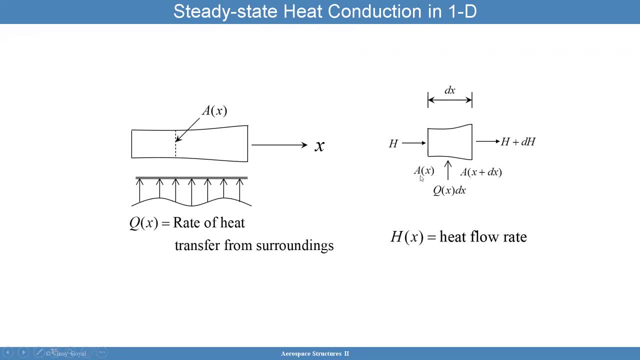 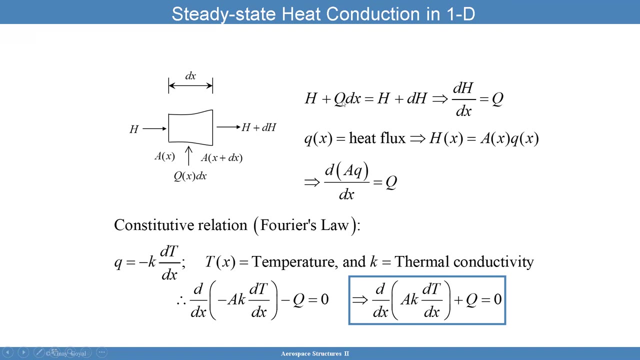 flow rate and this h plus dh, the area is ax, the area dx a ways a x plus dx. and here i have my heat, the heat transfer from the surroundings. i can take this free body diagram and kind of write it out: so h plus q dx, so this h plus the heat going in qd, qx, dx has to be equal to h plus d, h plus dh. um right. 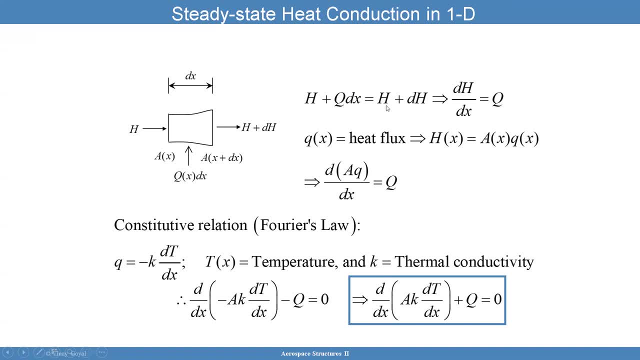 so that's heat going in and qd qx dx. so that's the heat going in and qd qx dx. so that's the heat going in and heat going out. so that has to be equal um, and you can see here that i can now cancel h. 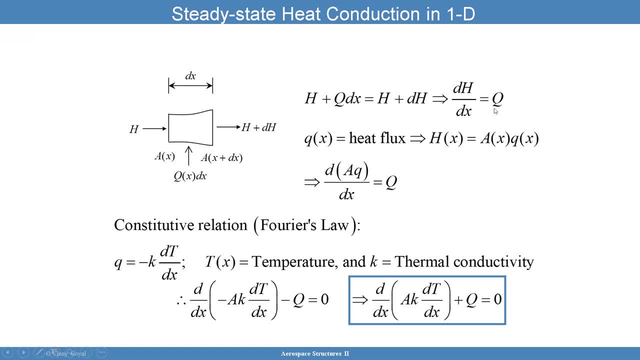 and i have then dh, dx equals q. the heat flux then becomes: if i look at in terms of area um cross section, then i have a heat flux quantity and that will be hx equals a times q right the area cross sectional area. so i can now substitute this: 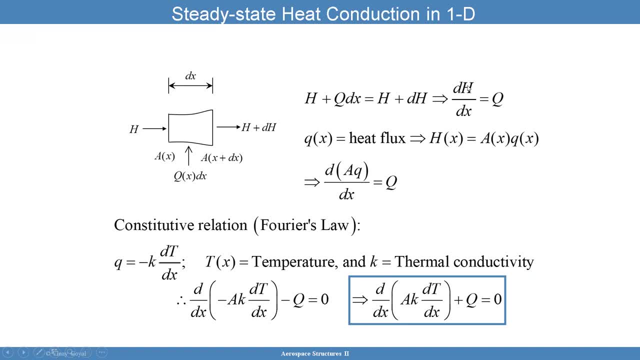 heat flux, this quantity, and i can now substitute this heat flux, and i can now substitute this heat flux, the quantity per unit area, into this equation. so i get d aq divided by dx respect to x equals q. a is known, because that's the area distribution and we're just trying to 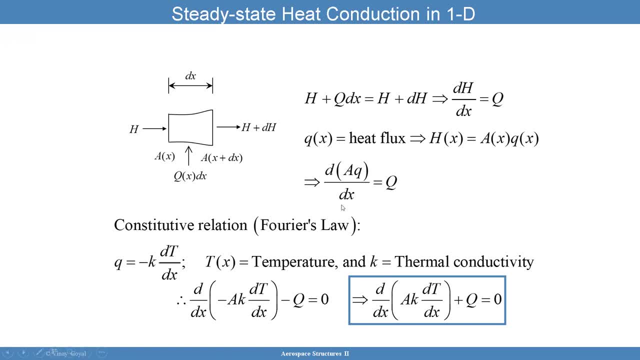 figure out how to now proceed from here. the one different dimensional version of this is that q equals minus k, which is the conductivity of the material, dt, d, x, and so now i can plug that in into this equation to fully get the steady state heat conduction problem for 1d. so now i have to do solve this. this one is easy to solve, you can. 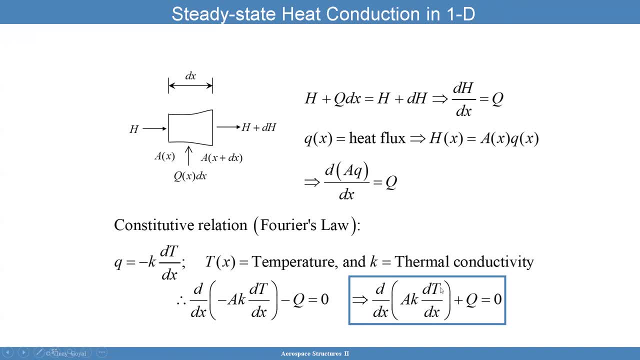 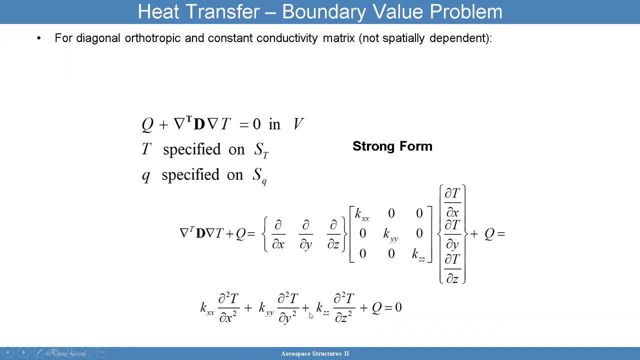 integrate it once and twice and you can solve for t's a polynomial, quadratic polynomial. so this is the same thing we saw here. it's actually almost the same. if i wanted to look at 1d, i just cancel. just turn this term to zero. turn this term to zero and this equation. 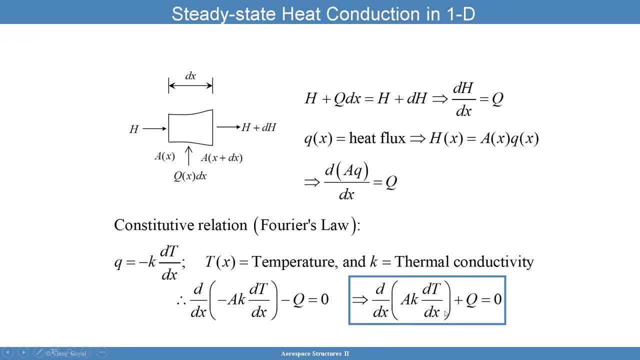 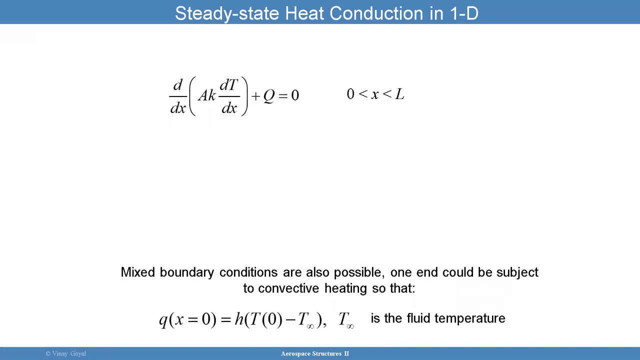 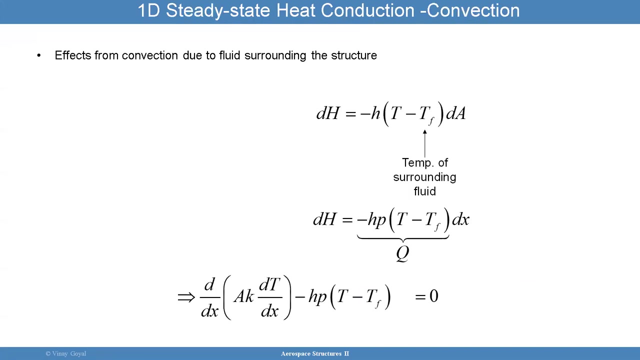 the first term and the very last term is, in essence, what i have here, in essence, if you think about it. okay, and i forgot to mention, i was applying conservation of heat in equals heat out. so that's the key there. that, i think, is quite straightforward. so, um, i could have. boundary conditions are interesting. for example, i could have: 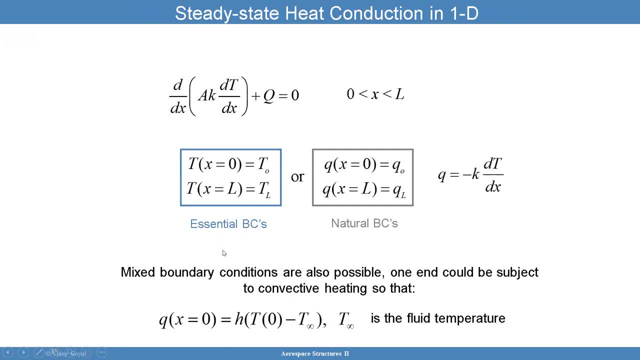 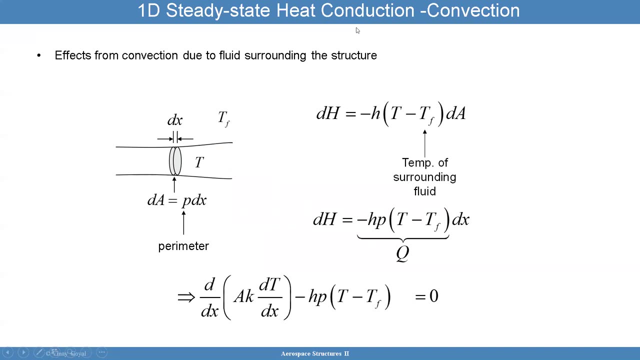 this. i'm sorry. i could have the boundaries, uh, to be related in some ways to, um, i could have boundaries that are subject to convective heating, for example, uh, the effects from convection. so assume you have convection on this side, right, there's convection on this side because there's a fluid surrounding the structure. well, 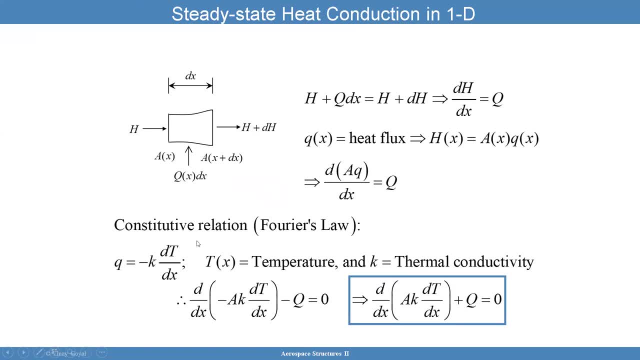 um, you see this term q here. that term q is a heat transfer from the fluid into the structure, for example. so i can take that q and figure out what to do with that q. that q can be calculated very easily. so i can take that q and figure out what to do with that q. that q can be calculated very. 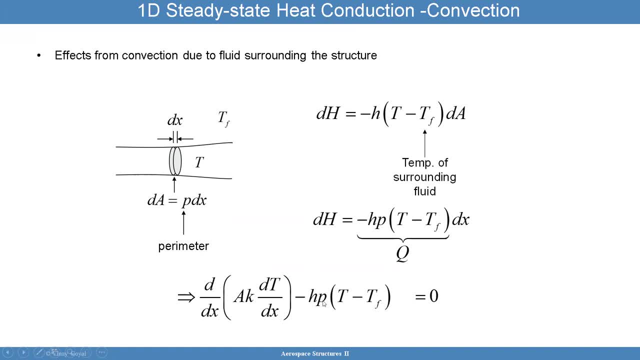 easily, so that q is going to be defined as hp times t minus t of the fluid, and h here is a heat transfer coefficient and p is a perimeter, now the perimeter of that particular location. what's interesting here is notice: if the temperature of the structure is the same as a fluid, then this: 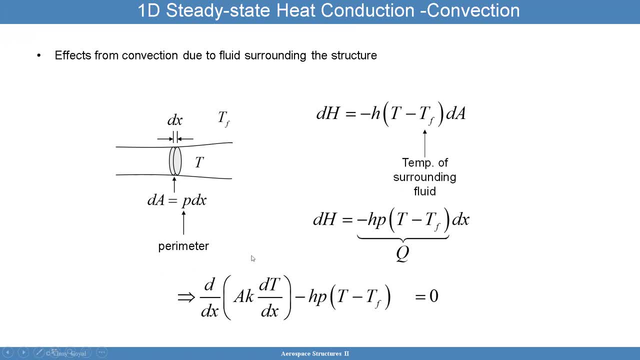 term vanishes and so there's nothing going on in terms of transfer of heat from the fluid surrounding into the material. but this formula here is really accounting for convection. so if you have a hot, a hot fluid, that hot fluid is going to push the temperature of that structure to be to get hotter, so that it 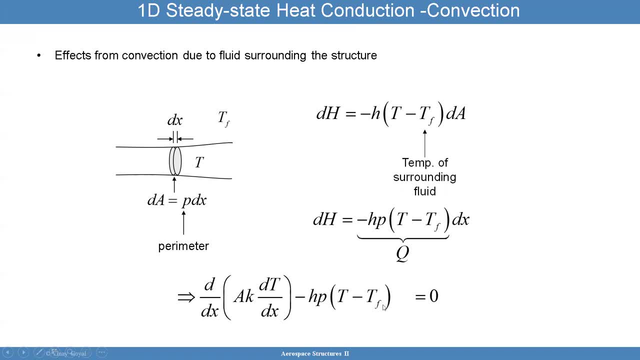 reaches equilibrium and it becomes as hot as a fluid, and when that happens, i will assume that the temperature distribution across the whole thing is likely to be tf- the temperature of the structure will become the same as the temperature of the fluid. hopefully, over time, i'll think that will happen. for example, if you have a very hot cup of ice- sorry, not a cup of ice. 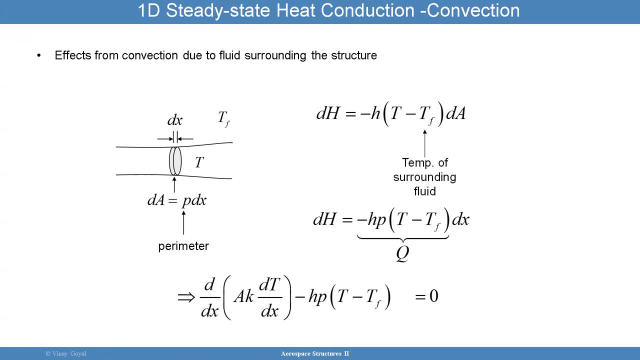 if you have a very hot cup of coffee that makes more sense and it's sitting out there, then the temperature of the cup of coffee coffee will drop so that it matches the temperature of the room that you're in now. what is causing that? what is causing that change in temperature is really convection. is the convection the fact that 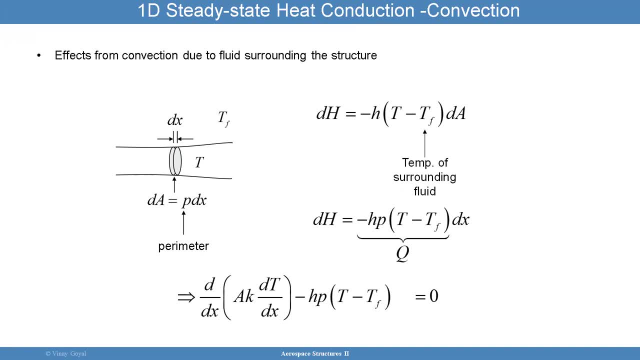 the cup of coffee is surrounded by a fluid, and that fluid is air, and that air is at a room temperature, and so this tf is, say, 77 degrees fahrenheit, while the temperature of the cup could be 100 degrees fahrenheit. so that's the temperature of the cup and that's the temperature of the cup. 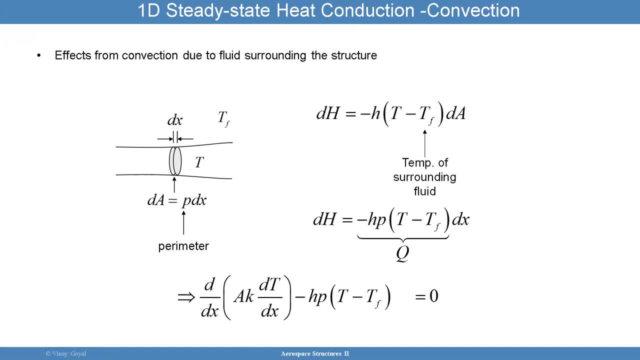 120 degrees fahrenheit, and so this temperature over time will approach the film coefficient or the fluid coefficient, the- i'm sorry, the fluid temperature. i apologize, h is a material property, or almost like a way of calculating how this h could impact. so the greater h is, the more the. 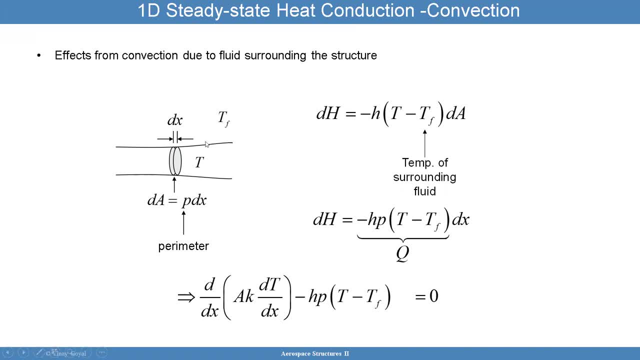 transfer of heat or out. you know heat going out or in from the fluid into the material. for example, if i have a coffee cup and i have a convection oven and i put that coffee cup in a convection oven and there is no air moving, that should take lower time for the cup of. that should take longer time. 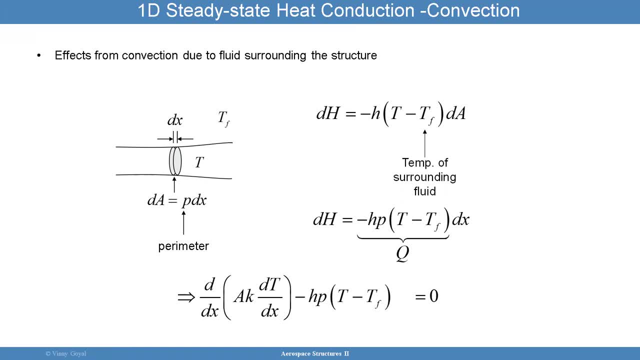 for the cup of coffee to warm up, compared to a situation where the convection oven is blowing hot air at very high speeds into the part. so to the question that i'm going to ask you is: what is the flow of the fluid and what that is? the flow of the fluid in the flow of the fluid. 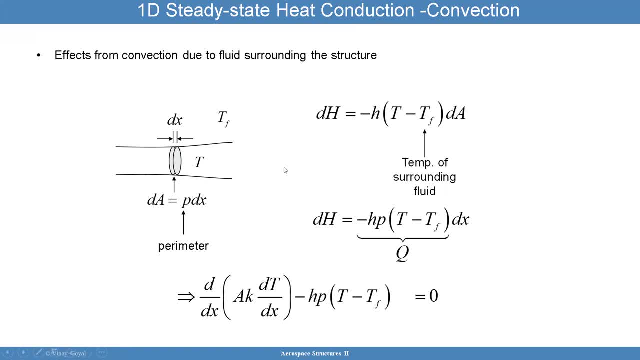 and i'm going to give you an example here- that i'm going to give you an example here that i was asked earlier how to account for convection, for example, or for vortexes. these were vortices could come into play, because if you have vortices, those vortices are going to increase h and h is going. 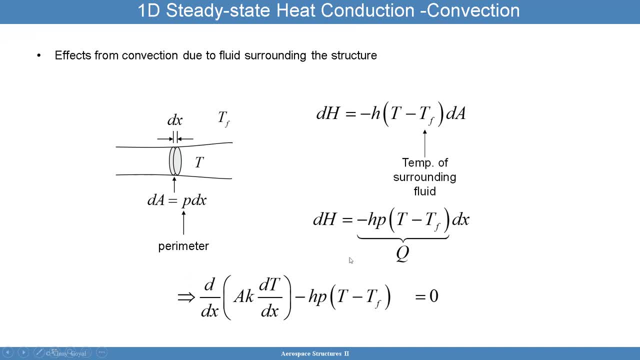 to increase the heat transfer. so h is where the fluid mechanics is embedded. that's where you want to figure out what h could be. but you know that that's kind of what we're talking about here is um, how to solve different steady state heat conduction convection problems in this case. so we went from. 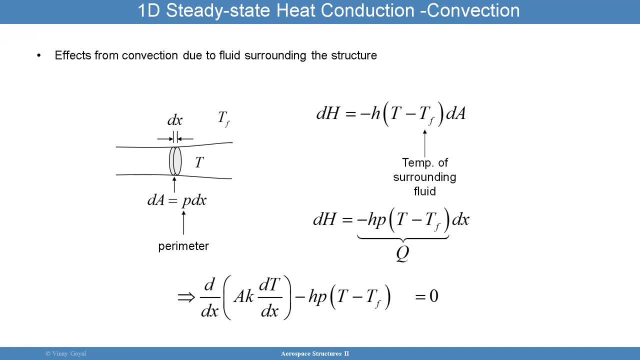 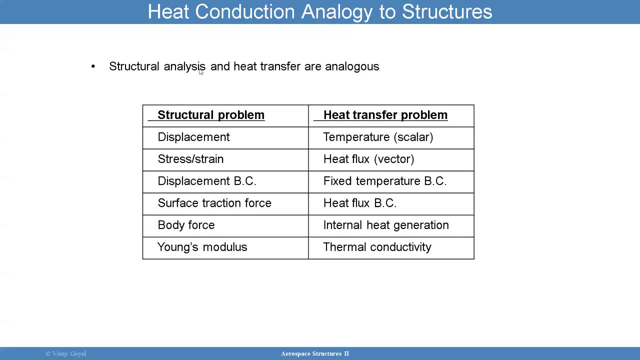 1d convection conduction to 1d steady state heat conduction convection, right, and so i'll keep moving along. i want to show the analogy between heat transfer structural analysis problems. so in terms of structural problem, you're looking at displacements. temperature is analogous to that. 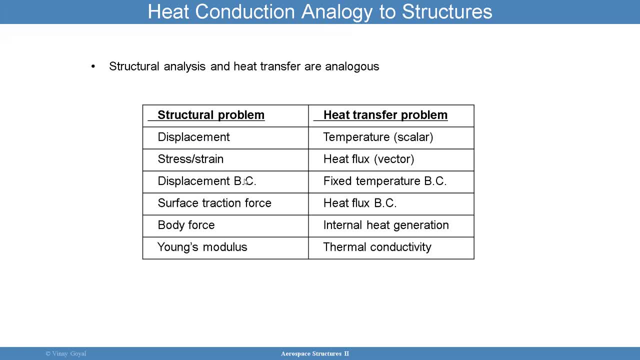 stress and strain analogous to that as it flux displacement analogous to that is fixed temperature displacement boundary conditions. what i mean there: you apply surface traction in heat transfer, you're applying heat flux boundary condition. in structural problems you have body force in heat transfer, you have internal heat generation. in structural problems you have the young modulus. 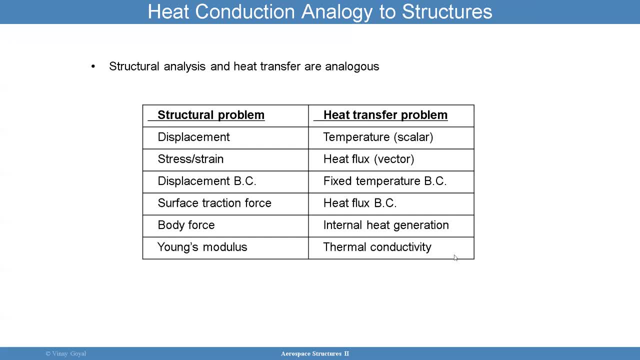 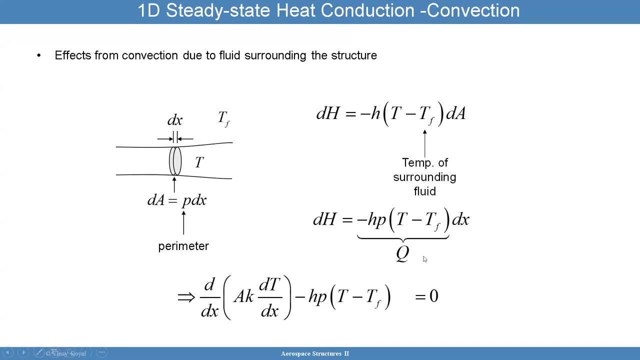 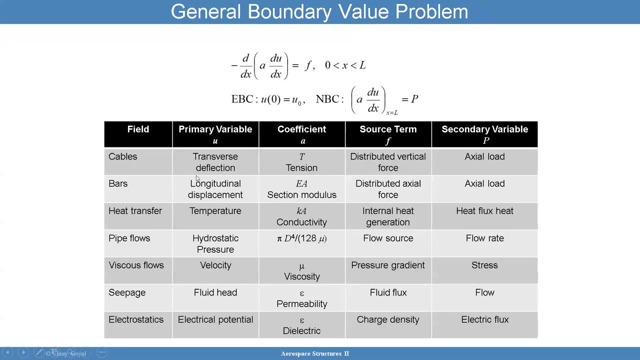 and in heat transfer you're looking at thermal conductivity, decay and also the age for convection problem. how, how efficient? basically, the question being asked there is: how efficient is the fluid able to transfer you the heat in or out from the structure? that's what that each is saying. right, because if h was zero, 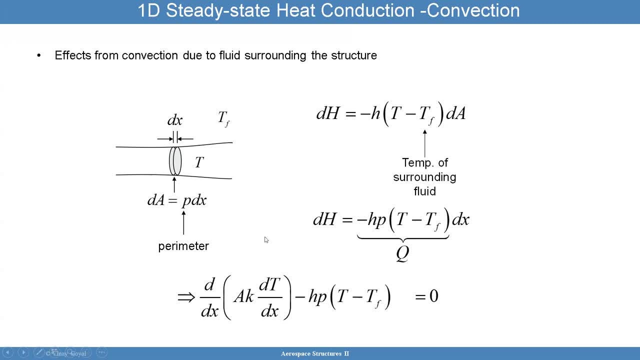 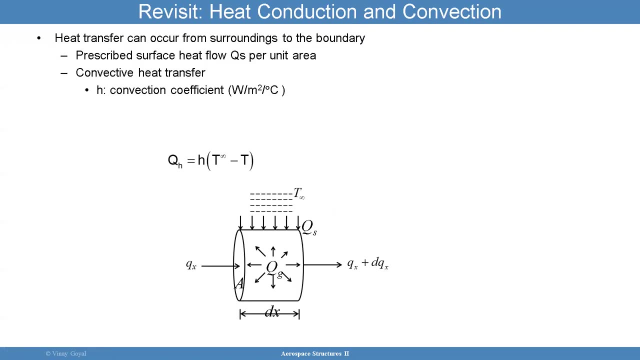 clearly, there's no heat transfer between the fluid to a structure and vice versa. so h, the higher the h is, the more transfer is going to occur, and so, and the faster, potentially so. so that's what the h is telling us and that's what that's about. so, uh, so yeah, just to summarize, heat transfer can occur. 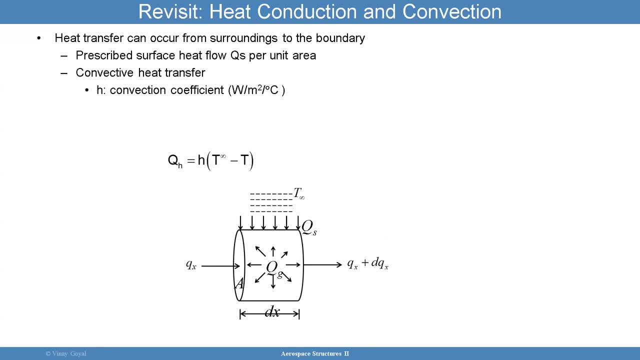 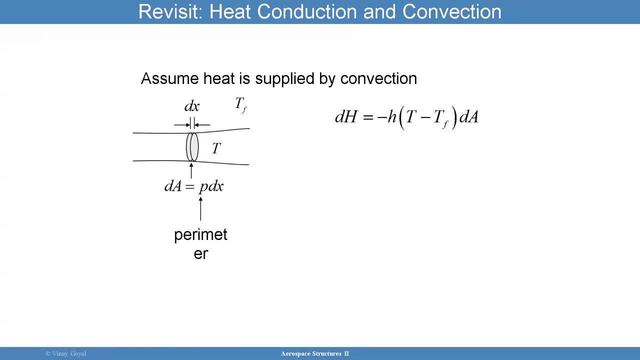 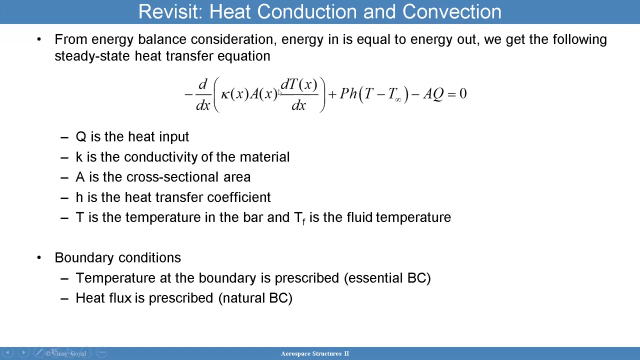 from the h is telling us, and that's what that's what that's about. so a and i can add more terms, so i can even add more terms in case i have radiation or something else, But the bottom line is that I have the heat conduction conviction problem in this. 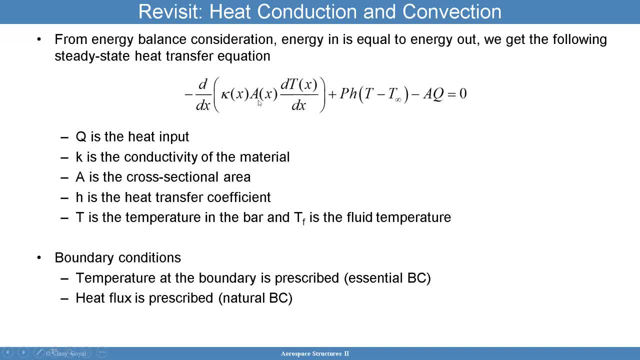 equation here: K is the conductivity of the material, a is a cross-sectional area, T is a temperature, H is the heat transfer coefficient, P is a perimeter, T is a temperature of the structure of the surface, T- infinity here is a fluid temperature. and Then a is a cross-sectional area and Q is the heat input. that could- I could even apply other types of heating boots. 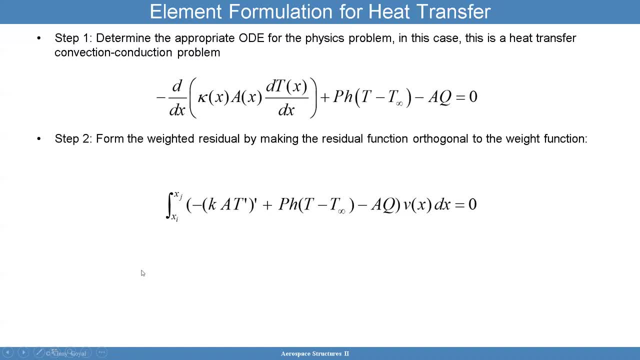 and then I will have: boundary conditions are specified, and So what I want to talk about. I don't want to go into the nuts and bolts. You know I don't want to go through every single thing and how to formulate the final elements, But I want to kind of show you the basic premise. So you have this equation. 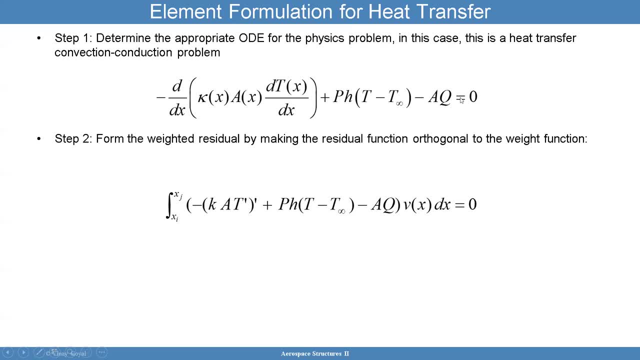 What you do is you take this equation multiply by some, some some sort of Function which are called V. So that's kind of the step that people take when they want Approximately solution to this partial differential equation. This is covered a more in advanced course. This course is advanced course but we're looking more at. 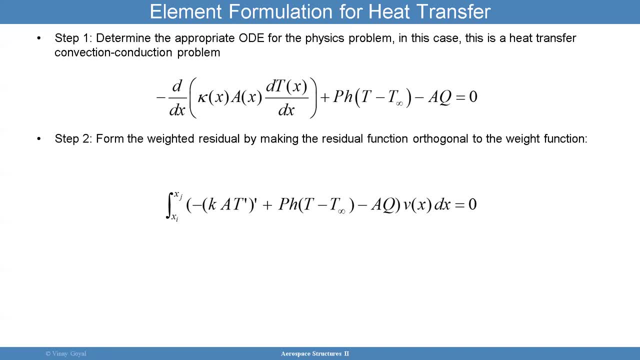 Applications. So in this particular lecture what I plan to do is cover a very top-level mechanics of how this equation can be discretized into the mirror mathematical miracle of a linear algebra problem where I can solve for temperature by just simply inverting the stiffness or the conductivity matrix. 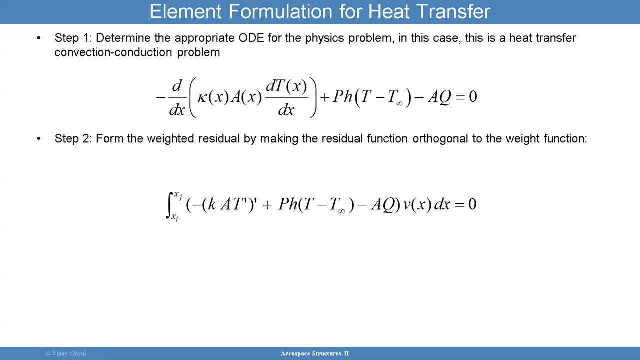 and and and. Yeah, just simply find the problem to that extent. So what I've done here, I've written this again and I multiply by V and I integrate this over the domain. I call this the weighted residual. That's what we call the. the problem We're. 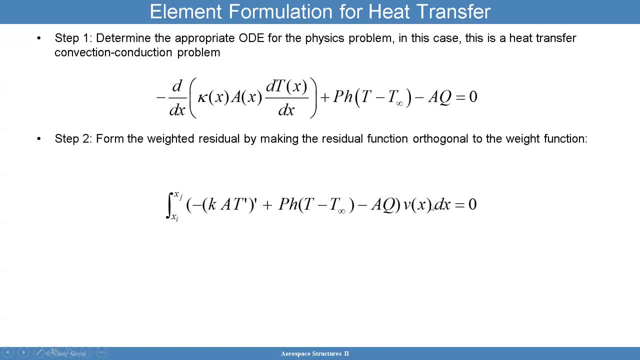 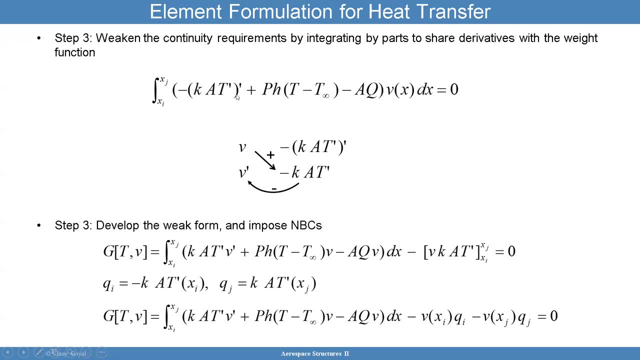 formulating the weighted residual multiplying by some orthogonal function, V that is unknown. and Then the idea is to integrate our parts in a manner such that the number of derivatives Here for the primary variable of interest, which is temperature, is shared equally with V. So we're just only doing the integration of our parts on this first term. 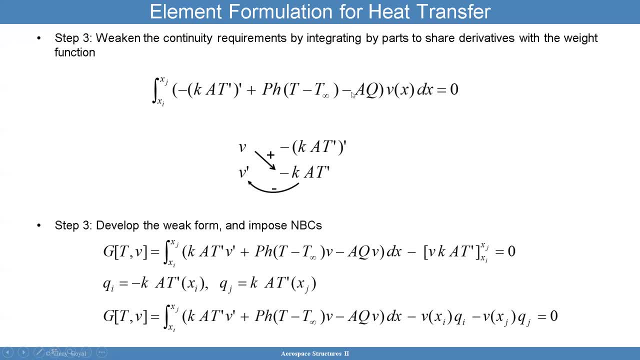 Not the second or third term, because they don't have derivatives. So to integrate our parts, very similar to what I showed earlier, write V on the left side, Put this on the right side, remove a prime and put it on the left side instead, and now I do a cross plus. 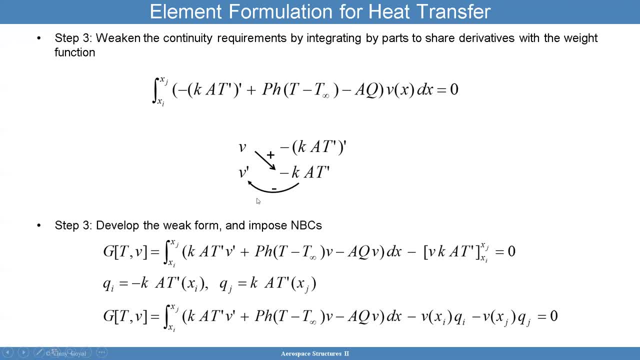 minus what's in, what's at the bottom of this integral goes back inside the integral. like that, it replaces that term. you can see here: k at prime times, V, prime is exactly that, and Then this cross term becomes your boundary term. This is exactly what's occurring on the boundaries, while these occurring inside the boundary and 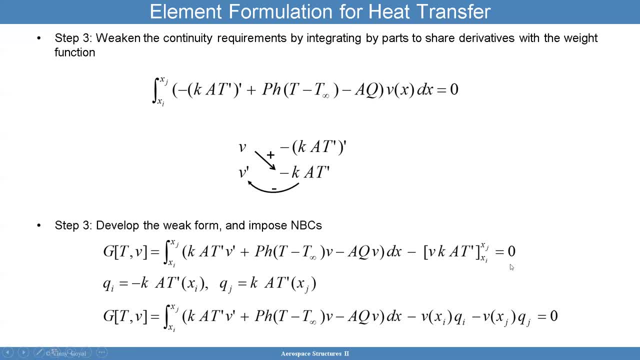 We call this the weak form of the problem, and I know I'm throwing a lot of ideas at you, But again, what I'm trying to do is explain Why we You know, is is is derived from a very simple mathematical principle, and this thing is called the weak form of the. 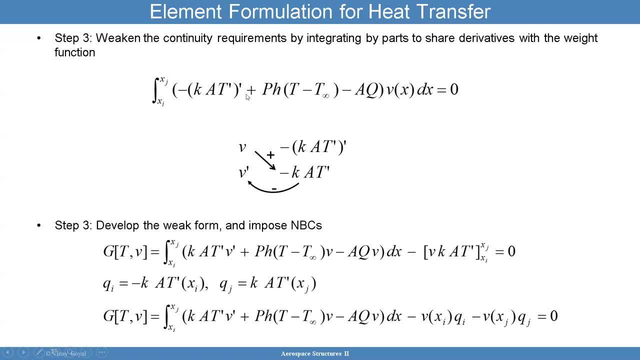 problem and why it's called the weak form of the problem, because i took two derivatives and got rid of one of them and i've weakened the continuity requirements. for example, if i have a linear function for temperature, the second derivative of a linear function gives me zero, so a quadratic. 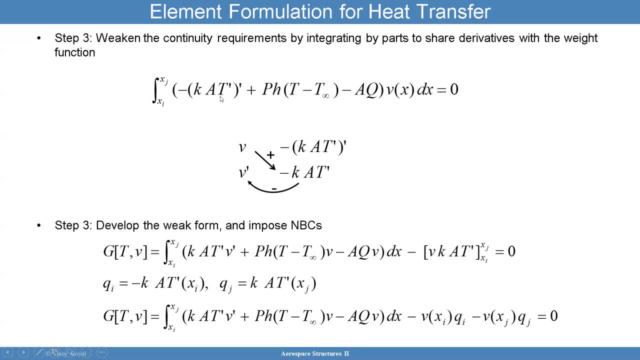 function. second derivative of that gives me a constant. so you can see that by lowering the order differentiation, what i've done is i've weakened the continuity requirements. now the temperature could have a linear function and the rate of a linear function gives me constant, while here in the original premise of the problem, t double prime disappeared because the derivative. 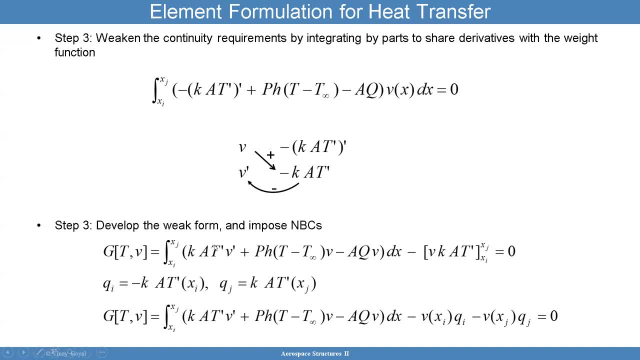 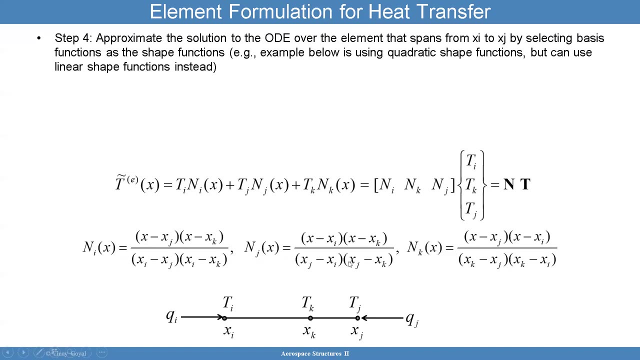 of linear function is zero. so that's the benefit of the weak function, and it allows me now to use approximation function. polynomials are very simple, like linear function and so forth. um, and i don't want to go into more detail here, bottom line is: once i have 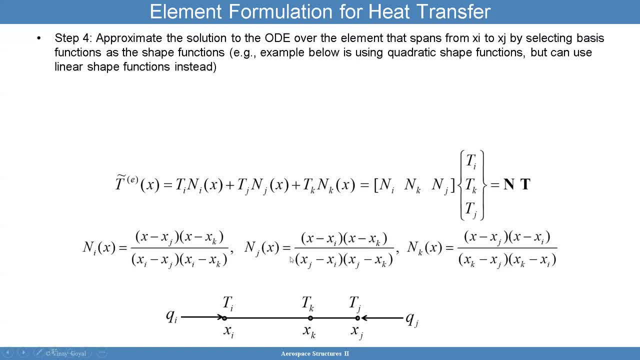 this weak form derived. now what i need to do is to derive in a polynomial approximation of some kind, and i know you see a lot of numbers here and it's very confusing, but just bear with me, because i think it's simpler than what you will think. 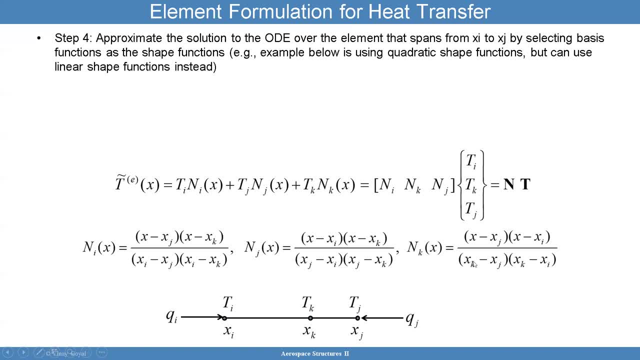 so these polynomials are selected in a very smart way. they're selected so that the unknowns, the temperature unknowns, are right at the nodes. so say, this is a single element and the unknowns for this polynomial approximation are going to be these coefficients t, i, t, k and t j. these polynomials are selected very carefully. all these k, x, j, x, k, all these are 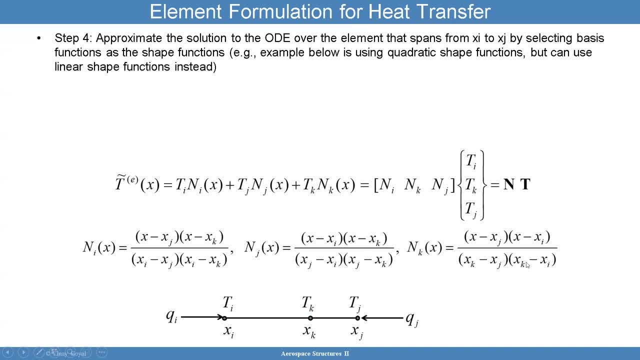 numbers, so you don't have to worry about that. these are all numbers and they're going to be all numbers, all numbers, and all i've done is approximated the solution over this domain. i have approximate solution over that domain using this polynomial. i'm just giving you the. 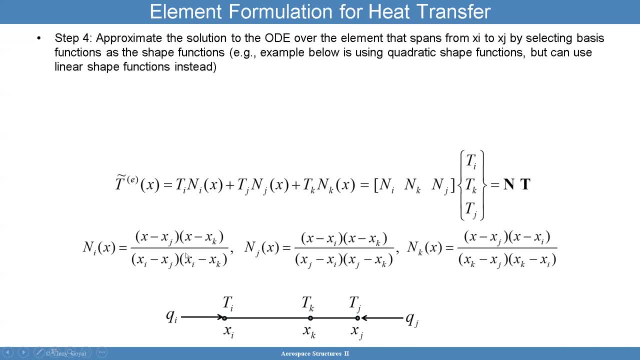 formula so you can see what it is and you can see that these polynomials vanish at a particular location. for example, this polynomial vanishes clearly vanishes at j and k. for example, if i put x- j for x, this goes away. if i put x- k for x, 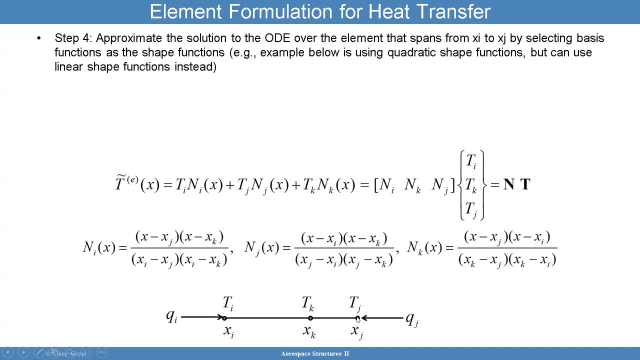 this goes away. so this polynomial is zero at that node and that node. but this polynomial is one. it has a value of one at the node of interest t i. you can see that if i put x- i here, x i minus x j cancels out. x i minus x k cancels out with this. so i get one. so these polynomials are carefully. 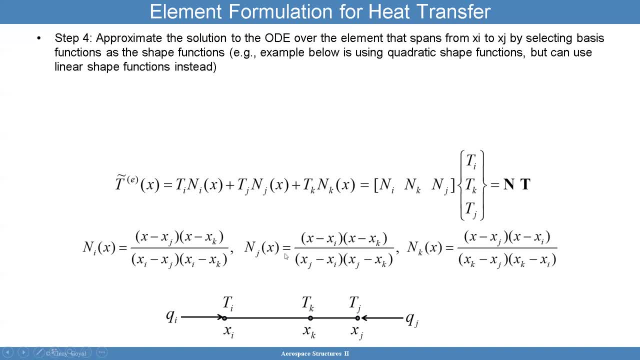 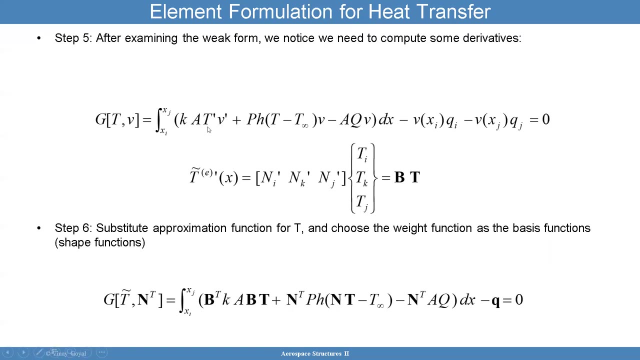 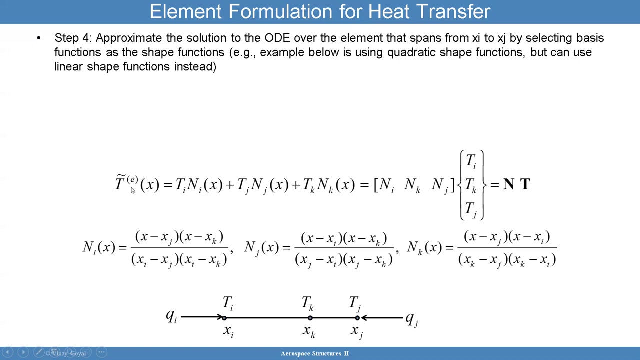 chosen in such a manner that i recover the temperature at that particular location, which is incredible idea. so once i have this temperature approximation over that domain, i'll then proceed to plug it in. i'll plug in this approximation into this, and here t can be written as the polynomial approximations times the vector. 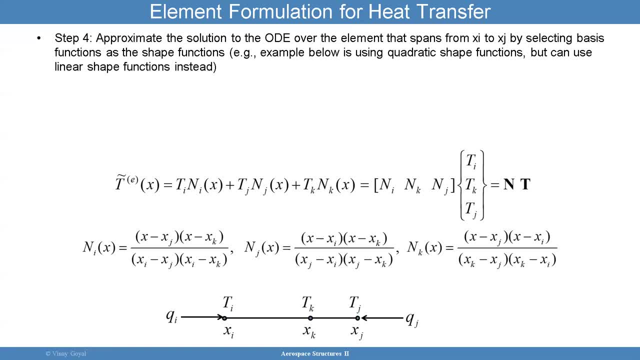 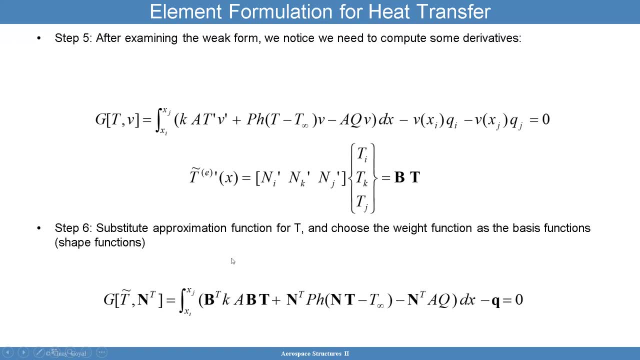 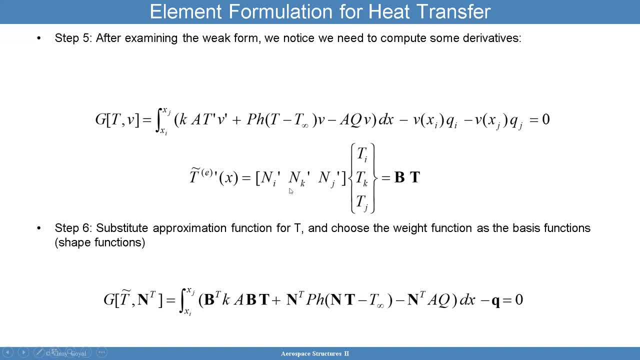 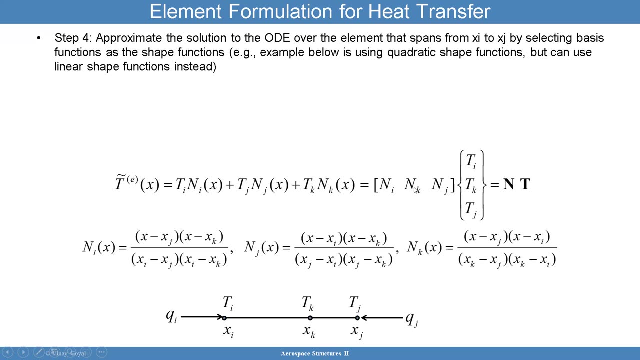 of those polynomials. t are constants. i don't know them, so i get b times t. i'm going to call this whole thing b bold. now i'm ready to substitute these things into here, and all i'm doing right now is: anytime i see t, i'll plug it in for n bold, t bold, which is basically: 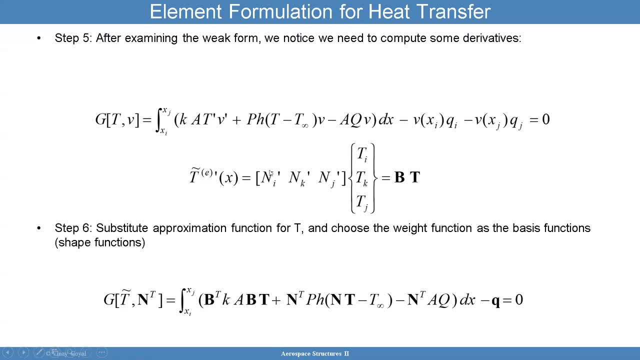 these polynomials times, it's unknown. and you can see, for t, prime, i plugged in b bold, t, bold, uh, and then for v, i'm going to plug in uh, basically, uh, yeah. for v, i'm going to plug in uh, t, right, so then i have the same thing here. i have t. 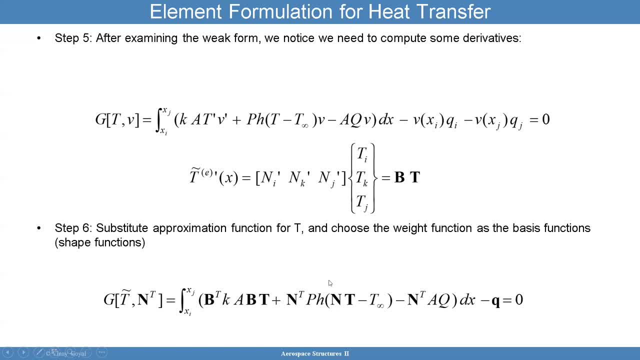 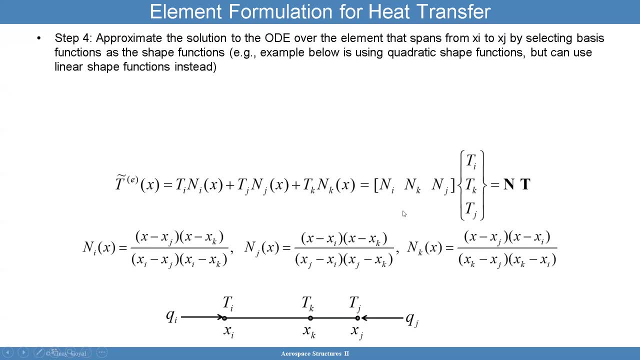 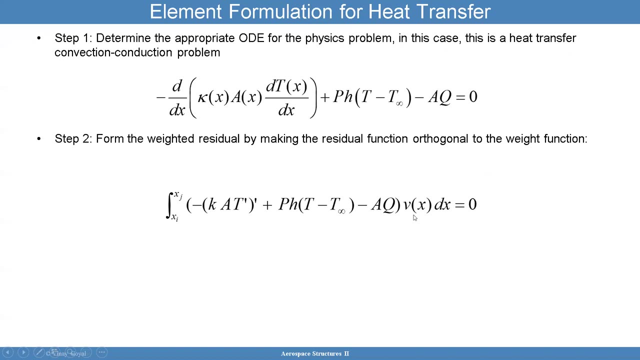 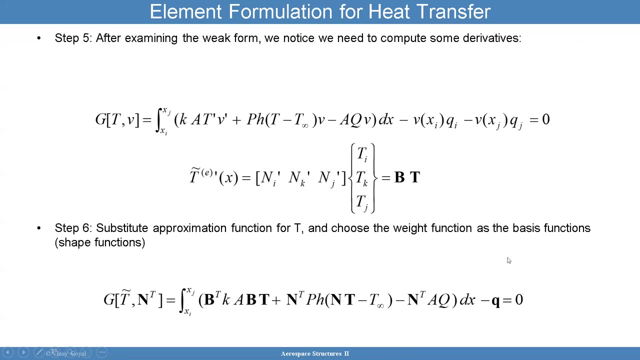 i plug in nt for that, and then for v, i'm going to plug in n, which. so let me remind you what v is. v is this function that i multiply the whole thing with, and this function is unknown, but i'm going to select it to always be this polynomial, okay, and so when you do the math, what you get is: 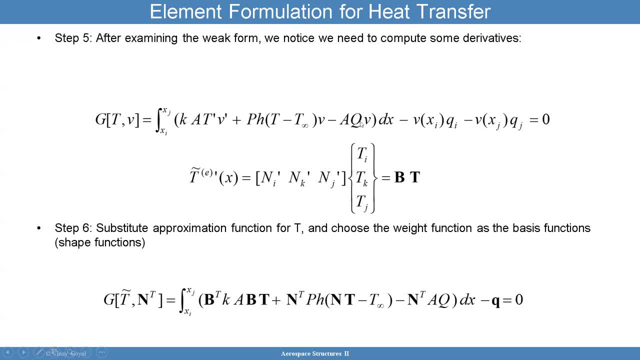 here, this equation here at the bottom aq times: v and v is the polynomials, right? so we're going to select the polynomials as, uh, the thing to be plugging in. here. you get b because the derivative v prime is v. v is this polynomial, but prime of that i call the b bold and that's why you see v to be plus b bold. 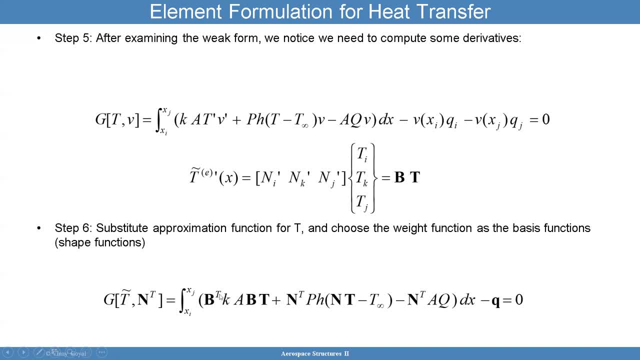 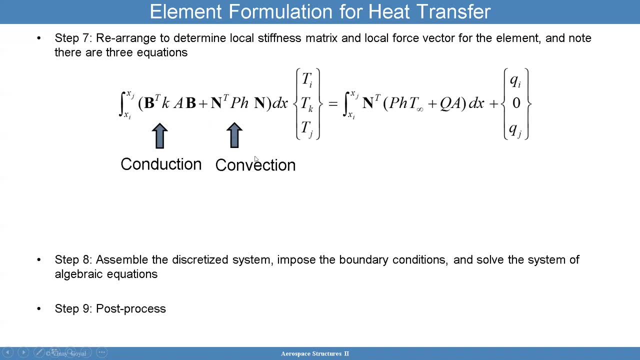 here, so very beautiful done. now i have this, this equation, that's true for one element, and this term corresponds to conduction, this corresponds to convection, and the idea now is to do this for every element and then assemble all the elements together. now, this course is not. 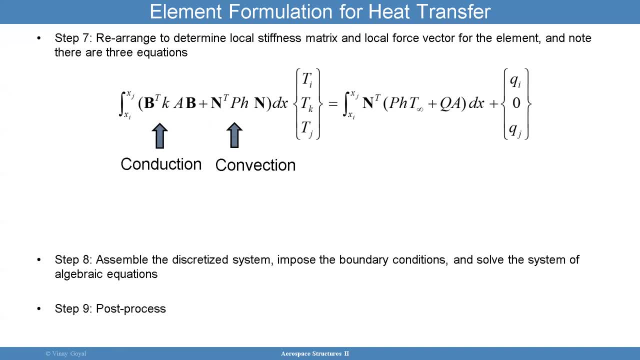 about going to a theory of finite elements, but i think it was very important to kind of show you how things work out if you were to start from first principles. so it's stuck in your head, as you're using finite elements in the various problems, that we'll be applying these to. so what? 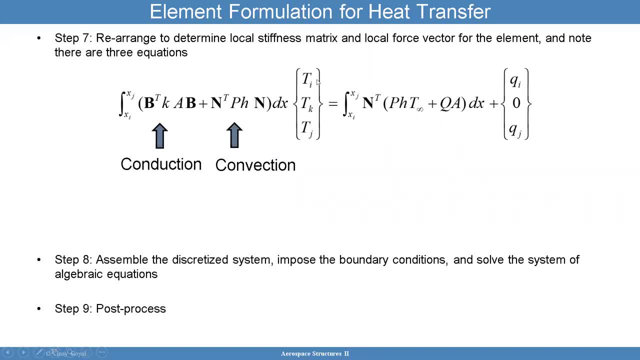 we're trying to solve for is this: t, t, i, t, k, t, j. these are the temperatures at the nodes. guess what? i know this whole thing. these are numbers, you don't have to worry. k, the conductivity, is known, a is known, the integral over over the polynomials is known. so these are all numbers. 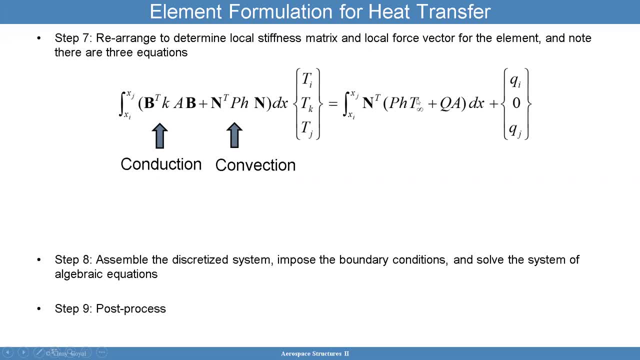 and this is going to give me a number and i'm going to show you how to solve this problem in a three by three matrix. all these are numbers and the heat fluxes are numbers, so you can now invert this using linear algebra or matlab to get the temperatures of the nodes. 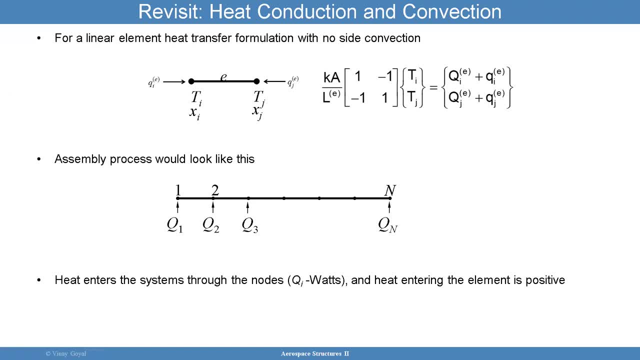 that's the beauty of that. as an example, we took a partial differential equation with just two nodes and guess what? after you apply the process i talked about, you get a very simple matrix: times t, i, t, j, the unknowns of the nodes, the temperature, unknowns of the 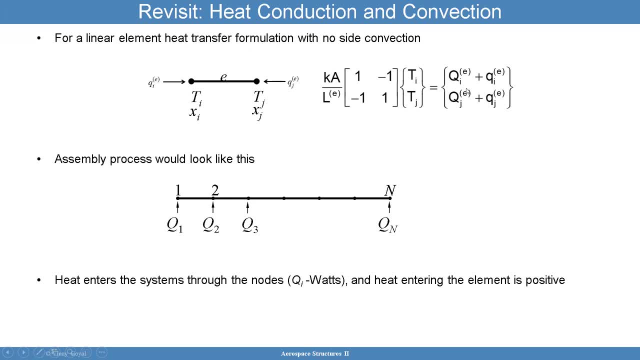 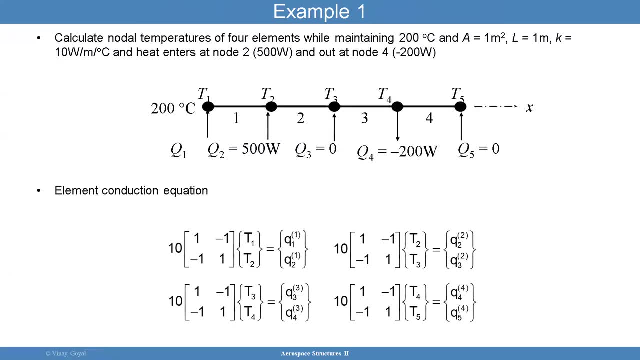 nodes and all you have to do is now invert this. given the heat flux, you can then solve for t i and t j, the temperatures, add those nodes. here's a quick example: calculate the node temperatures of four elements while maintaining 200 degrees c. so you maintain this at 200 degrees c over here the area, the cross-sectional area. so 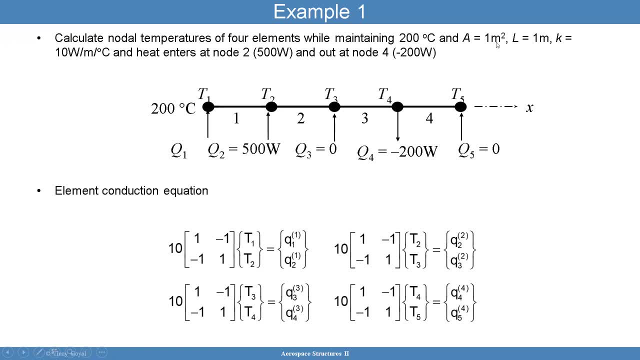 assume this is like a tube. the cross-sectional area is one meter squared, the length is one meter and the conductivity of the material is given here. the heat enters a node two. so we're going to enter some heat here and we're going to enter some heat here, and we're going to enter some heat. 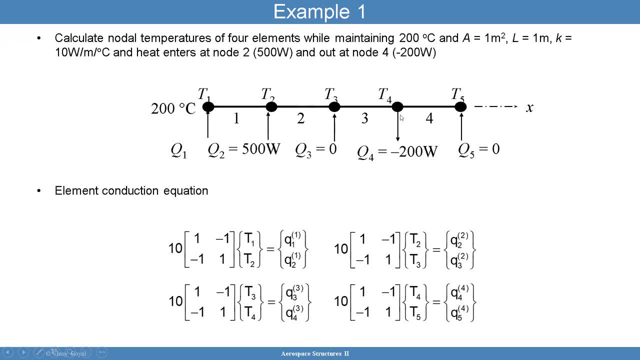 here at 500 or 500, the heat goes out at node four of 200, and so the question is: what is the temperature across the tube? so then you write the, the, the equations for each element. i have four elements, so this is my domain and f's divided domain into four elements. 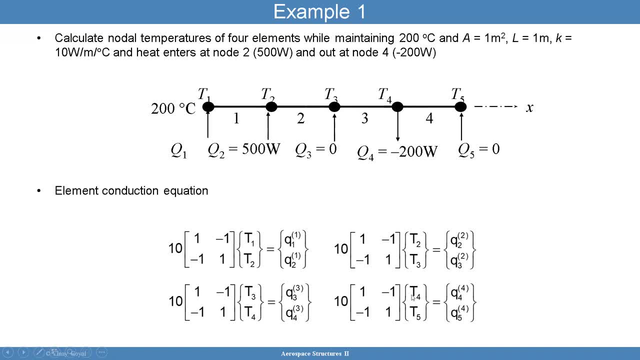 so i should have four of these guys: one, two, three, four. i want to. i won't go into the extensive details on how to assemble it, but you will assemble these four elements together by knowing that they're shared at the nodes. and when you do that process and you can see here, element one is made up of: 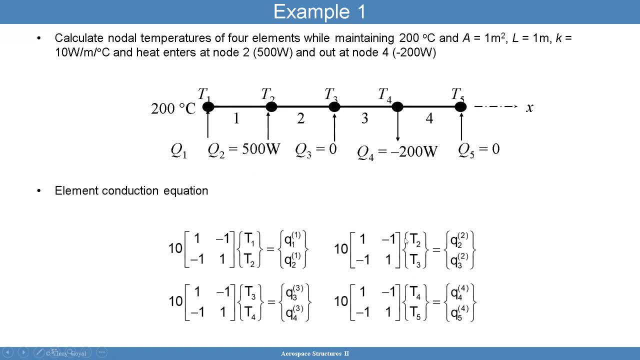 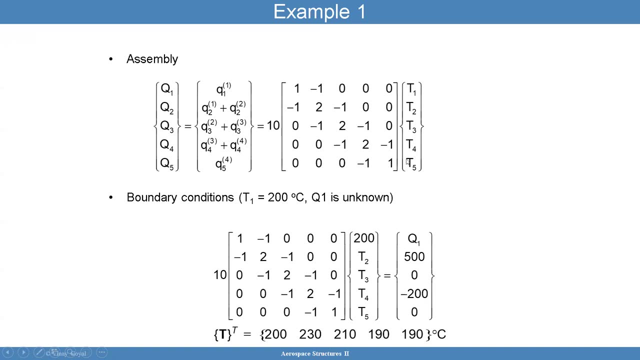 temperature t1 and t2. element two is made up of temperature t2 and t3 and so forth, so t2 is shared. you can see that there, and if you were to put it all together into one single equation, it's going to look like this: these are all numbers, and now all you have to do i know the heat fluxes at the 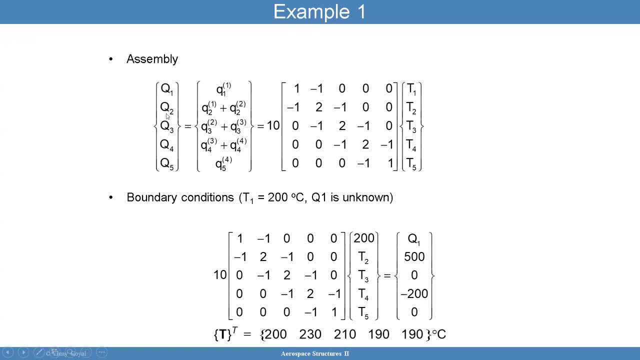 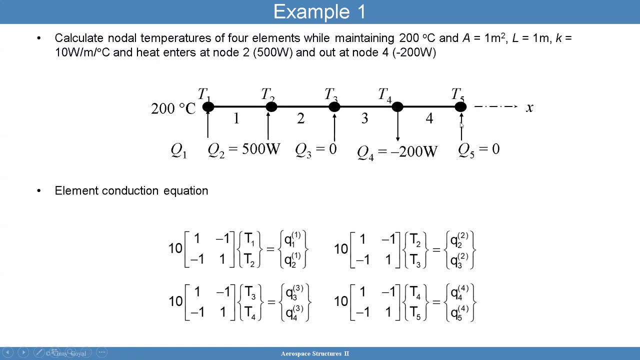 boundaries of the nodes. q1 is not known. q2 is known: it's 500. q3 is zero because there's no heat flux coming in and out, so that's zero. q4 is 200 out. q5 is zero because i have nothing going in, in or out. this one is unknown because 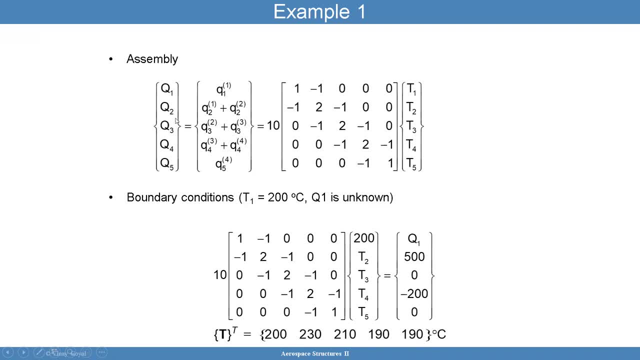 i'm specifying the temperature, so we don't know what's going on with that one. but for the rest of them i know what's going on, so now all i have to do is solve for. solve for t2, t3, t4, t5 and q1. 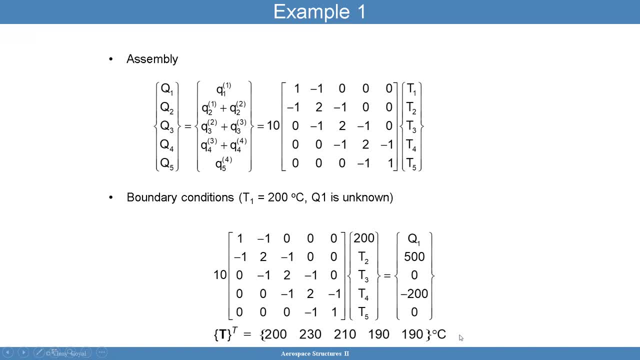 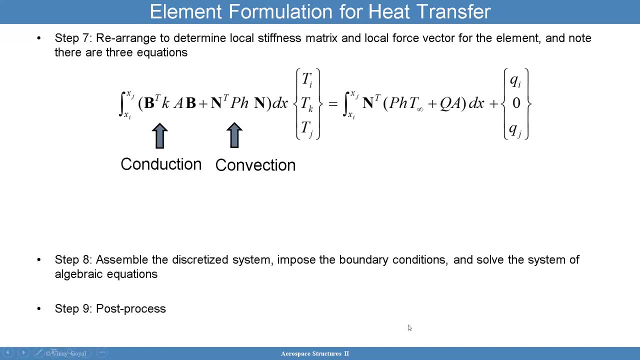 so, for example, i'm taking this problem and i'm going to write this down. so i'm going to take this problem and this problem that's going to be equal to zero. so that means you do that. you get the temperatures across all the nodes in this problem. so listen how we took, look at how we took this. 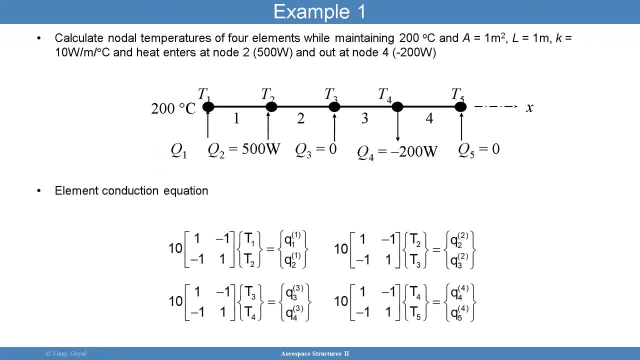 problem this, this, this differential equation, this differential equation, and we solve for temperature by using linear algebra. right, we solve it just using this, and how? i know what the temperature distribution is across the elements. well, i told you that i know that a polynomial approximation is across it. So if I know T1 and T2, then I can determine what the 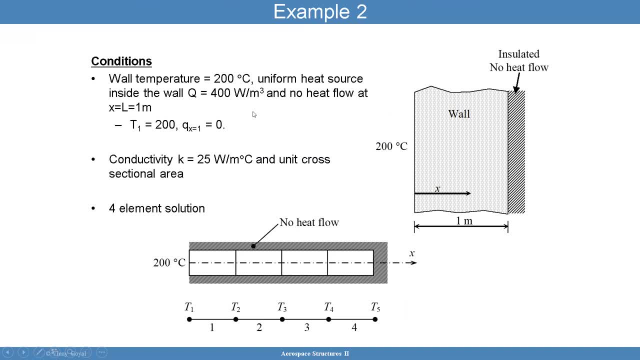 distribution of temperature is across these two elements, two nodes. Here is yet another example of four element solution for a situation where there is no heat flow going out and this wall is infinite in this direction. So in other words, there's no heat flow out here and I'm 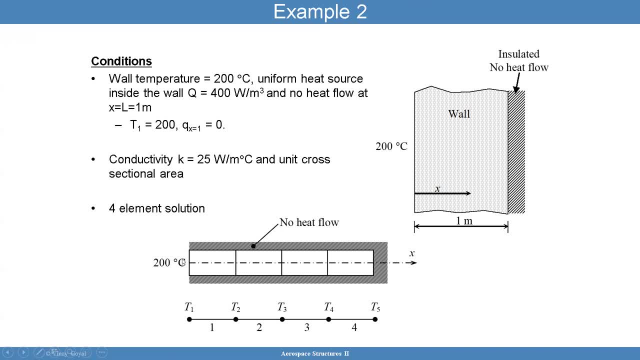 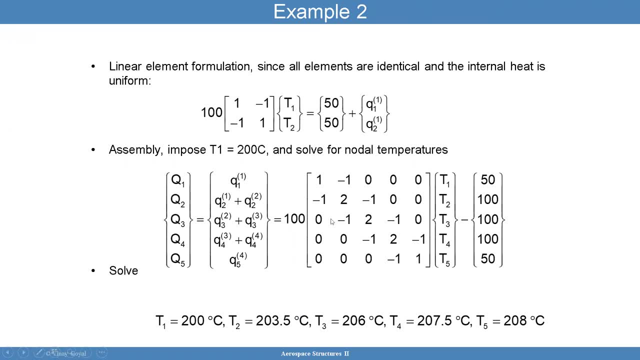 fixing this at 200 degrees F. So the question is: you know what is the temperature distribution? I can divide again the domain into four elements. Same process, I just use the same process, and I can solve for temperature. I can solve for temperature very, very. 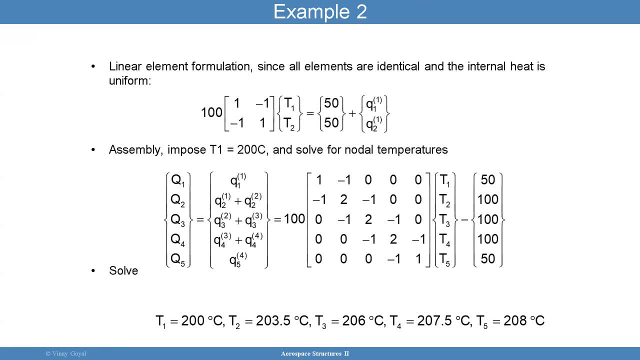 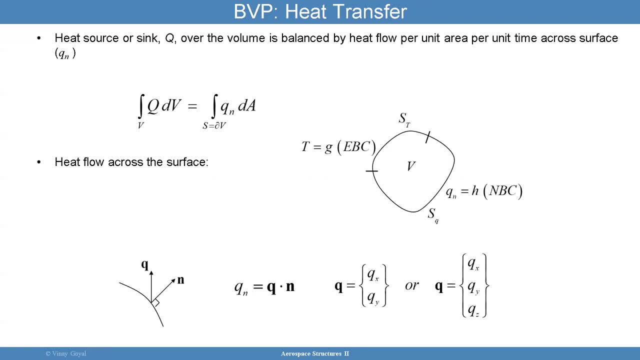 easily and very quickly, And I won't go into the specifics because the whole point of this is to kind of give the big picture perspective. So, in summary, we have the boundary value problem for 2D and 3D. This was for 2D. 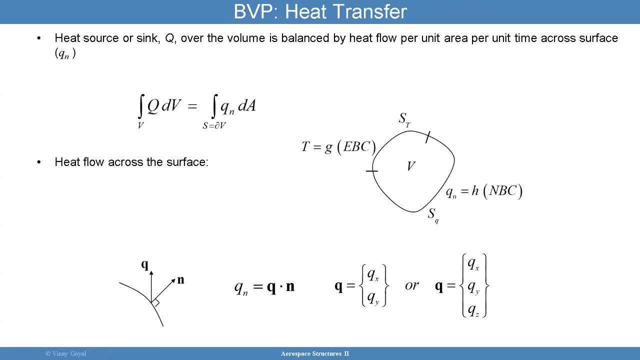 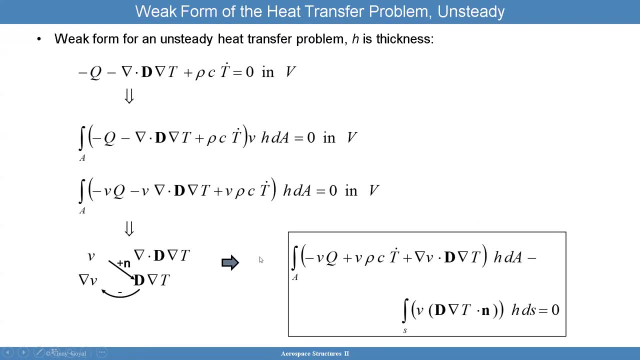 This is for 3D And this is for 2D. Sorry, this is not for 2D, This is for everything, And this applies to 3D and then applies to 2D, which I already covered in extensive detail. Okay, So with that said, 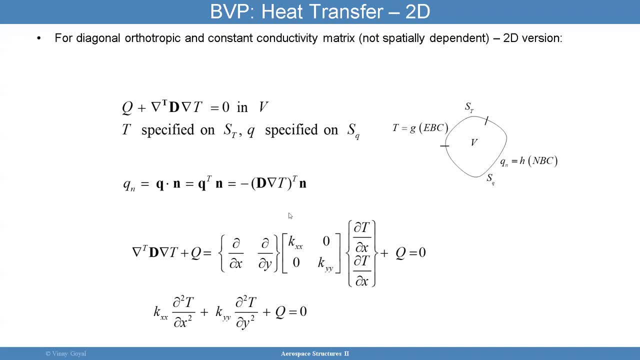 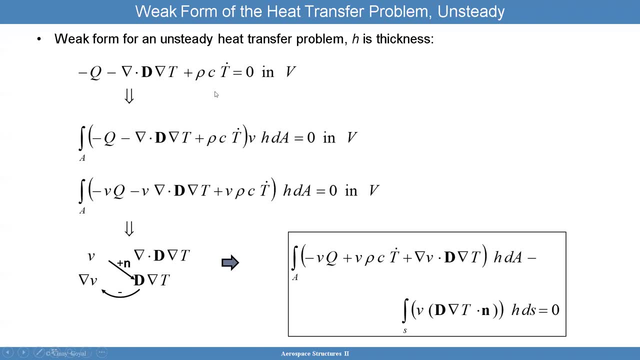 so now let's look at how we will consider a time-dependent problem. So in a time-dependent problem, you're going to have to consider the specific heat of the material, the density, and you have to add this term ddT, dt. So the temperature has a derivative. now 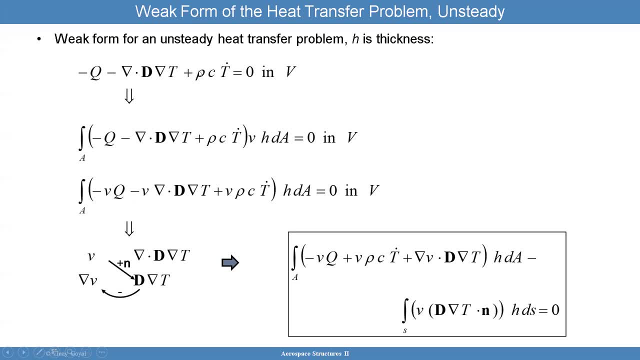 respect to time. And now you have to consider the density and the specific heat of the material. And now this equation now has to be discretized, just like I showed before: Multiply the whole thing by V and integrate by parts, as shown here, as I did before. And once you do that, 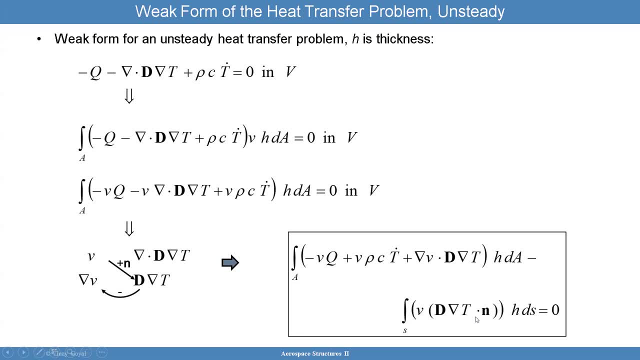 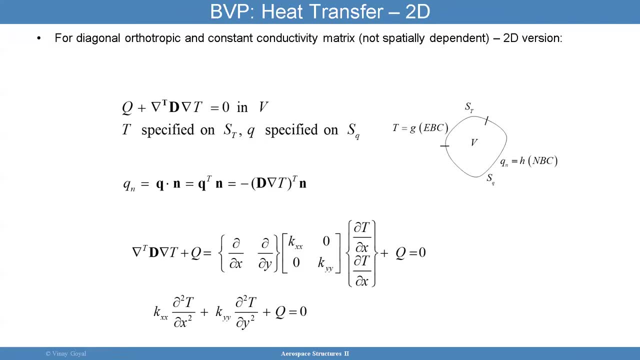 you get this equation, And this equation is now valid for time, but it's not a dependent problem like an unsteady behavior. So before we're looking at a steady state where it's not dependent on time, Here we're looking at how things could evolve over time. 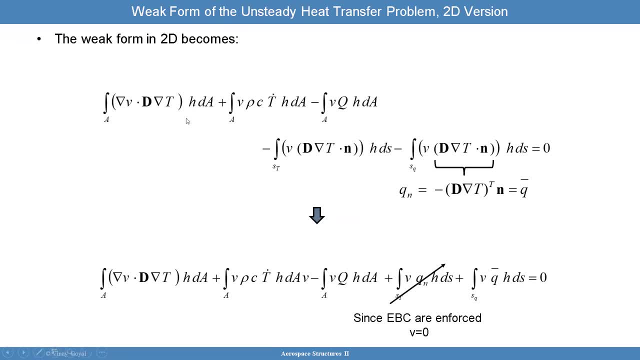 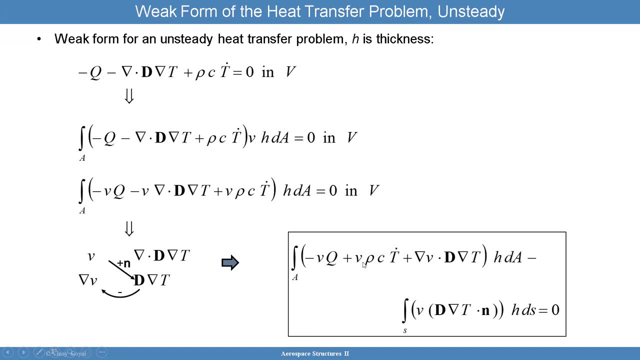 So you can develop now the weak form using the process I discussed before in 2D. This is for 1D. In 1D you get this. I'm sorry, this is not for 1D, This is for 2D. 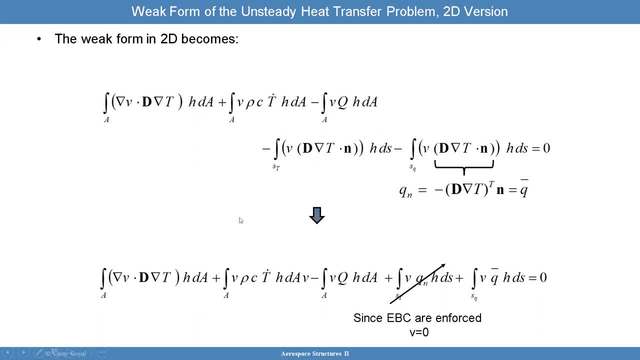 And now this is shown, what the weak form is in 2D, And I'm kind of skipping some of these details because the bottom line is it's the same process as before, but I'm keeping this term. now I have this time-dependent problem. 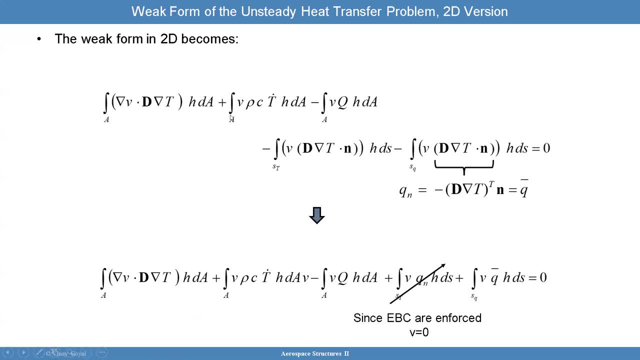 Now if I didn't have, I had a steady state problem. this one goes away, But in our case this stays here and has to be looked at carefully as we move through these derivations. This V shouldn't go here. That's an error. But in general, everything looks pretty good, And we just just you know we're going to have to do this, And we just just you know we're going to have to do this, And we just just you know we're going to have to do this. 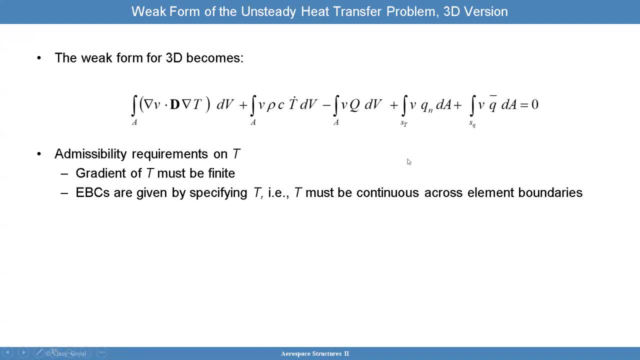 And we just just just you know we're going to have to do this- We just substitute everything we talked about before And the weak form for 3D becomes this one here, And I already have another video in fine elements. 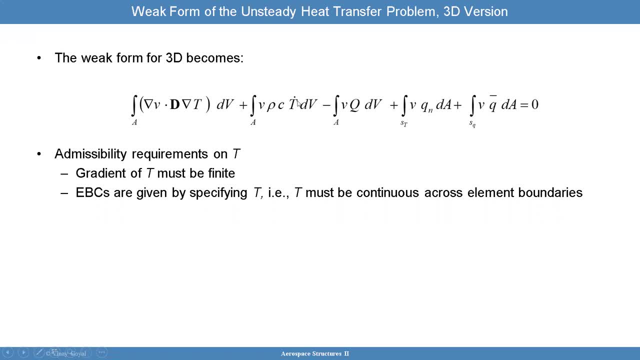 that goes into extensive details on the discretization problems for fine elements. But here we're given a top-level view and not going into extensive details. And again, V is an arbitrary function. We're selecting V2.. And again, V2 is going to be the polynomials. 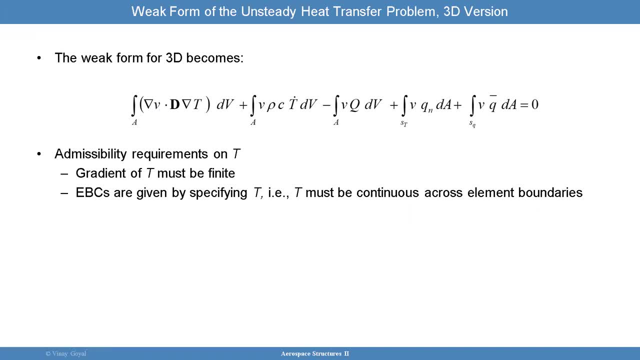 that can solve the problem within a domain, within an element. D is a conductivity matrix and T is what we're looking for. okay, So there you go. And so now what we want to do is discretize the domain, So say, I have a domain of some kind. 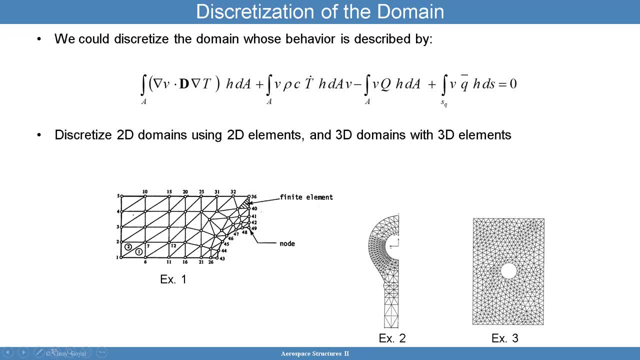 I could discretize it using 2D elements, like you see here, triangular elements and so forth, And we're going to discretize this equation over single element And we're going to discretize this equation over single element And we're going to discretize this equation over single element. 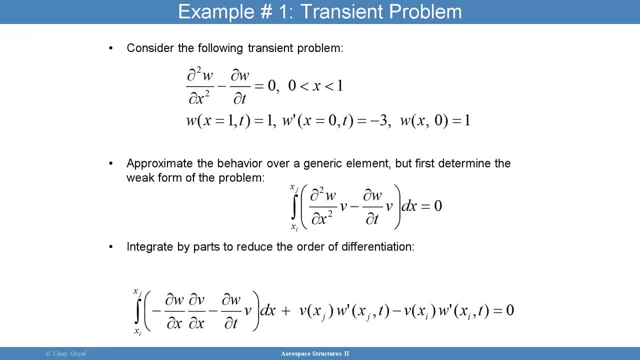 that gets mapped into a standard element. So here's an example of a� onunва problem. You have a, you know, a constant problem of some kind where this is equal to zero, D is equal to zero. I have some initial boundary conditions. 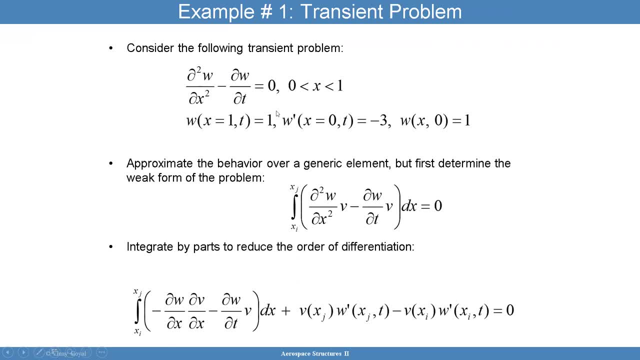 I can approximate the behavior over single element by multiplying this partial differential equation and making it orthogonal to a function, V. So I'm multiplying this by V, basically, And what I'll do is I'll integrate by partial deviation and I turned the variable versus the height of the elevation. 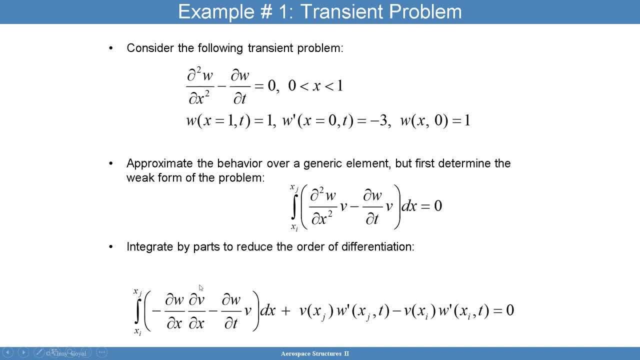 by removing this derivative and transferring over to V for this term, because this term has equal derivatives on V and W. So, as a consequence, I don't have to worry about this term and I'm trying to weaken the continuity requirements. So when I integrate our parts, 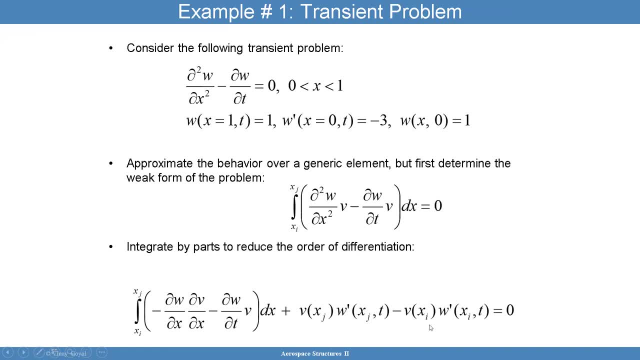 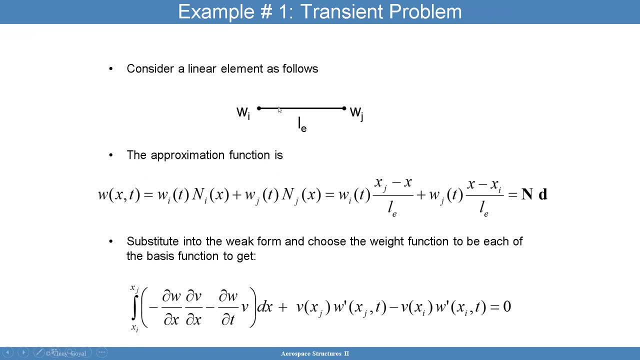 I apologize. I get this here with the following boundary condition, And so if I look at a single element, I can approximate the behavior of how W varies between this point and this point, And I'm going to select this polynomial. It should be linear, because I have only two unknowns. 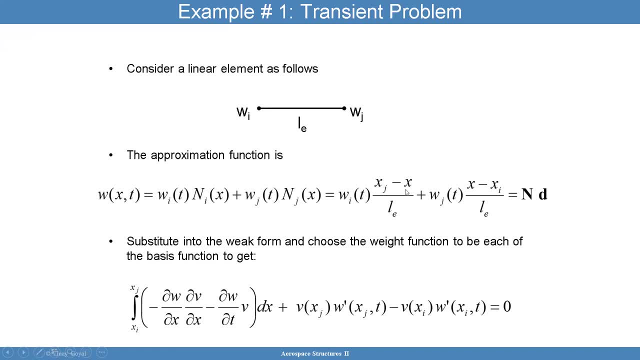 You can see that it works out, because if X is XJ, which is this point here, I get zero, And if X equals X J, then this becomes the length of the element XJ minus XI. LE divided by LE is one. 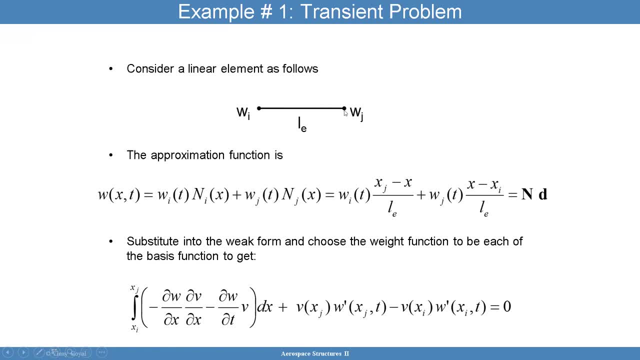 So clearly, W is WJ at X equals XJ, So that works out. You can see that this polynomial works out. You can also see that. now, what I'm doing too is I'm varying the nodal deflection, the nodal values, not deflections. I apologize. 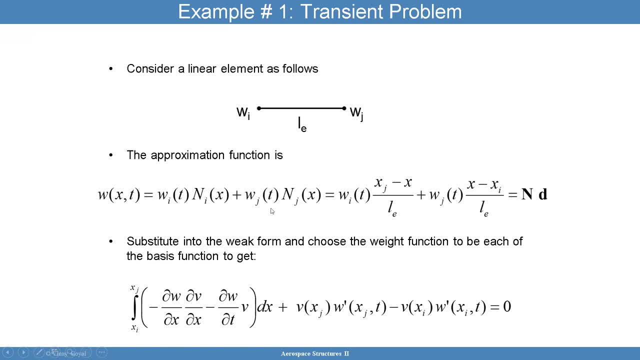 The nodal values. I can vary them over time. You can see that there. So that's now varying over time. Before these were constant. this was not varying over time. Only we had WI and WJ and they're not varying over time. 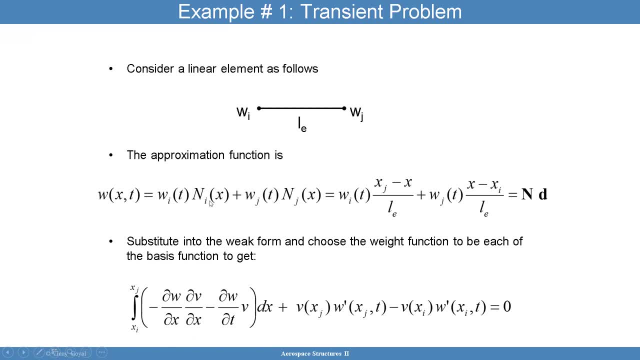 but now they do, And you can see that we're applying separation of variables. here We're separating the time domain from the spatial domain. I can again put this in a matrix where N is a polynomial, here this first polynomial and second polynomial. 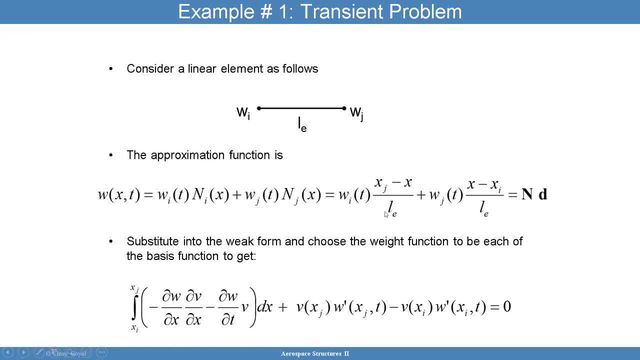 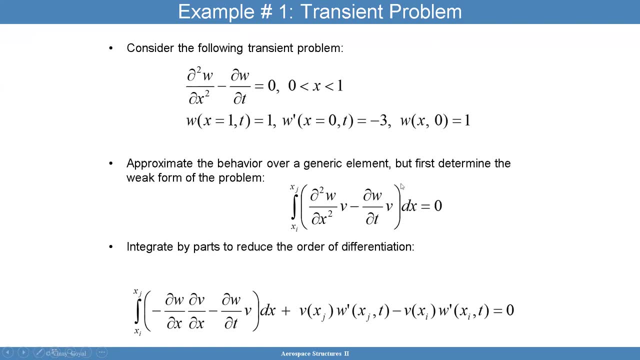 And D bold is made up of these two quantities here. We'll then substitute this equation. So for W we're gonna select N times D, and for V we're gonna substitute N. So that's what I've done for this equation. 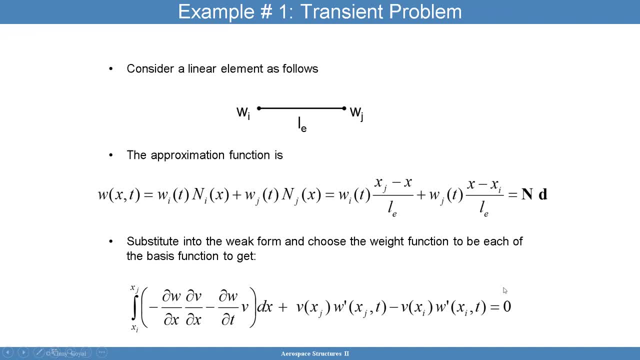 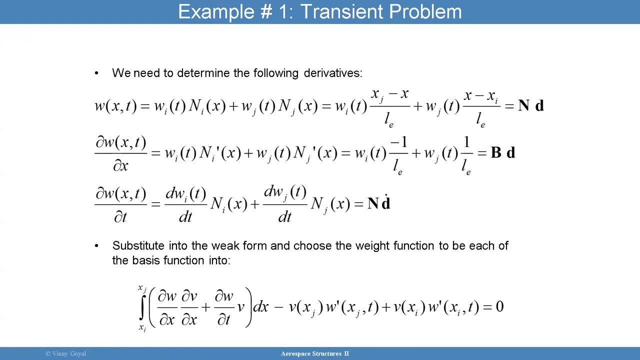 We're gonna take this N times D and just plug it in there and see what happens, And when I do, when you look at all the things that need to be considered in this derivative W is just N bold times D, So that's easy. 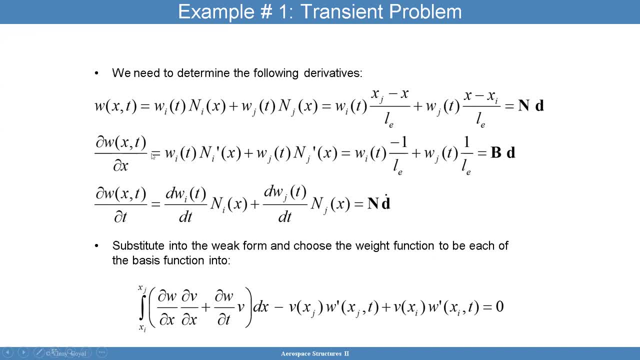 Derivative of W with respect to X needs to be calculated. You can see that here. So when you go through that, this becomes B bold times D And then you have the derivative of W with respect to time. That's easy. That's N bold times D dot. 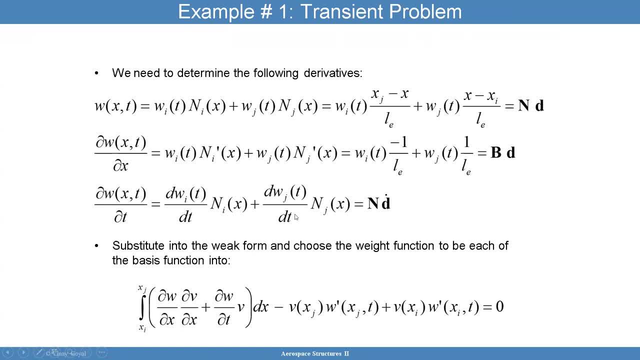 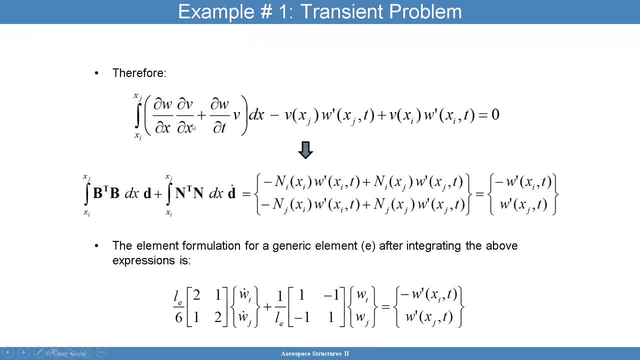 where now these derivatives are the ones that are being looked at, And now I can go ahead and substitute it, And when I do so, and I invite you to do it at home, so you can see that I can go from here to here- 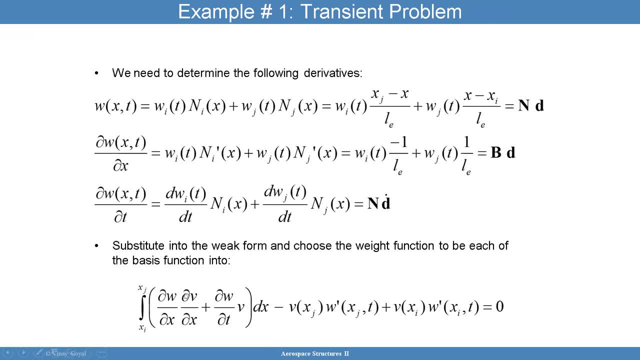 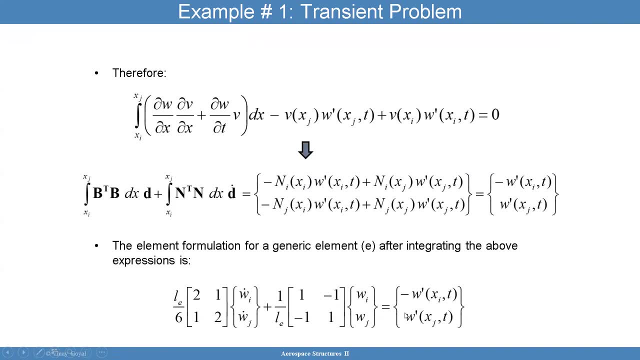 And any group, any group that derives it, any group that derives it going from here, from this step, if you can derive, going from that step to this step, I'll give you 50 points towards, or, if you're able to do it, 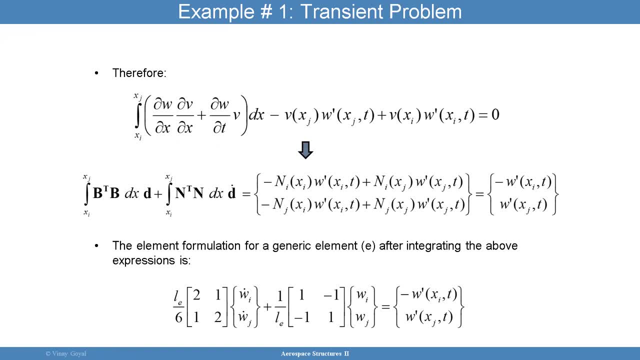 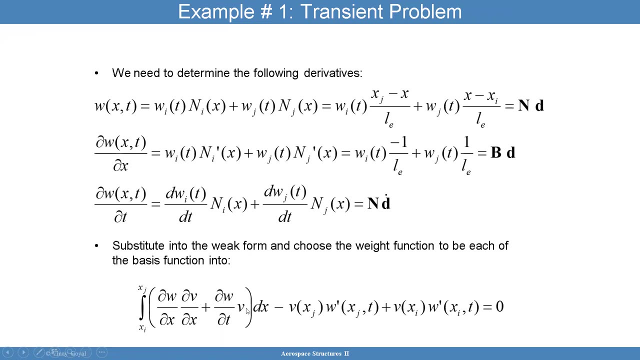 we can come up with an agreement of extra points that can be applied for issues you're encountering, But the point I want to make is that this is very easy, because all I've done is substitution, just substituting these guys in here, And for V I'm going to substitute N, transpose. 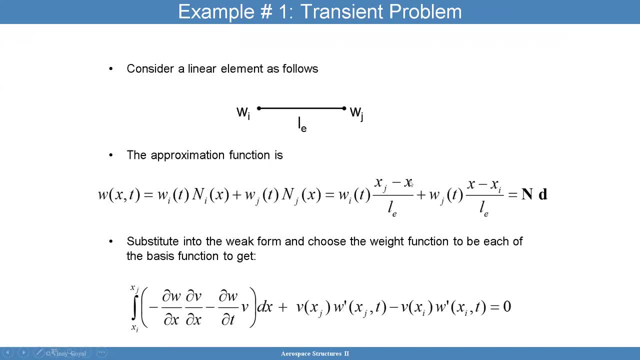 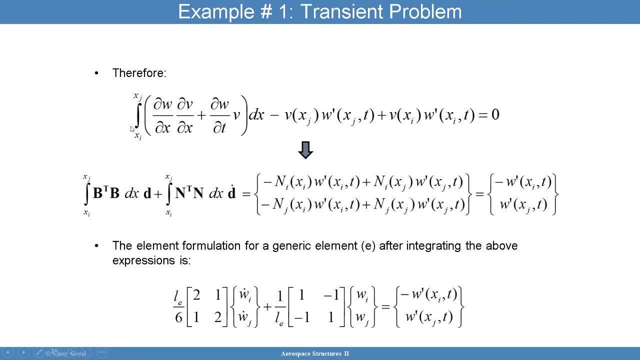 So when I do that and I solve for this, this N1, Ni and Nj, when I'm able to substitute to that and integrate it over this integral, what I actually get are just basically numbers. This is what I get. 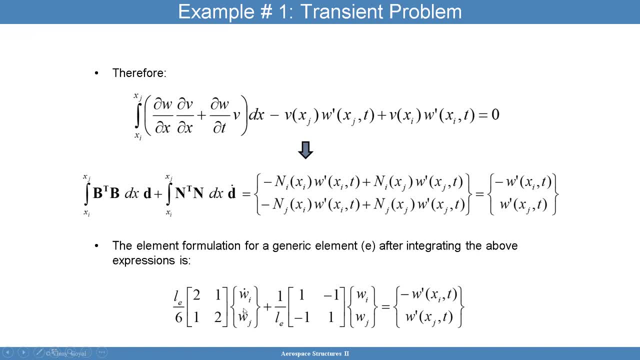 It's very simple For a single element. it looks very simple. Now what I have is- I think you've seen before how to solve time-dependent problems numerically, but this is the equation that we're looking at now. Very simple now. 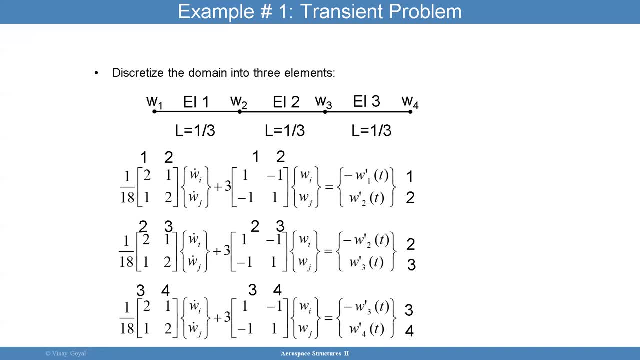 Looks very simple for a single element. But now I have to look at, say I want to discretize the domain into three elements. I have this domain. All I have to use this equation three times: LE is one third. You can see here: LE is one third. 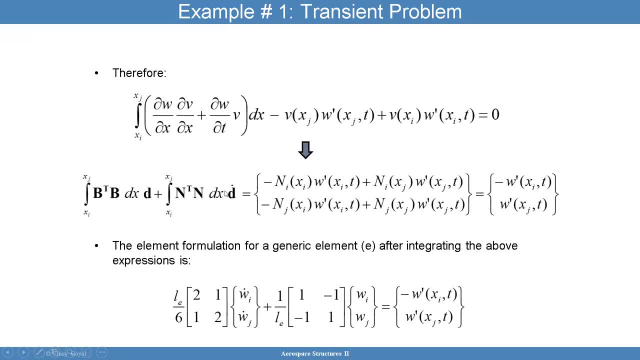 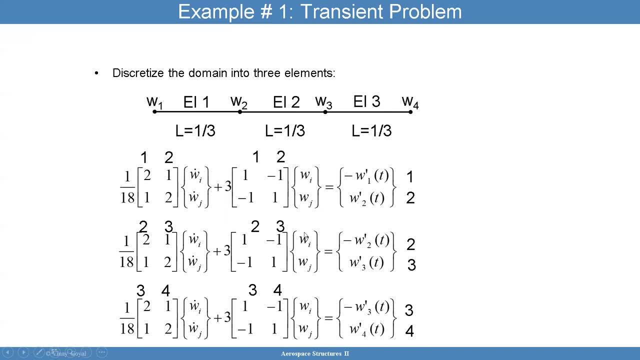 so I get one over 18 and that's three. This LE is one third, so I get three there And yeah, that's element number one. element number two, element number three. Now notice that if every element is the same size, 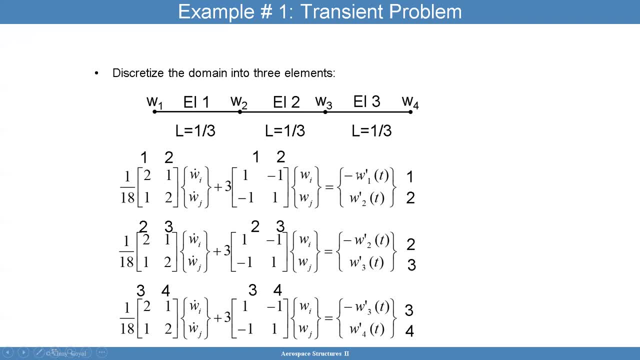 every single of these are the same. Nothing changes, which is amazing, Because that's cool. I don't have to keep doing these calculations over and over and over. if the element size is the same, I can then assemble these equations into a mega equation. 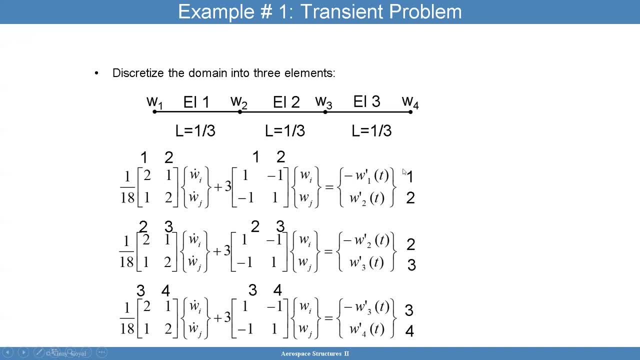 because you can see here that I have this for node one and node two, but element two is node two and node three, and element three is node three and four. So there is a way to bring everything together, And when I do that I get this four by four matrix. 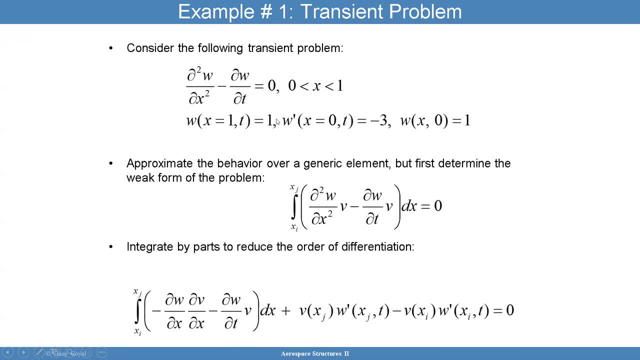 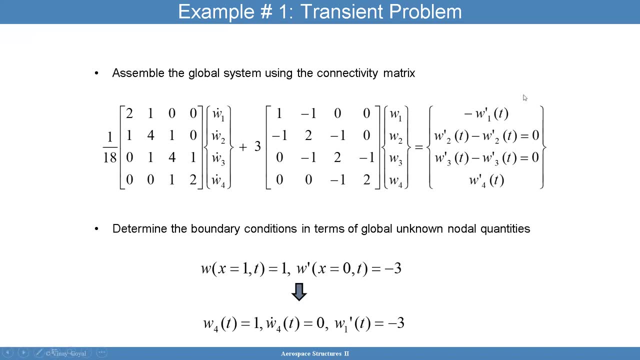 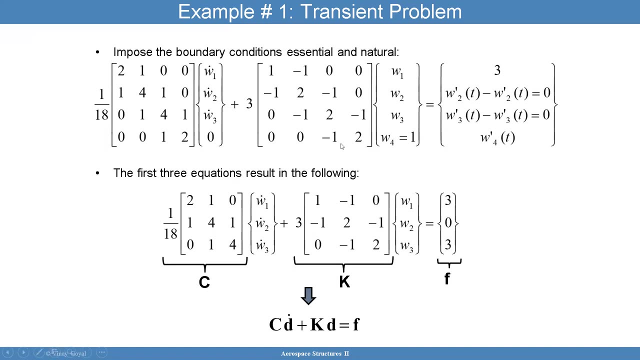 I apply the boundary conditions. I know them. they're given to us in the initial statement, They're given to us here: W at x equals one is one, for example. So I can just substitute everything here and now. I can, then basically yeah. 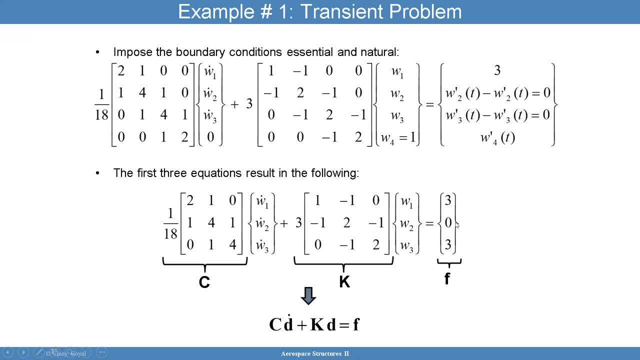 So I basically simplify the equation into this: right W one, w w three are the unknowns, And now I have to do now? Now, all I have to do is do a solution to this which is using finite difference. So if I call this C bold, this K bold and this F bold, 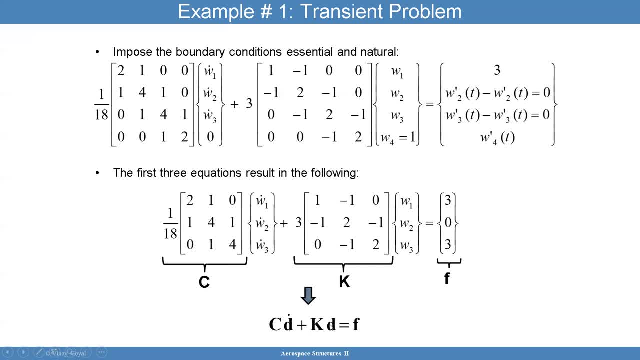 and I put this into D dot and I put this into D. So now that I have these equations, these three equations, I'm ready to solve for W1, W2, W3.. And to do that we're going to use an idea called finite difference. 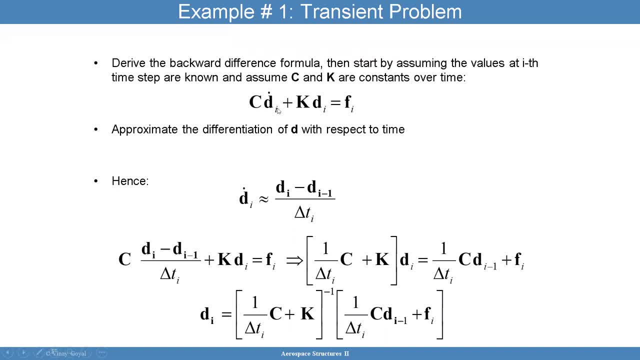 And what we plan to do is then take this as a time derivative- D, D, D, T- And so I'm going to approximate the solution as the solution in the present minus the solution in the past, divided by the time step. when this occurs. 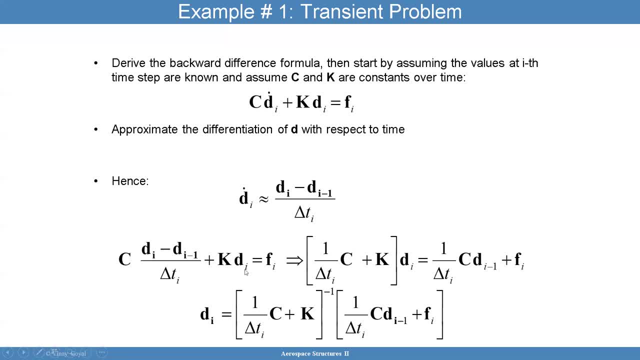 And so I plug that into this D dot and I have this D I. I'll leave it alone. I can now solve for D? I, So I basically get D I equals all this. So, in other words, if I know the solution in the past, 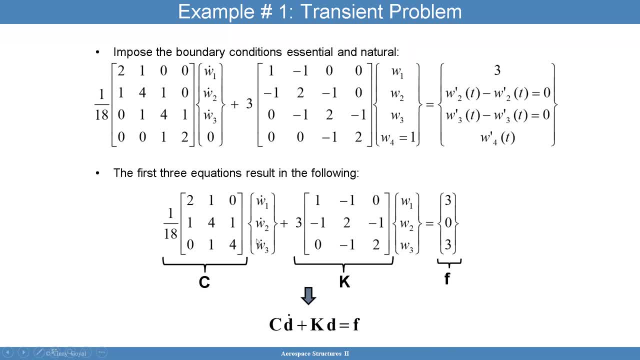 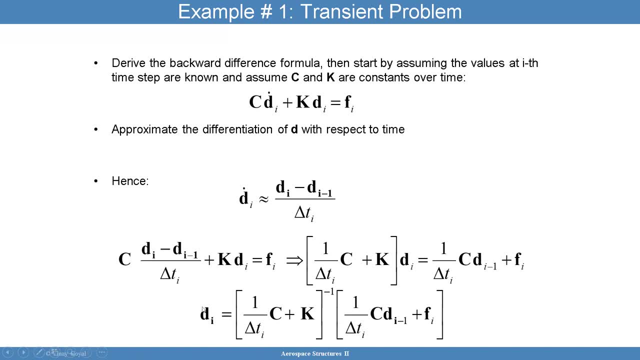 if I know the solution in the past for W and I know C, I know K, these are all numbers- then all I have to do is plug everything in and, given the time step, I can calculate the values of D presently. 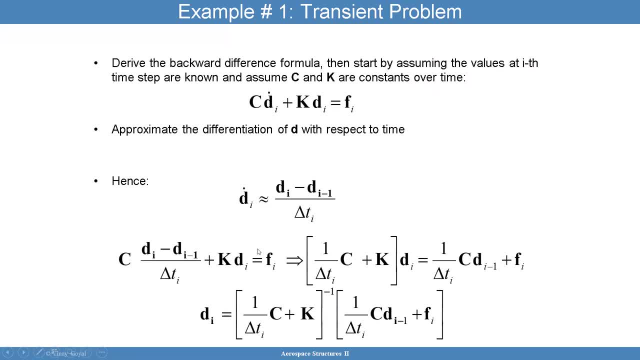 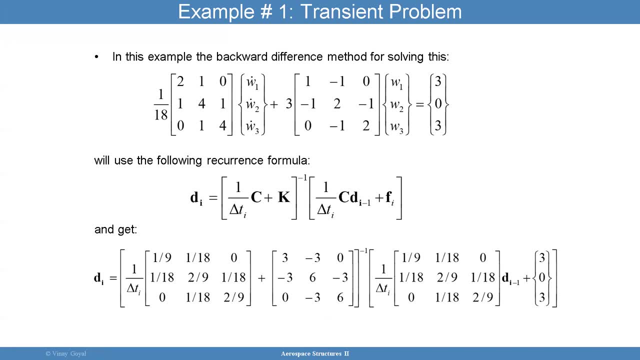 meaning. I know W as a function of time. So that's the idea here- is to march the solution forward once I know the initial conditions. And so here I don't want to go into the extensive details, but you can see, here the equation is given. 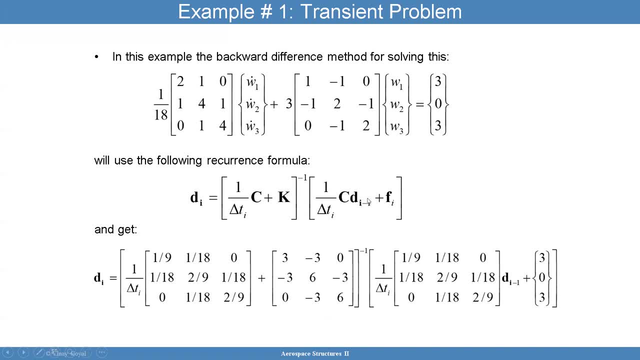 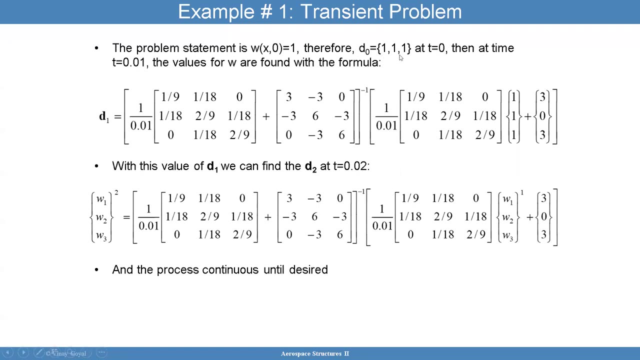 You can use the recurrence formula. Once you know the initial state, the initial value of W, you can then time march the solution to get the future solution And you can see here what's done. here, Say, you start with the initial value of 1, 1, 1 at time equals 0.. 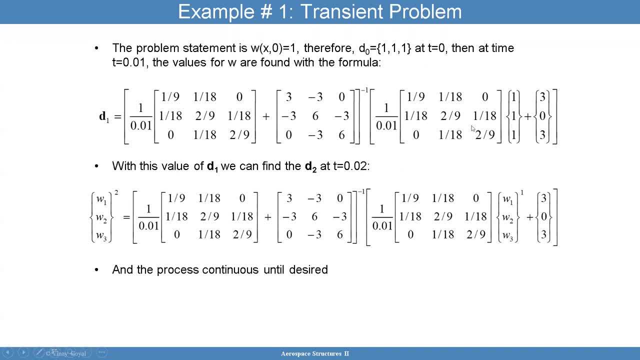 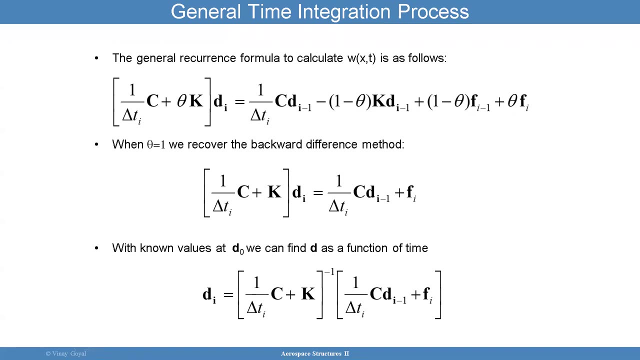 You can see how quickly. these are all numbers that basically end up being very simple And so, as a function of time, you can now get the evolution of W. as a function of time, There's more advanced ways to use the recurrence formula, but in general the backward difference method works really well. 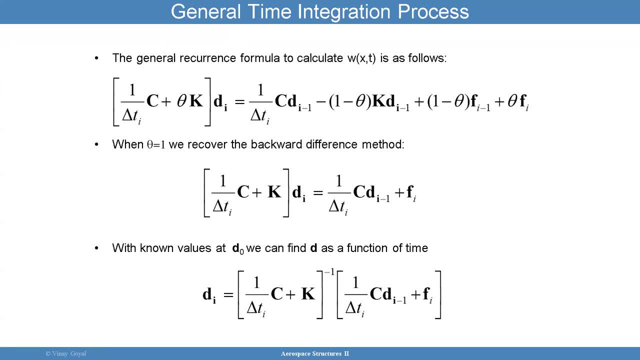 And I don't want to bog down this particular lecture, because this lecture again is not about the theory of finite elements, although I'm covering some aspects very top level, so that you know how that works. So there are various methods. 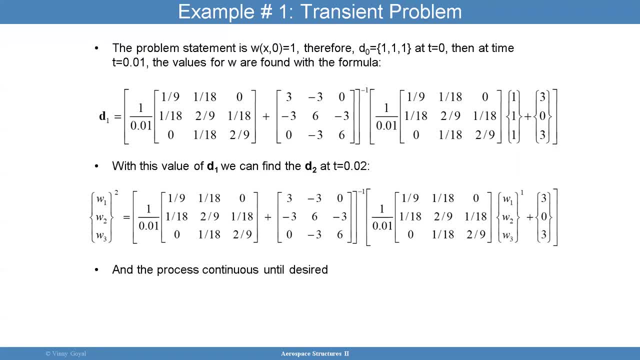 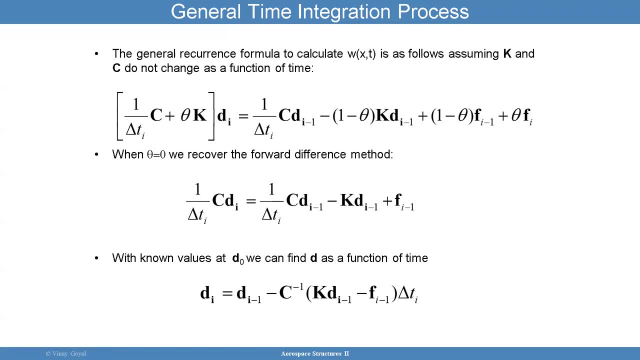 The method I showed you is called the backward difference method. There's a forward difference method, And so this equation here allows you to look at various formulas like that. So this is your forward difference method in this case. And then here- and I'm moving quickly- 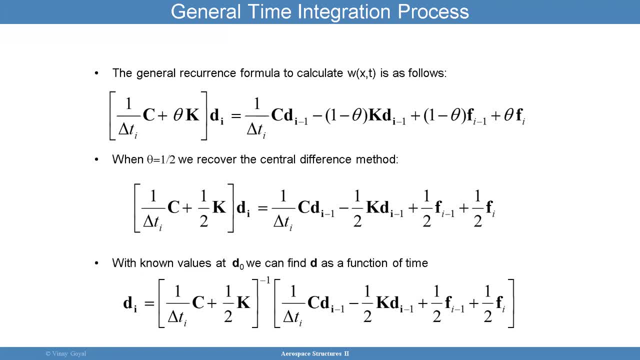 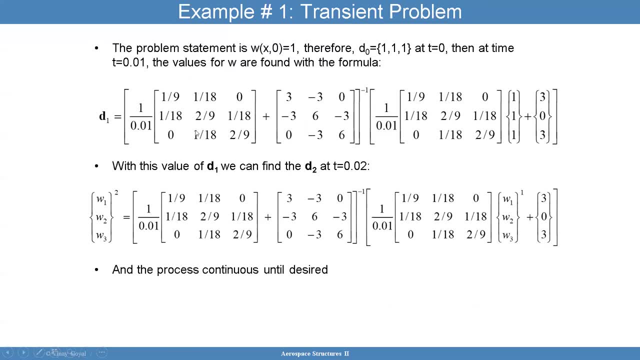 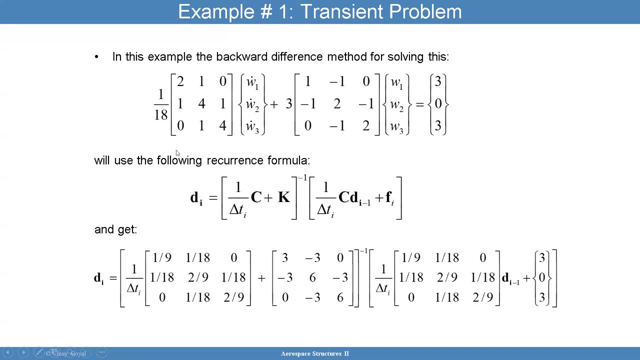 You can pause the video and look at it later. We can look at more advanced techniques. Like if I put theta equals 1 half in this formula at the top, that I gave here this one here 1 half, So for theta equals 1, you recover exactly what I showed you here in the previous. 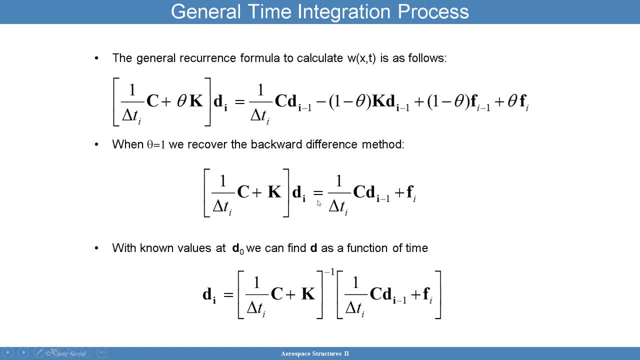 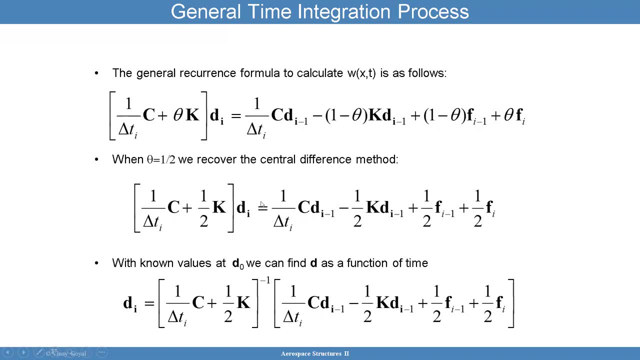 this equation, that's a backward difference. If you put theta equals 0, you recover the forward difference method, which I'm not covering here, And if you put theta equals 1, half, you recover something called a central difference method, And you can then time-march the solution just like I explained. nothing too different. 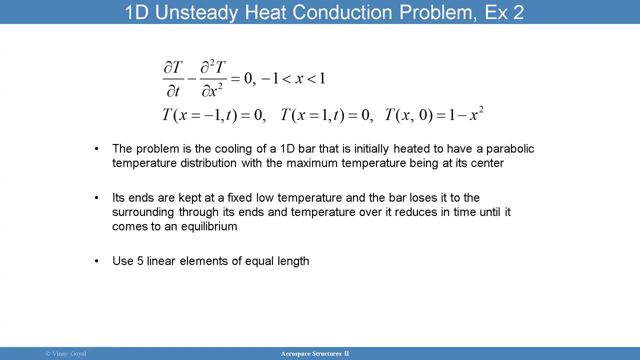 So if we look at an unsteady heat conduction problem, we can look at that And say I have this problem with these binder conditions And the problem is really looking at cooling of a 1D bar that's initially heated to have a parabolic distribution. 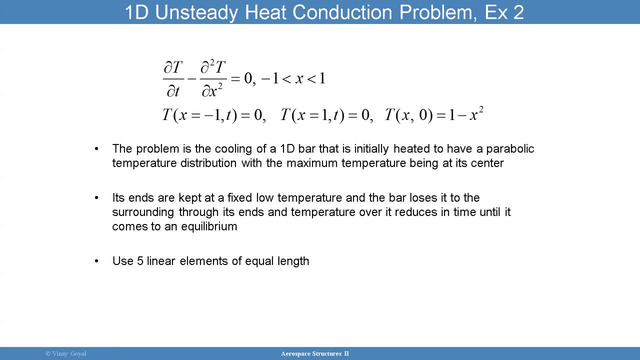 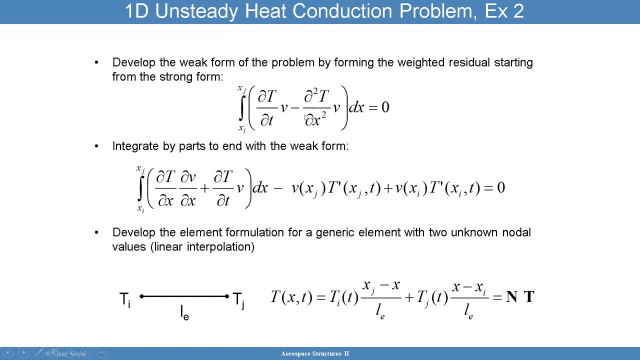 with a maximum temperature being at the center. So we can look at that for five elements And again use the same formulas that we just discussed. Multiply this by V. So take this, multiply it by V, integrate it by parts and you will get this. 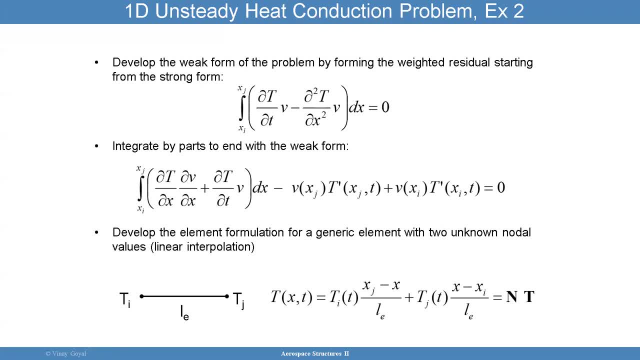 And if you don't remember how to integrate parts, look it up in a calculus book, because it's explained there, or use the methods I described today. So you get this equation. And now I approximate a domain using a linear function, simple linear function. 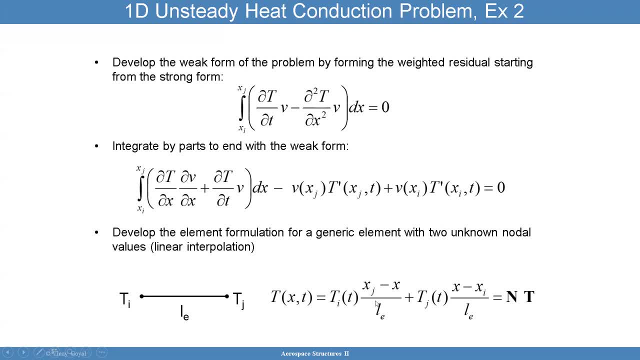 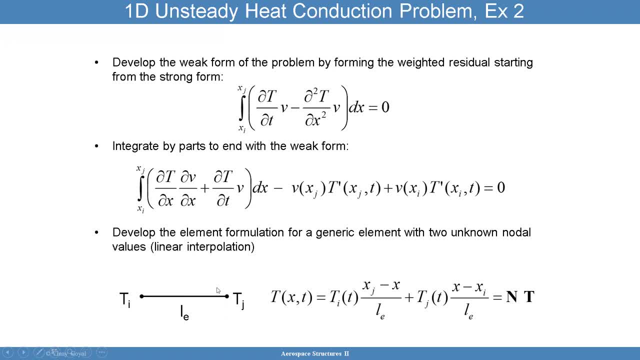 If I put Xi here, I get 0.. If I put Xi here, I get 0.. If I put Xi here, I get 0.. So I do recover back that value. If I put X equals Xj, this goes away. 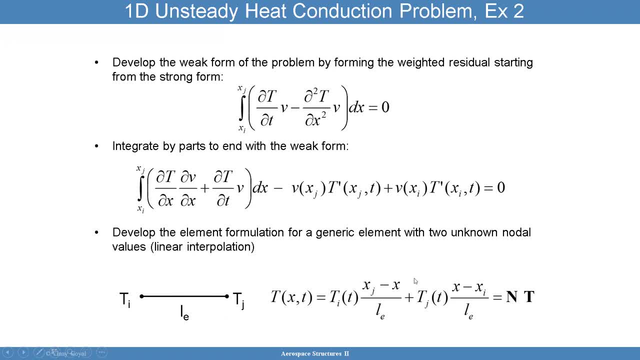 This becomes 1. And so I recover that this temperature becomes Tj, which is that point, And anywhere in between X can be anywhere between Xi and Xj, And this is going to be the temperature in between. It's going to be a combination of something here plus something here. 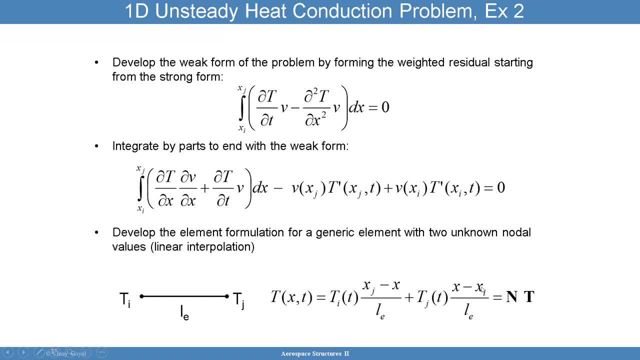 I put this into T and these interpolation functions into N- This point here- And so I'm going to have a polynomial approximation, And then I'm ready now to again to execute. I can find this, I can find this, I can find this and plug it in. 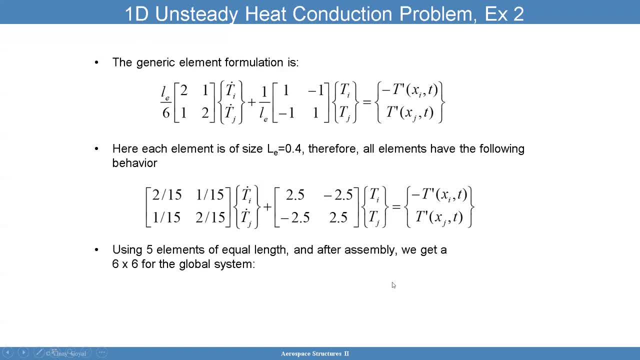 So that's what I've done here: plug it into the equation And now evaluate the integral And you get this for a single element. And since each element in our case is of size 0.4, and I stated it here- 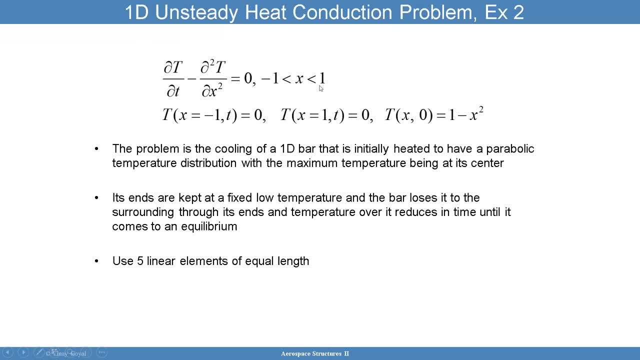 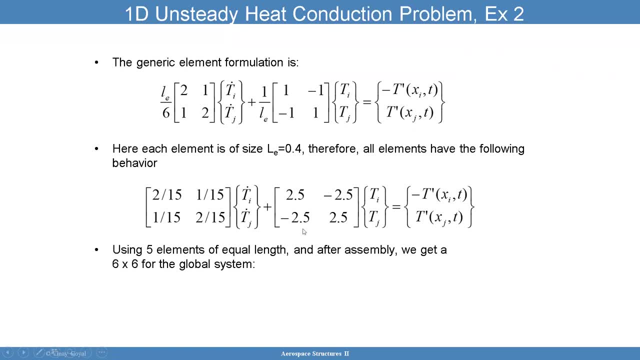 because I said it was 5 elements going from minus 1 to 1.. So clearly the least I can say is minus 1 to 1.. So I have to say that I did a double multiplication. length of the element has to be 0.4.. So L is 0.4.. I plug it in and I get this as which is true for 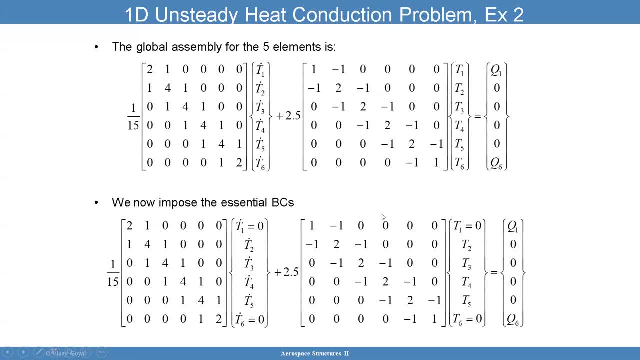 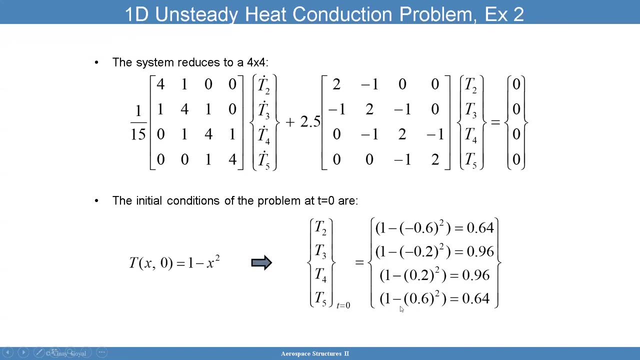 every element, this, this equation. here I can then assemble it, because the nodes are shared across element boundaries And when I, when I impose the boundary conditions essential, the boundary conditions which are the temperatures, I get this, And now I can reduce the. 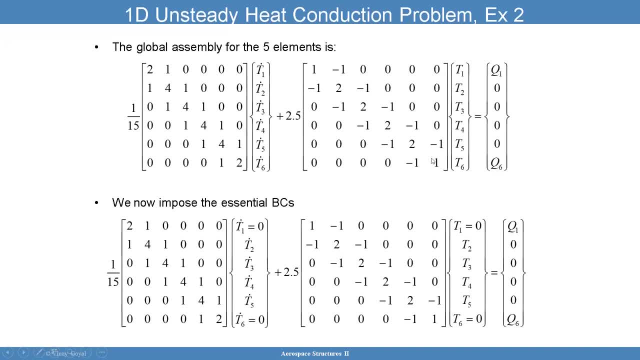 system to what matters, what I want to solve for, Because I already know this: T1 and T6, and T1 and T6. So all I don't know is T1 through T5. So now I'm ready to apply the idea of the forward or 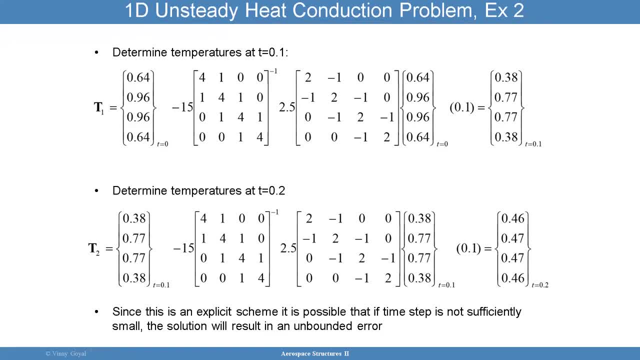 backward difference, whatever appetizes you to look at. Yeah, So you can then time march the solution. T equals 0.1.. I get a certain temperature And then I plug that in again And I get a new temperature. at time equals 0.2, and so forth. So I can time march the. 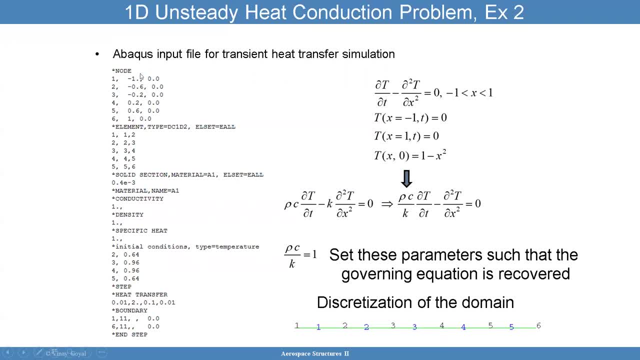 solution. This was done in abacus. You can see here the nodal values are provided, The elements are provided. That's the element type within abacus. That's a one-dimensional heat conduction element. The two means that it's a two-noded, two-noded element. So very. 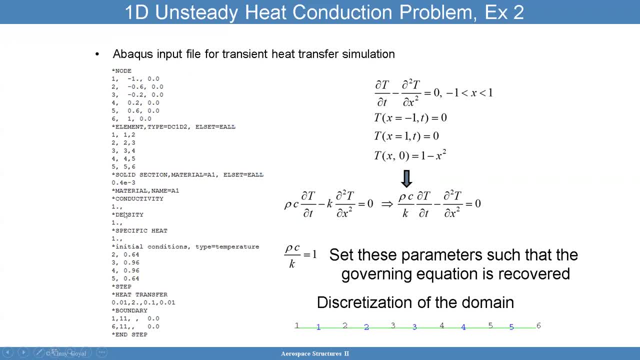 simple. Here's aluminum material, So the conductivity of the aluminum is provided, Specific heat and so forth. So all that is provided here And the step here what it does. it basically time marches the solution and solves it. All this you can do through a GUI, So it's not. 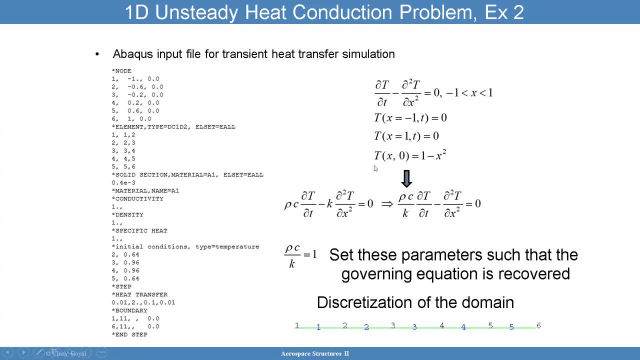 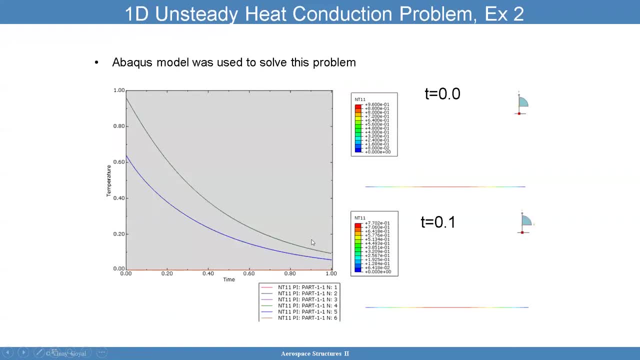 really important to really learn these intricacies, But in general, we can then solve this equation using abacus, Where the final end software and not to show off, but the solution matches what I did by hand, And this is the temperature: at time equals 0, at time equals 0.1 and so forth. 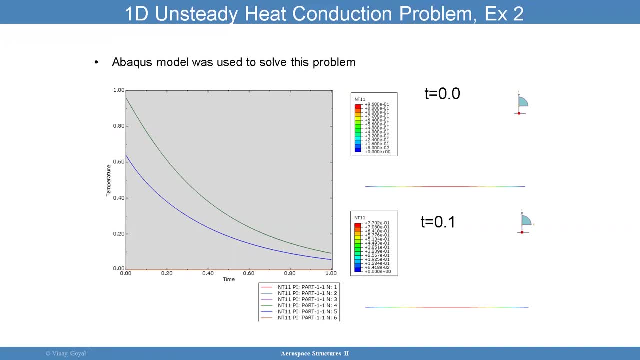 So it's temperature is varying over time. You can see that here Temperature is varying over time And the temperature here is varying over time For node number 1 and 2, 3,, 4,, 5, 6.. 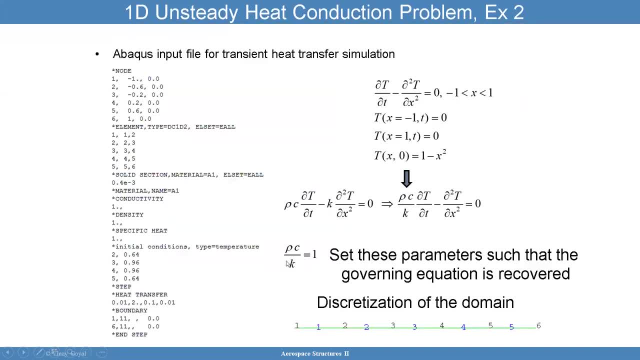 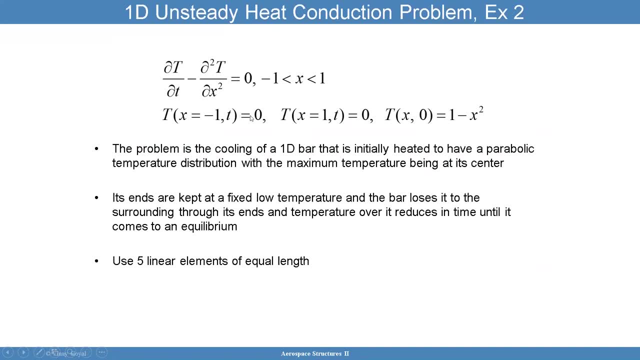 shown here that the temperature is dropping over time and you can check to see if it makes sense. right, you have the boundary conditions is saying that the temperature forever is zero at x equals minus one. the temperature is forever equals zero at x equals one. so clearly we're fixing those. 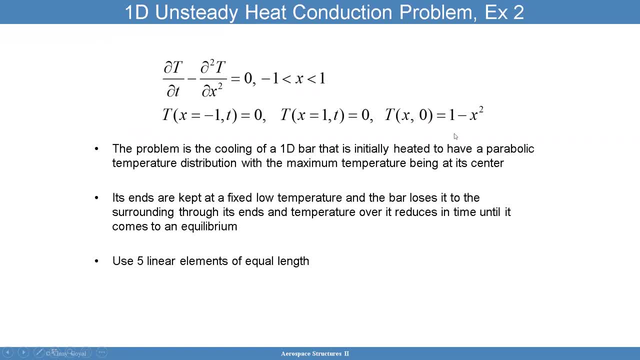 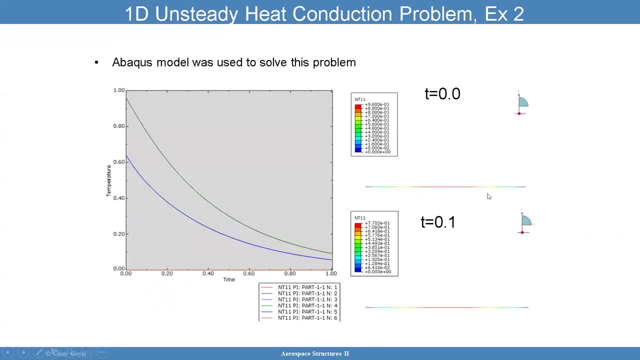 temperatures at zero, while in between is parabolic distribution temperature. so it makes sense that the temperature is dropping over time. you can see that the temperature here is parabolic. it starts zero and increases and then drops off, and that's clearly parabolic and over time. that's very 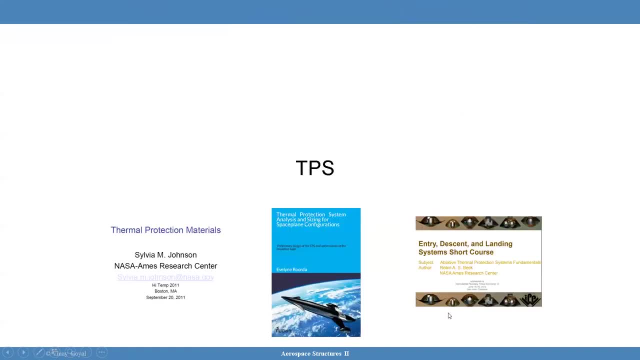 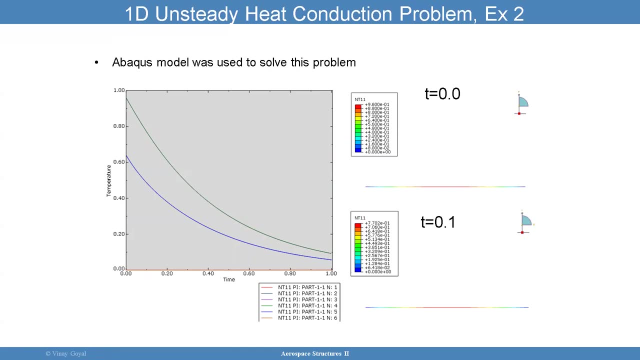 changing over time as well. so very cool. so, with that said, i'm going to move into thermal protection system. this is a basic course in heat transfer that i'm going to now take, and i covered five elements. so i covered two topics into one: heat transfer as a by itself finite elements by itself. 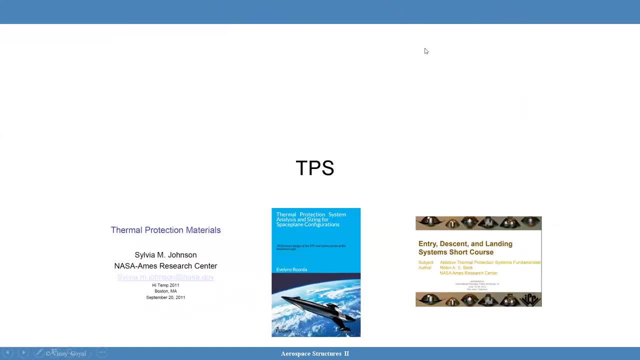 and now i'm going to cover thermal protection system. so you can. you can see that the temperature is dropping over time and then drops off and that's clearly parabolic. you can get an idea of where that is used. so, thermal protection systems, i'm borrowing materials. 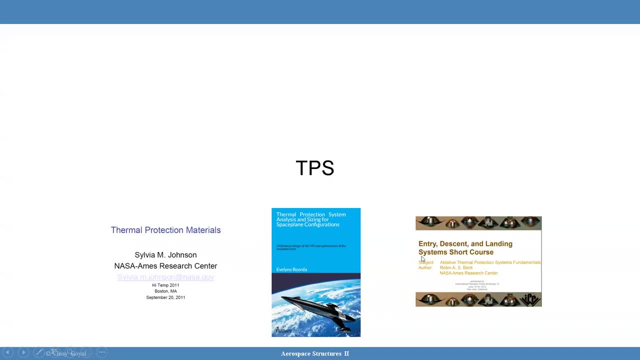 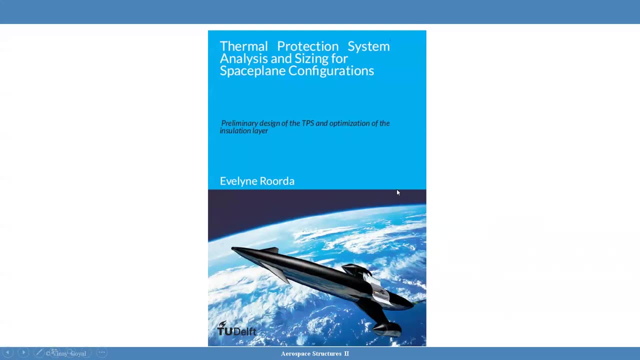 from three different sources. all these materials can be found through online sources and i recommend you download them and look at them carefully. i think it's worth it. this is a very good document that talks about thermal protection systems, analysis and sizing for space plane configurations, and talks about the preliminary design of the tps and the optimization. 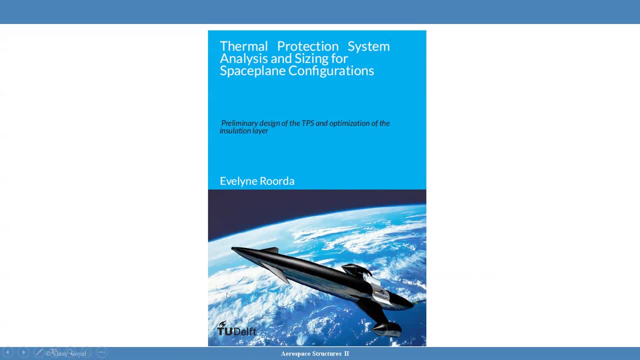 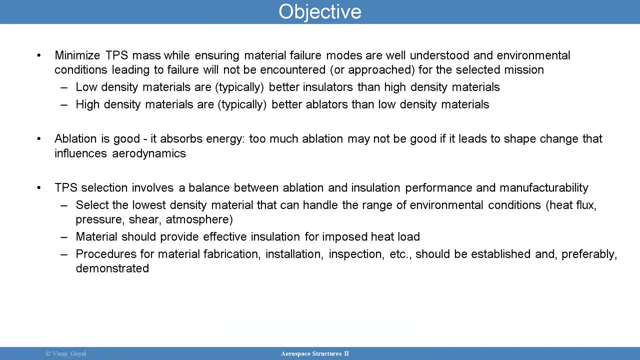 of the insulation layer and this is written by the deft university over there and it's a great document. i recommend you look at it. the objective is to minimize thermal thermal protection system mass while ensuring that the material failure modes are well understood and the environmental conditions leading to failure will not be encountered. for the selection selected. 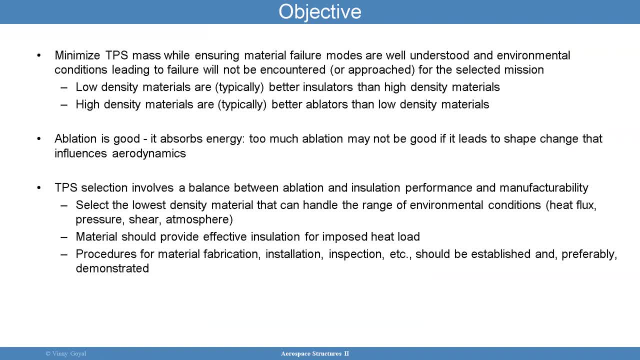 mission. so what you want to do is you want to use low density materials, which tend to be better insulators than high density materials. you want to use high density materials- that are who are, which are better ablators than low density material. ablation is good if you're losing material is good because that's absorbing energy too much. ablation may not. 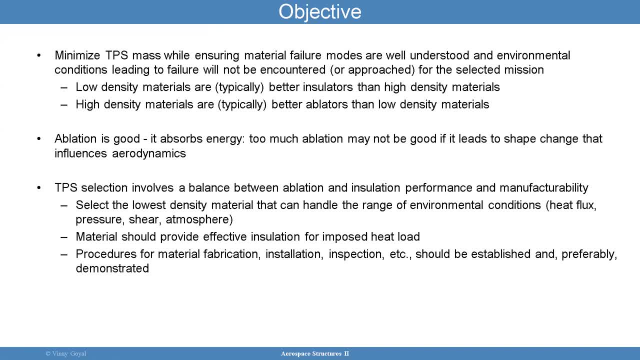 be good because it can change the shape of the structure and influence aerodynamics. secondly, if you have too much ablation and the material is getting lost to the point that you could have a structural failure, thermal protection systems installation involves a balance between looking at good ablation amount, looking at insulation, 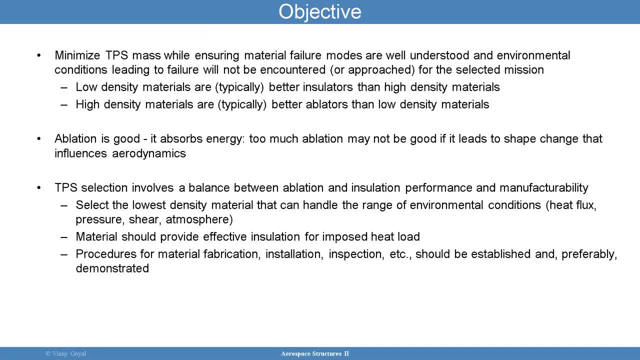 and in within that we want to look at performance and manufacturability. we want to select the lowest density material that can handle the range of environmental conditions: heat, flux, pressure, shear and atmosphere. the material has to provide effective insulation for the imposed heat and procedures for material fabrication. installation inspection should be established. 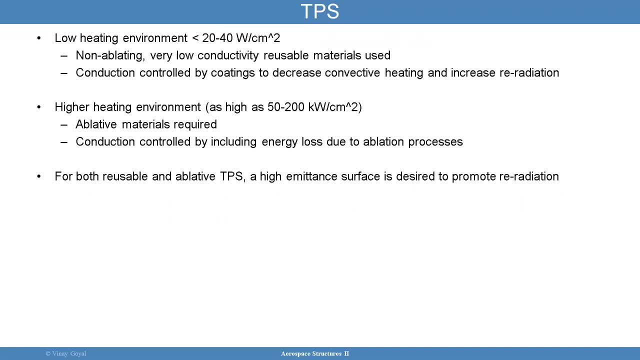 and preferably demonstrated. very important consideration for low heating environments, less than 20 to 40 watts per centimeter squared. we're looking at non-ablating, very low conductivity. you can even look at reusable materials. you can also look at conduction control by coatings to 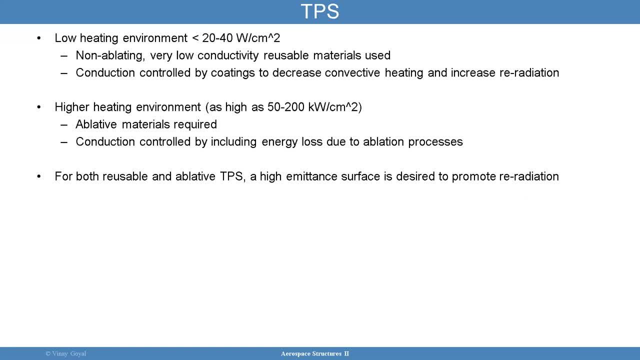 decrease convective heating and increase re-radiation. you also can look at situation where you have higher heating environments, as high as 50 to 200 degrees celsius, and you can also look at situation where you have higher heating environments, as high as 50 to 200 kilowatts per centimeter. 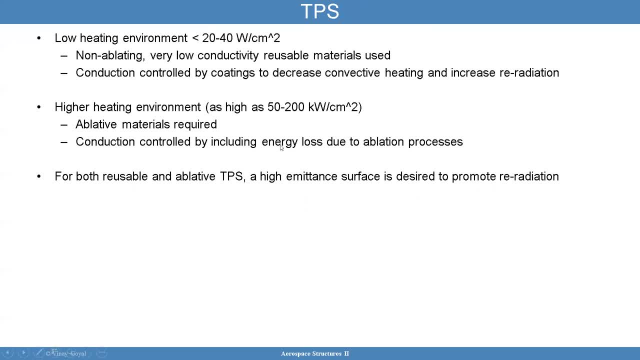 whereas in those cases- i'm looking at ablative materials, which are really required- conduction is controlled by including energy loss due to the ablation process and that's important, you know, you're, you're- you're basically controlling the heat by ablation, actually for both reusable and 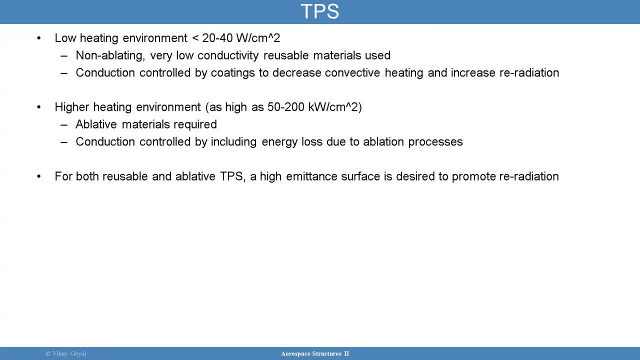 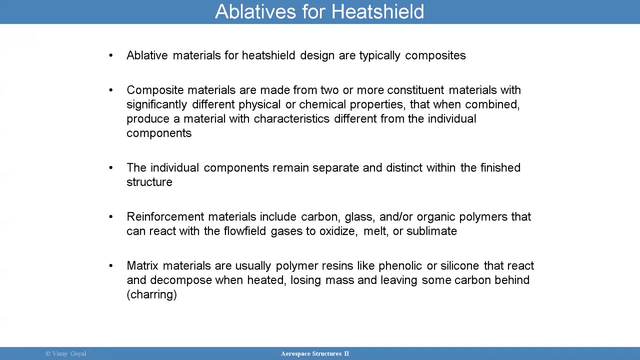 ablative tps, a high emitting surface is desired to promote re-radiation. in other words, you want to have a surface that can emit really well and you you can do that, and that way you can also have heat being removed from the system. ablative materials for heat shield designs are typically composites. composite materials are: 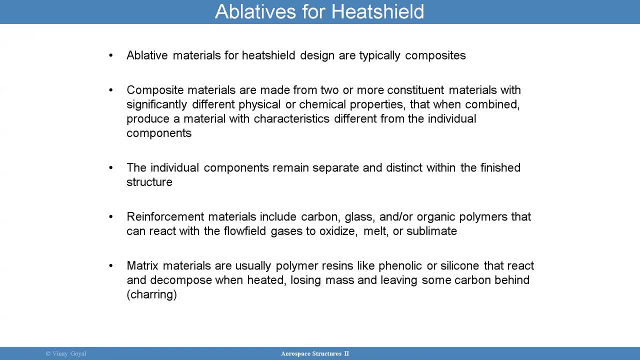 typically made of two or more constituent materials with significant different physical or chemical properties that, when combined, produce a material with characteristics different from the individual components. the individual components remain separate and distinct. we can define a structure, and a lot of the reinforcement materials you may encounter are going to be like. 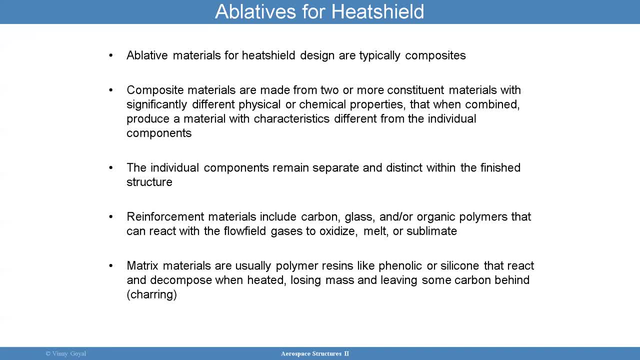 carbon, glass and or organic polymers that can react with the flow of fuel gases to oxidize, melt or sublimate. the matrix materials are going to be typically resins such as phenolics, silicon and those react and decompose when heated and it will lose mass in some cases and expel some gas. 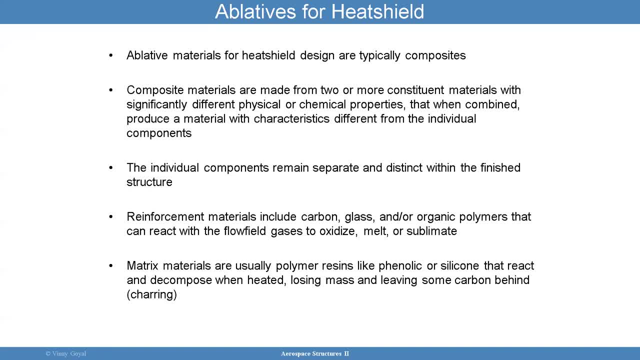 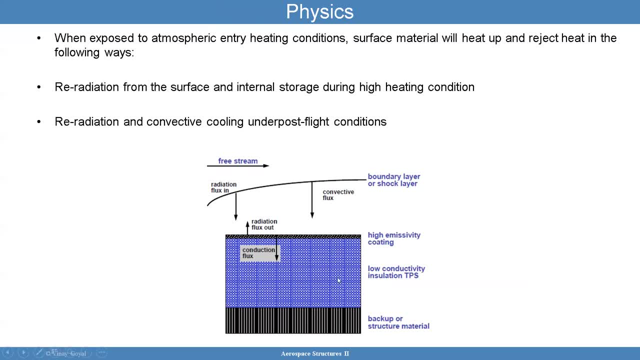 you're also going to have carbon behind being left, which is the charring process. just to show you a little bit more, if you have a structure that's flying in the air, and this structure has a backup structure. so i'm looking at a cross section, by the way, and this is the outside. 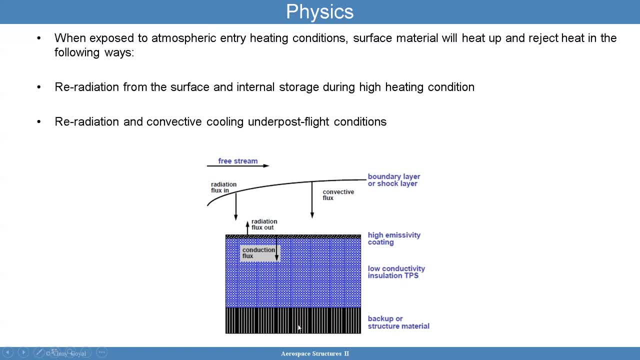 air, so free stream. and this is the backup structure and this is the insulation material, so the blue and whatever you see here. so the point i want to make sure is that you understand that the structure is flying on the air at high speed, say, for example, and when exposed to atmospheric 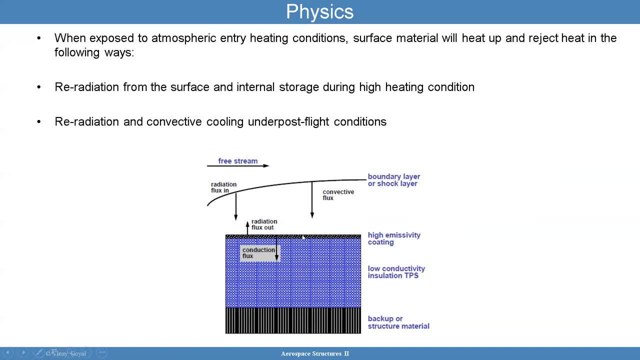 entry conditions. the surface here is going to heat up and the heat is going to get rejected in two ways. you have re-radiation from the surface out- okay, and some of that will go back in through conduction. that makes sense. you also have convection flux going in- okay, and if you have the 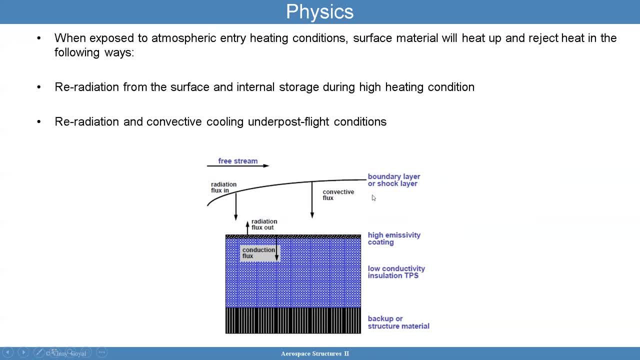 flow developing. you're going to have a boundary layer or shock layer. you're going to have a high emissivity coating. you want to emit a lot possible so you can have radiation out, and then you're going to have- you're going to have a low conductivity material here, which is in blue. 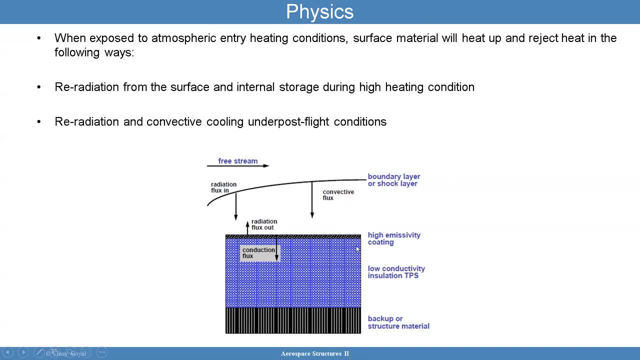 to help you so that the heating does not go through quickly because you want to keep up. you want to keep the backup structure as cold or as as safe as possible. if you have astronauts inside, i want them to keep them safe. so i don't want this backup structure to heat up, so i need to. 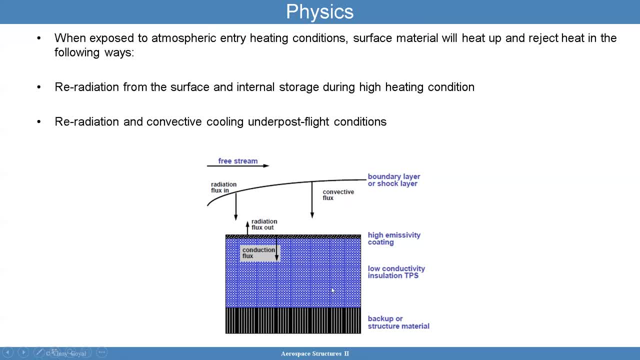 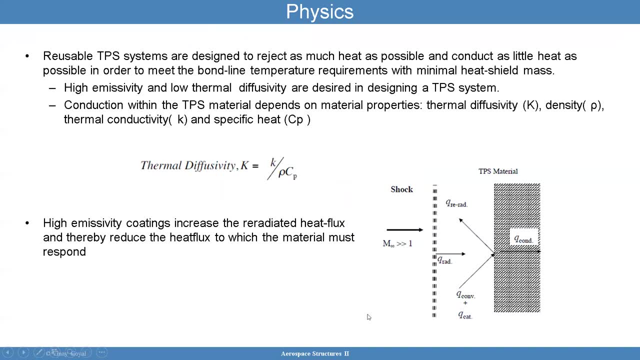 design this material such that it it doesn't heat up too quickly in the cabin area. right, reusable thermal protection systems are designed to reject as much heat as possible. right, and conduct as little heat as possible in order. so, right, that's what we talked about: we want to conduct as little heat as possible here. 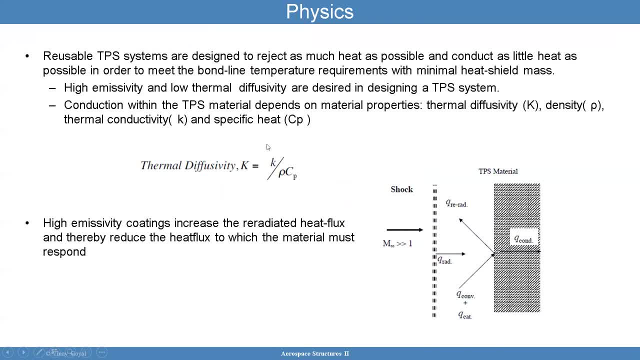 re-radiate as much as possible there and- and that's going to help us get where we need to go- the high emissivity and low thermal diffusivity are desired in designing a tps. conduction within tps materials depends on a lot of properties you have. thermal diffusivity comes into play. density. 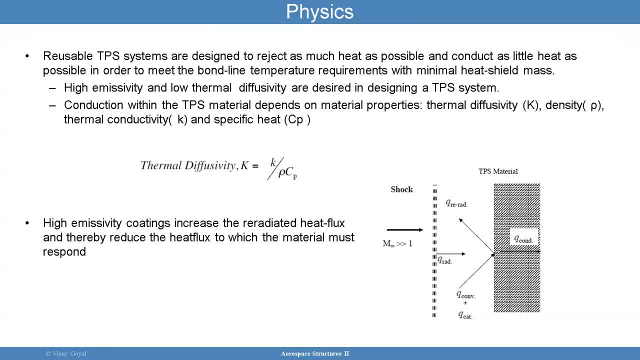 you have thermal conductivity and specific heat, if you're going to come up with a, with a formula that puts everything together. thermal diffusivity: if you put the conductivity material here, density here, in specific heat. this tells you how quickly the material will conduct like a, like a global quantity. it's very nice, very compact, high emissivity coatings increase. 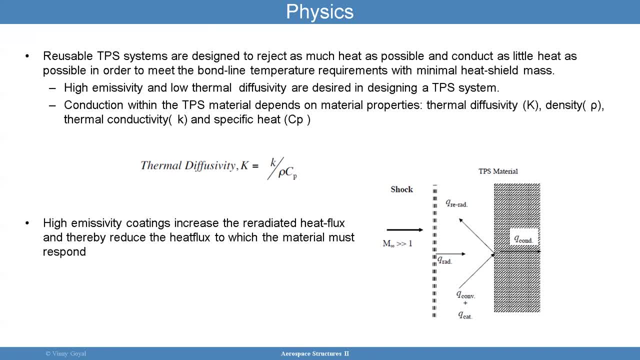 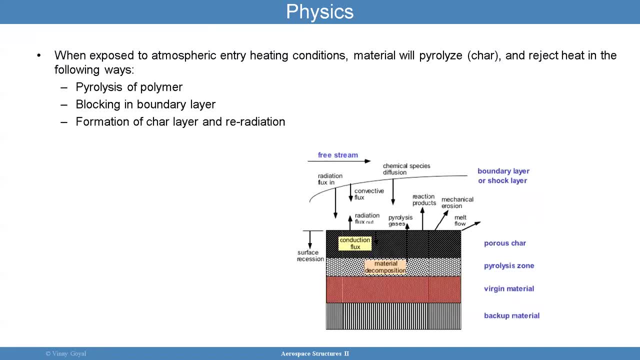 the re-radiated heat flux and decrease the amount of re-radiation radiation that goes into the material. so i want to explain some things that happen that are quite complex within this blue region for high heating applications. so in the case of atmospheric re-entry conditions, heating conditions, the material will paralyze it. 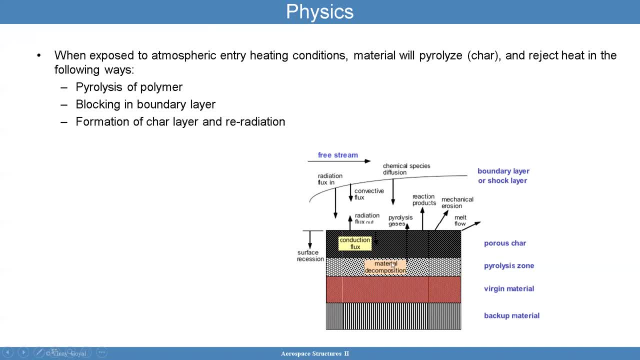 will charge. so this: you're going to have a lot of char here, you're going to lose some material potentially and you're going to reject heat by paralysis. paralysis blocking in the boundary layer and formation of the char layer and re-radiation. so what you see here is that the 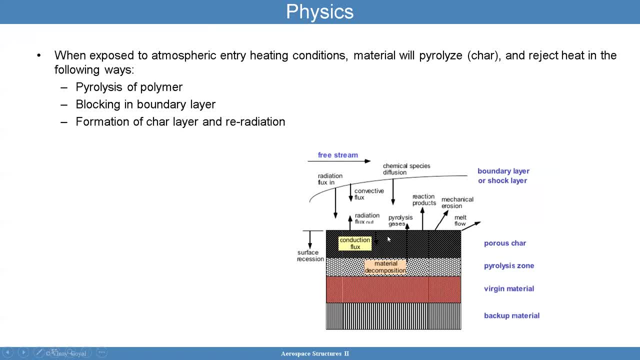 black here and, i pardon me, the black here has been, has been eliminated, has has basically ablated away. so you have mechanical erosion occurring from that and then you still have the material decomposition. this material beneath is decomposing. you have char here and then you have the material that has not experienced much yet. so we want to keep that as 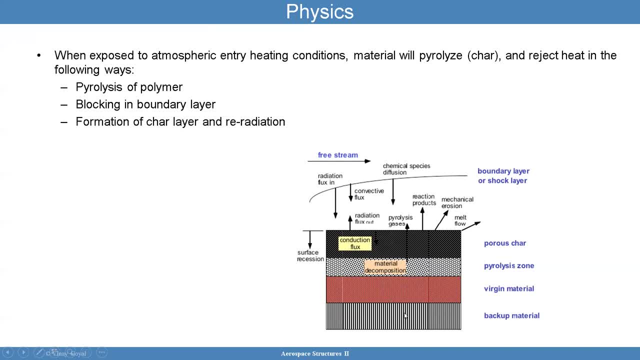 cool as possible, to keep the structural material as cool as possible for the cabin where the astronauts could be and or the payload or whatever you're looking at. but here is where all the action is happening again: ablation char, which is paralysis. there's a lot of activity going on here with gases getting. 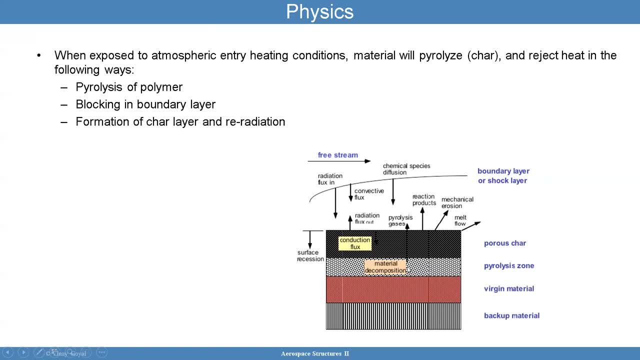 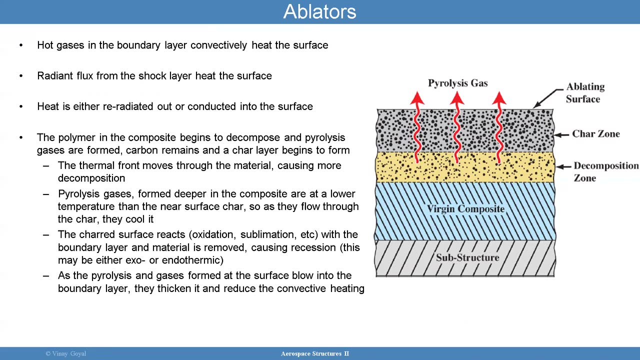 expelled. you can see here, when you heat up a structure at high temperatures you can expel gases, but particularly resin and yeah. so that's kind of what we're talking about here. very simple, and here i have a better picture if the previous picture was not helpful. 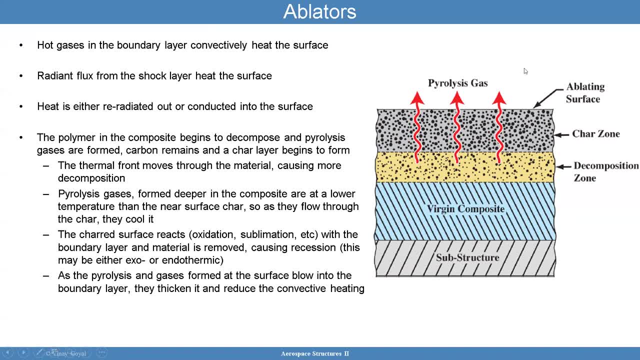 and uh yeah, you have the bleeding surface, the char, ablated already. i'm not sure what got ablated. you have the charge zone, the competition zone, the virgin composite and the polymer in the composite begins to decompose and paralyze and the carbon will remain within the charter which you know you're going to have some amount of. 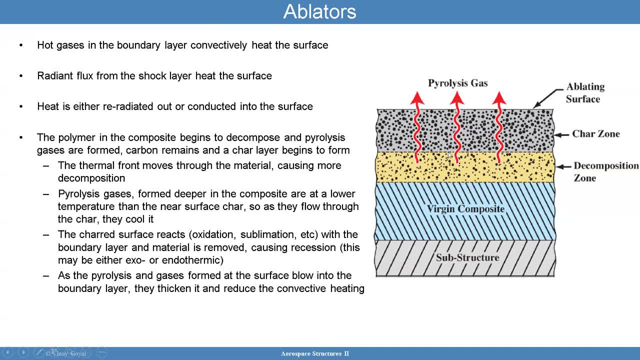 dark matter there, this thermal front. this thermal front is going to move through the material, causing this right here, this paralysis zone. the more you heat it up, the more it's going to move through the material down deeper and deeper right. so, as a mission, the space, the launch vehicle is taking off. 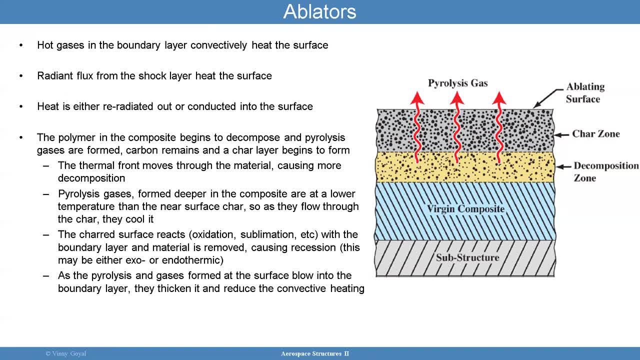 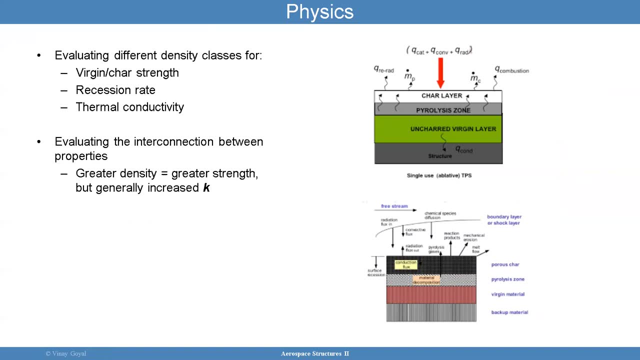 or the re-entry vehicle, like the space shuttle, for example, is re-entering, or you look at nozzle materials. this is going to keep moving down. what we want to make sure is to keep the structure cool. that's really what we want to do, and so the questions that typically looked at involve evaluating the questions typically. 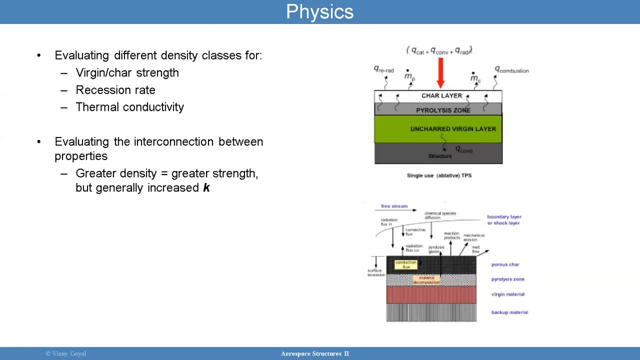 tackle the virgin, the char, the recession rates- you know how quickly we're receding, losing material thermal conductivity- and it evaluates the connectivity between properties. so it's going to look at how strength could be influenced by the connectivity, for example. but here are some of the variables that we start introducing, but you can see here the 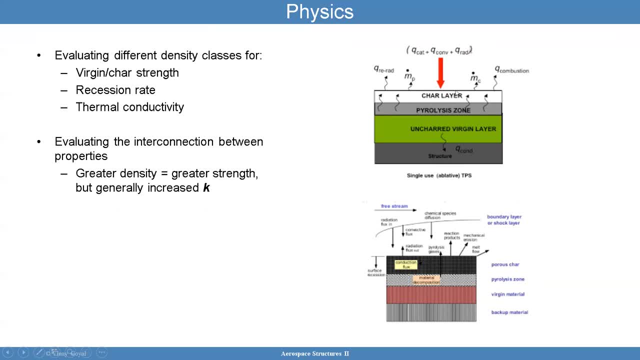 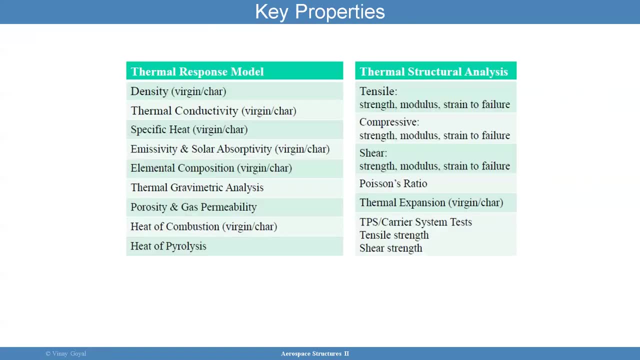 heat fluxes that are being considered mass losses at the surface and what we want to do is then look at the key properties needed to do an analysis this complex. that kind of analysis requires a good thermal response model. it requires a good thermal structural analysis model and is going to require 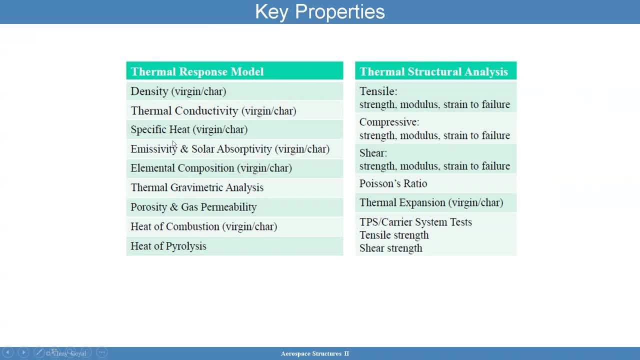 measuring density, thermal conductivity, specific heat emissivity and solar absorbivity. and you're going to do that for the virgin and char materials. you have the elemental composition, the virgin and char, you have the thermal gravity metric analysis and then you're going to have to also simulate the porosity and gas permeability. you also have 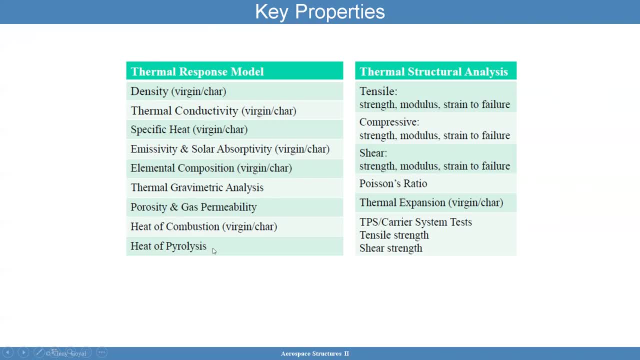 to have modeling that looks at heat of combustion and heat of paralysis from the thermal structure analysis standpoint. we're looking at strength modulus, strength of force, strength of force and ofагility throughout gas and understand what happened at both of these endings and when the kolatorrhythmos têm. 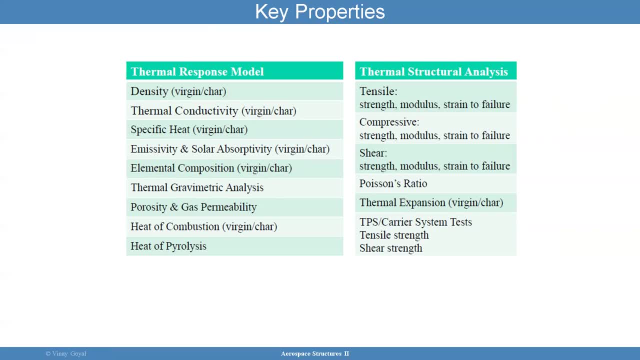 sporting properties, and thus we need to do these things or we're going to get to these today's key problems. you also have to find out how high we are, gas concentration and vacuuming the model, And so if the model is insufficient, we have a problem right If the model is using. 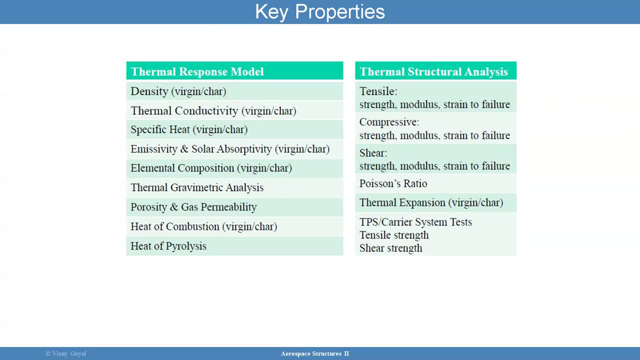 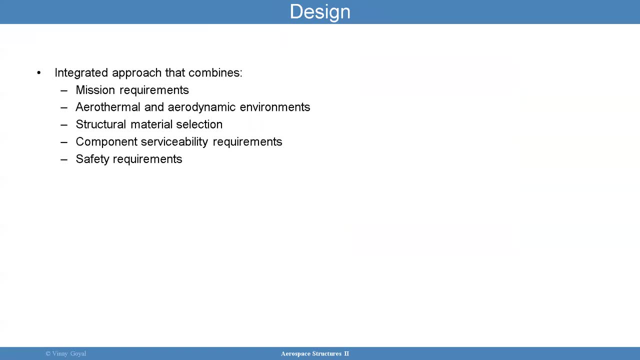 fake properties or assumed properties are not correct, we have a big problem, right, And so yeah, so that's what we got there: The design. So typically the design involves an integrated approach that combines mission requirements, the aerothermal and aerodynamics. 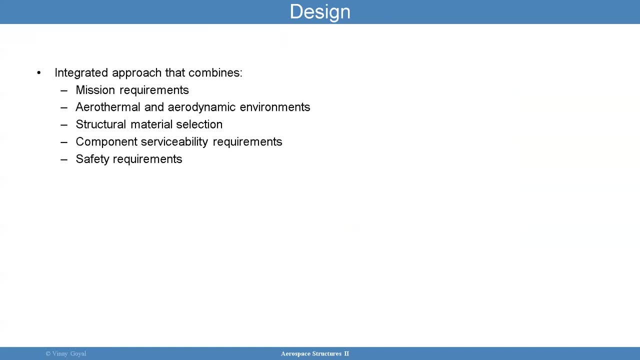 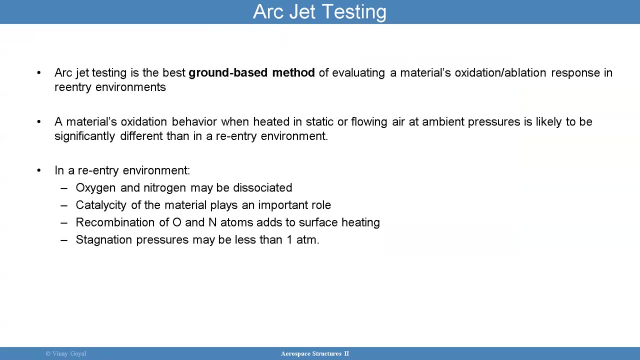 environments, a good selection of structural materials and the ability to service the components. Also, we want to make sure we have good safety requirements. So a good test that's done on the ground to test the materials at hand is called the arc jet testing. It's one of the best ground-based methods for evaluating the material. 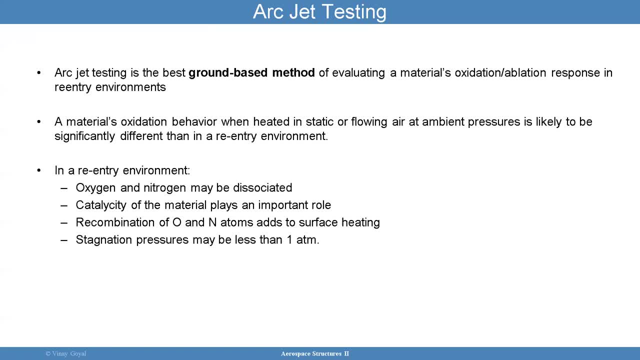 response, ablation and oxidation in a reentry environment. A material oxidation behavior involves a good selection of structural materials and the ability to service the components. A material oxidation behavior occurs when heated in static or flowing air, at ambient temperatures, pressures, and is likely to be significant during reentry environment. 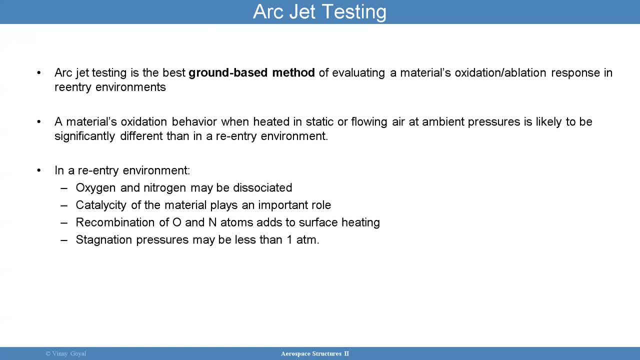 In a reentry environment you're going to have oxygen and nitrogen, which could be disassociated. Catalysity of the material also plays a role. A recombination of oxygen and nitrogen atoms can also occur at the surface that's been heated, And then you have the 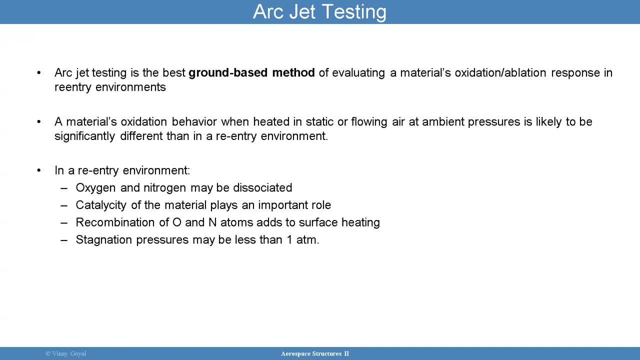 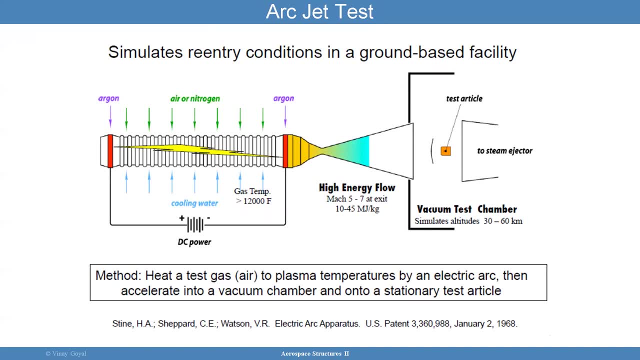 stagnation pressures that could be less than one atom. So those are the things to be considered. for that, The arc jet test is a very powerful approach. You can download the paper here. It's very old technology. You can study that, But you have argon gas being used, You have air and 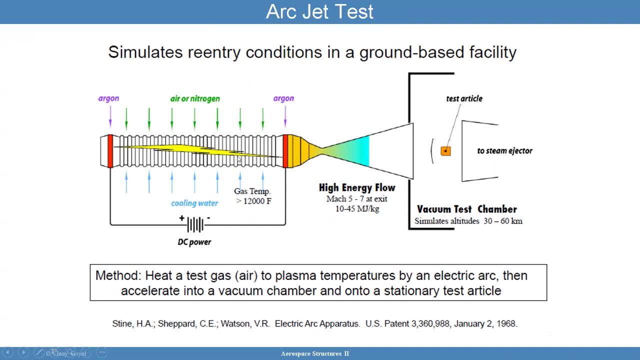 nitrogen, And you have gas temperatures up to 12,000 degrees F, with a DC power and a cooling tower water, because you don't want to Damage everything, And so this has a nozzle that expands And it's going to have high energy flow at Mach 5 or 7, with very high energy megajoules per kilograms being pointed. 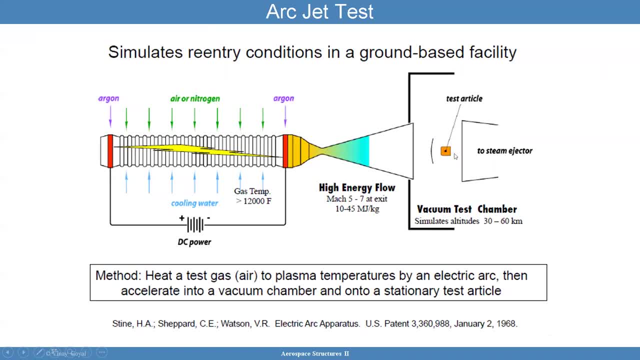 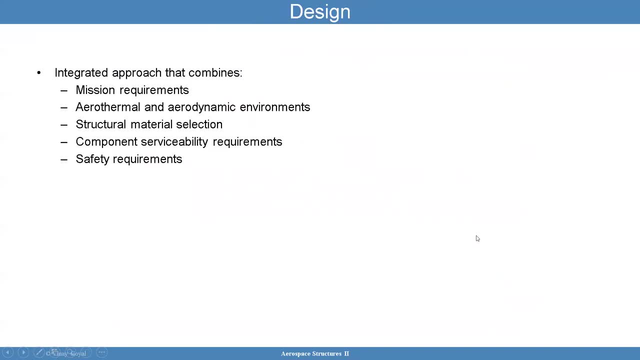 and directed at a test article. So this test article is your material that we're trying to study. So this kind of material And the idea is to look at the performance of that material, It can help you anchor analysis to test And it can help you look at the performance. 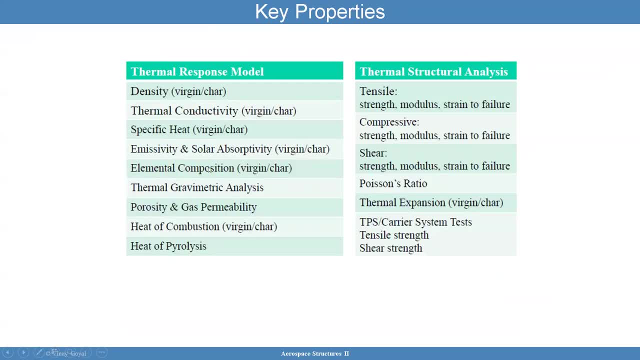 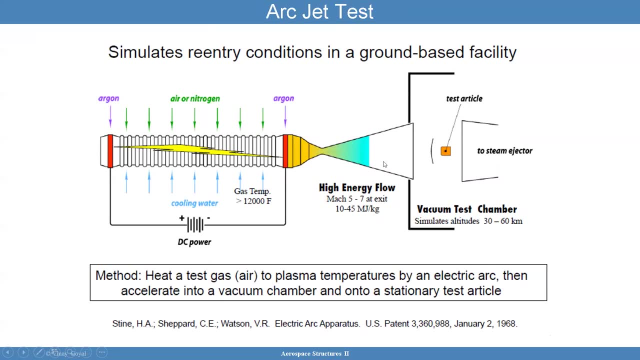 of that material And it can help you test to make sure analysis- that's using these thermal response models and thermostructural models- are accurate, because those models will then be used to analyze the flight trajectory you may have, And so that's an important aspect. 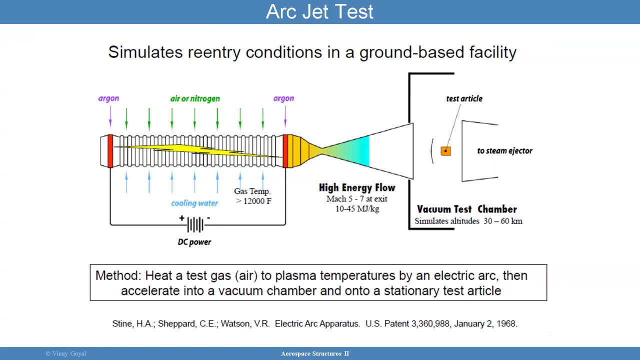 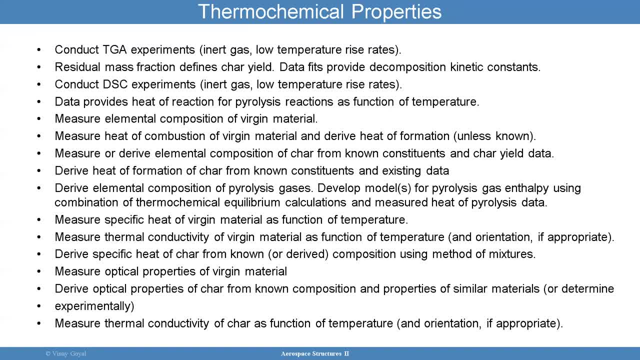 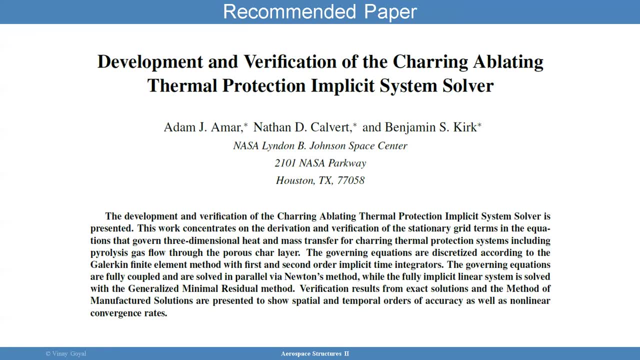 materials have a directional dependency. I apologize for rambling there for a second, but we want to look at measuring the conductivity in the different directions, because they're going to be different for composite. I really recommend reading this paper. It's called Development and Verification of the Charring and Blading Thermal Protection. 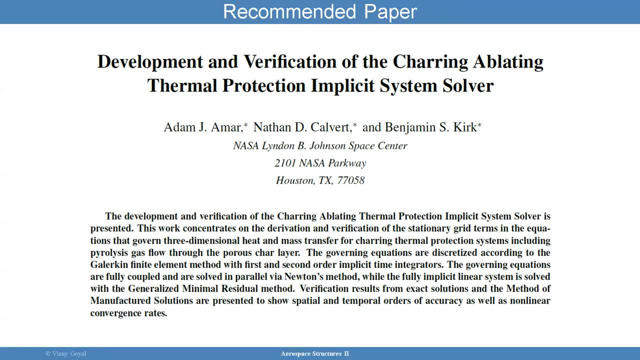 System, Implicit System, Solver, And I do think this paper goes into extensive derivations and verification of what they use for the equations for modeling the heat and mass transfer in 3D for charring thermal protection system, including how to model paralysis, And it uses very similar techniques we discussed today, which is using the weak form of the 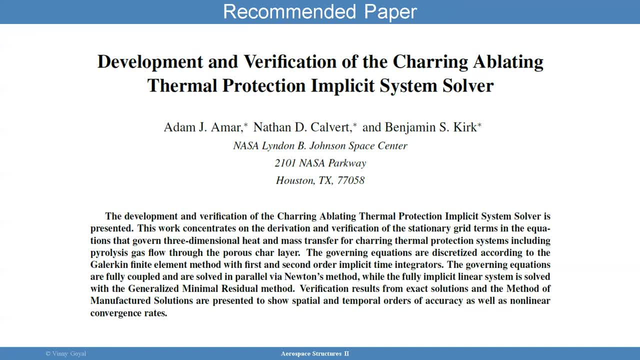 problem. I showed you how to do that. We start with the governing equations. We multiply by a function that's unknown, We make it orthogonal to that, We assume a, we assume an approximation over the domain which is polynomial, And then we discretize the PD, the partial differential equation, and we turn that problem into KU. 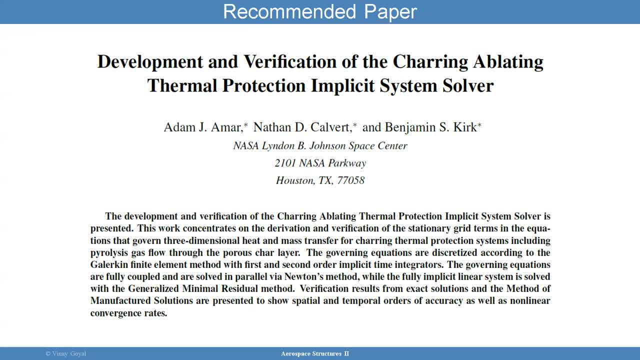 equals F, And we added a time dependent problem, which we need to for this kind of problem, And we can then solve it Basically. we can time march the solution moving forward or backward, And we can then solve it Basically: we can time march the solution moving forward. 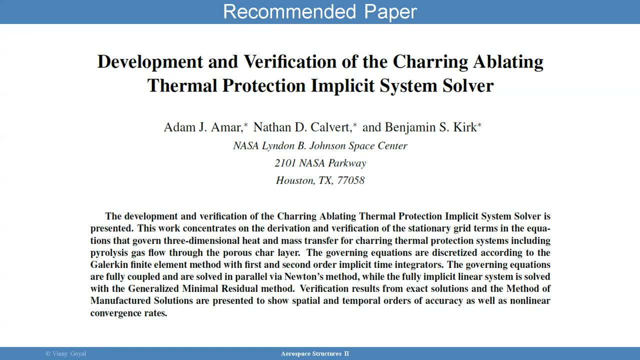 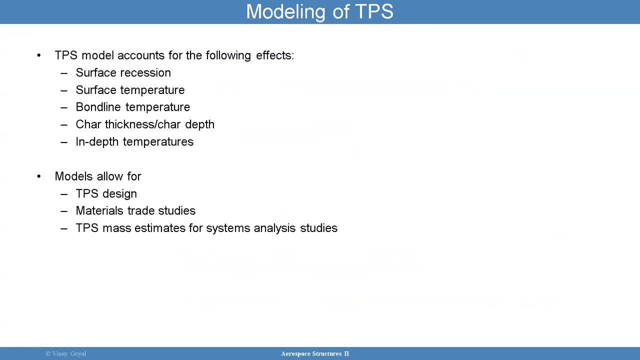 or backward, Because those two we had to do are having a backward difference. But you have to really look at the temporal and spatial behavior of the of the solution, Because these, these are very important when sizing a structure: insulation material, The TPS. 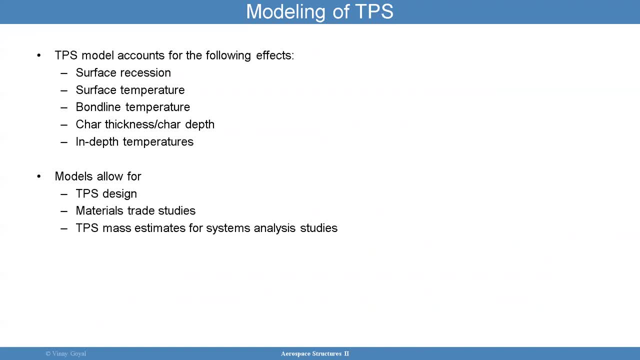 model has a couple of effects of surface recession, surface temperature, reunion temperature, char thickness and char depth in depth temperature And the models have to allow for TPS design, material stress studies, TPS background. So, in short, of measuring an insulation graph. we try to make efficient resolutions that are more cost effective and the comfort of entities which we charge: municipalities, environmental, Litre, thermal energy and tour And TPS models, materials, system stacked with service. Uh, and actually this says: featuresango R governs long features with thermal. 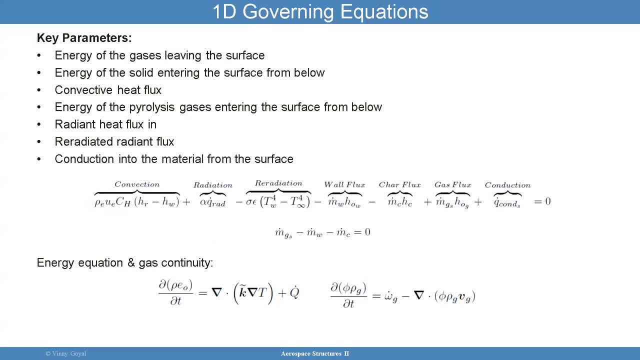 mass estimates for system analysis studies. Just to show you how complex it is, I'm showing the 1-D governing equation. This 1-D governing equation shows how you have to tackle the various aspects: the paralysis gases aspects, the convective heat transfer, the convection and so forth. 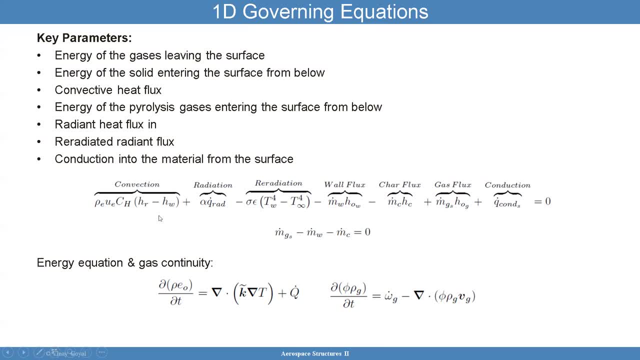 And I want to go through each term. So here is the convection term. It looks very similar to what we talked about before. You have the radiation term, which is going to account for radiative heating, So the hot gas itself can radiate heat into the material. 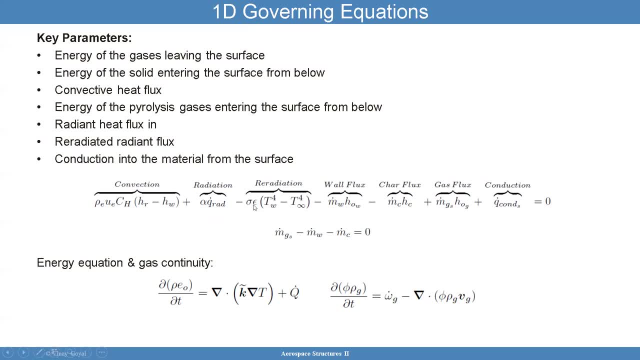 Then the re-radiation, which is going to have the Stefan Boltzmann coefficient here, epsilon, And then you have sigma here. So these are constants, And now you have this re-radiation term. Then you have the wall: mass flux at the wall. 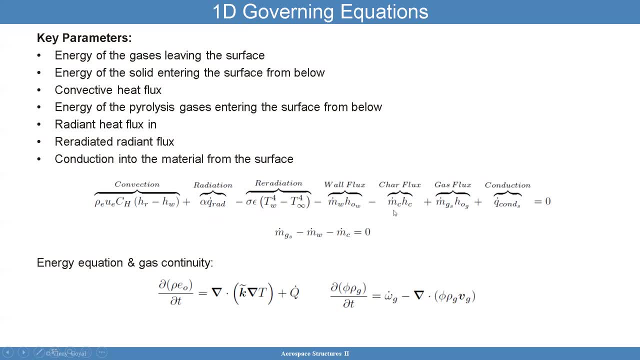 You're going to lose some mass. potentially You're going to have some char, some mass lost from char, You're going to have some gas flux And you have to have these three things in equilibrium. Mass has to be constant, So whatever is lost and anything in has to be constant or equal to zero. 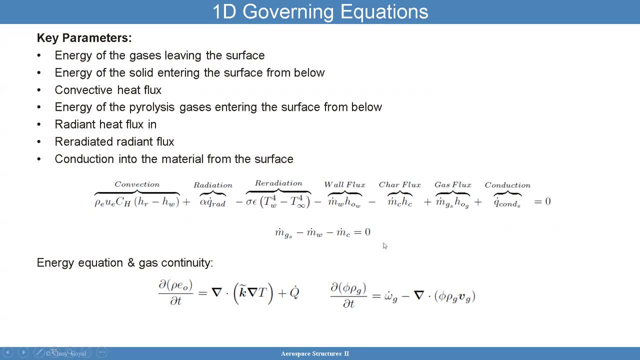 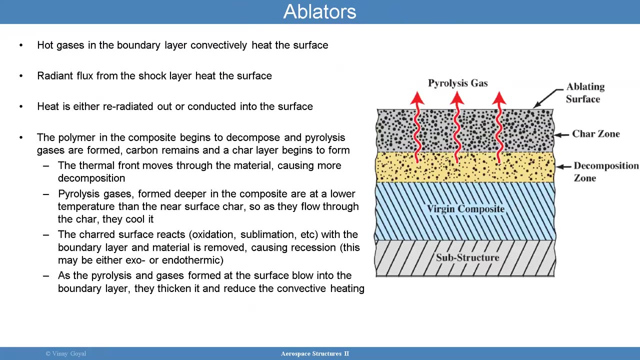 Then you have the conduction aspects. So all this has to be accounted in these equations. And then you have to add the energy equation and the gas continuity equation. Those three, four equations together for one, they need to be solved. So a lot of times these problems, which may be three-dimensional in nature sometimes, 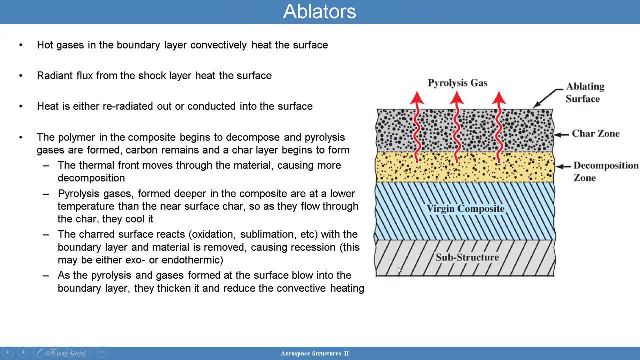 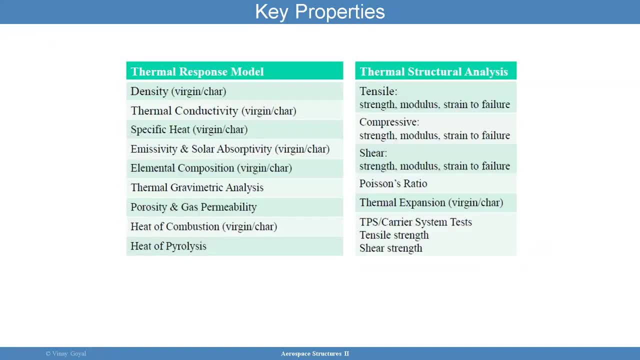 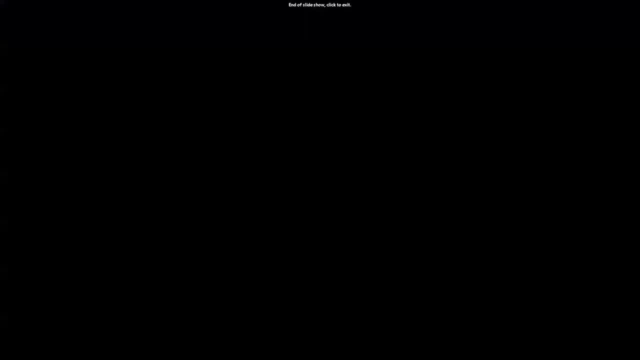 are solved in a one-dimensional manner to solve the problem, to basically accelerate solving the problem as much as you can. So, with that said, this gives a very top-level view of a thermal protection system problem. We'll be doing some of that in a project. 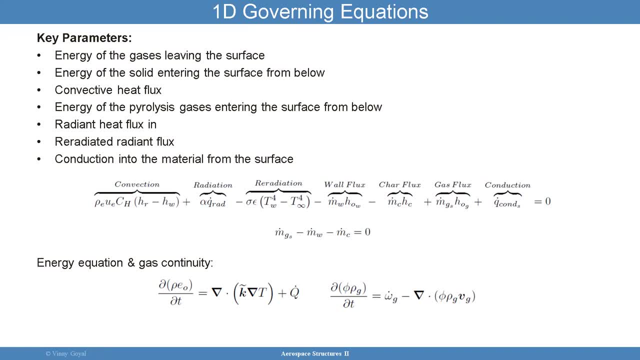 We'll be looking at how we can size the thickness. You'll be looking at that, But we're going to try to not focus on these other terms that can be quite complex, but maybe like a first-order estimate of what that would look like.